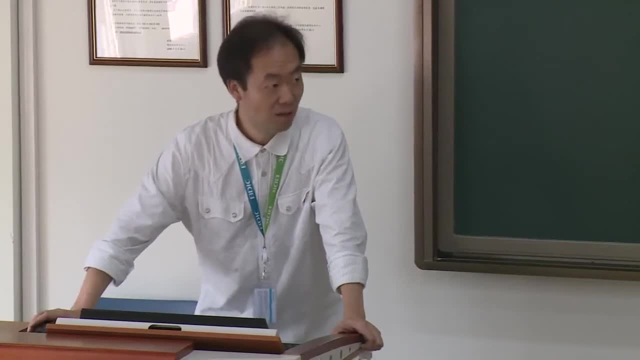 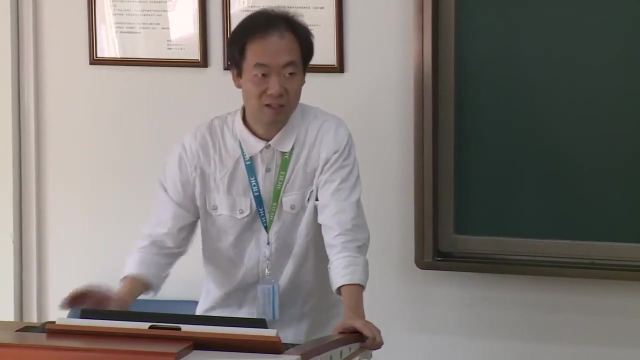 So it is our great pleasure to have him to give us a four-day lecture, A short course about topological fluid dynamics. Here we have a suggestion for the audience: Please just write something on your notebook, Because he will just give you handouts, maybe two days after giving the lecture. 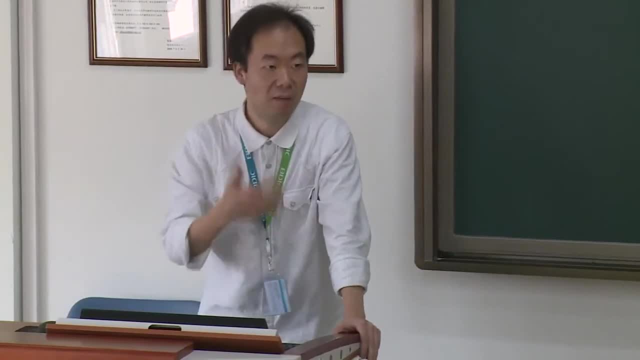 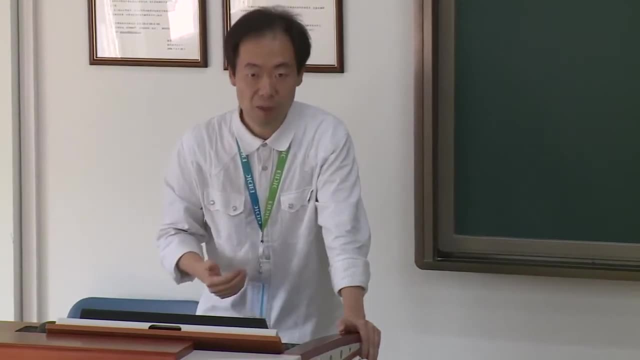 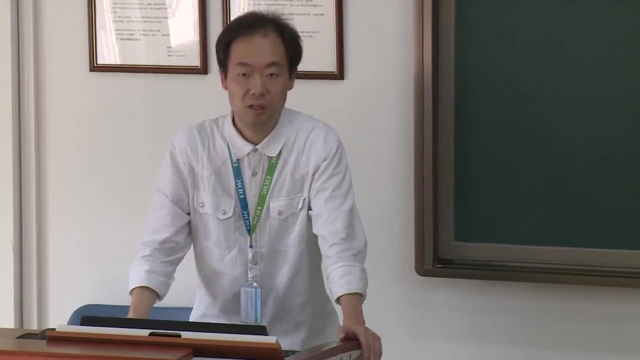 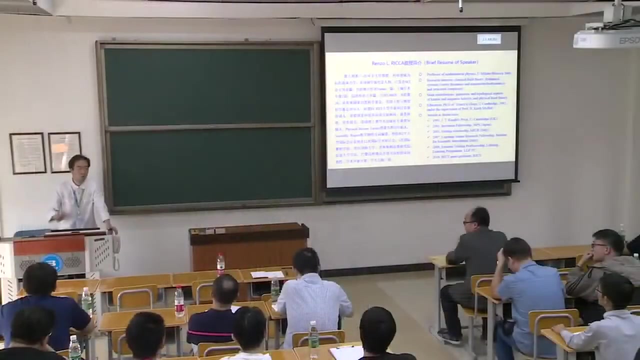 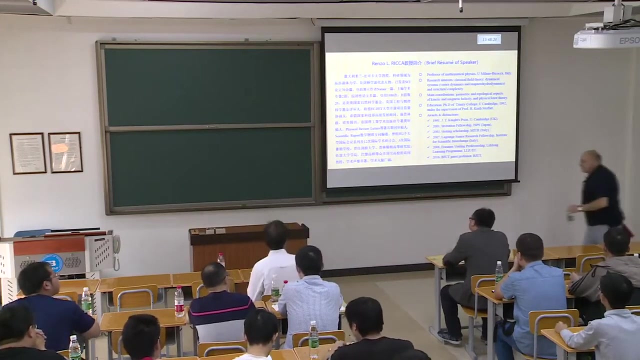 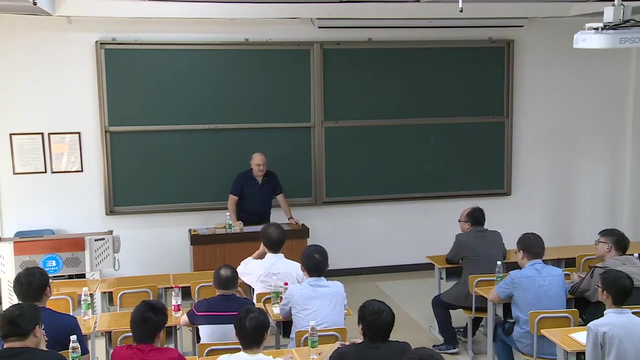 So Well, thank you very much. Thank you for the invitation, Of course, the Institute of Theoretical Physics in particular. 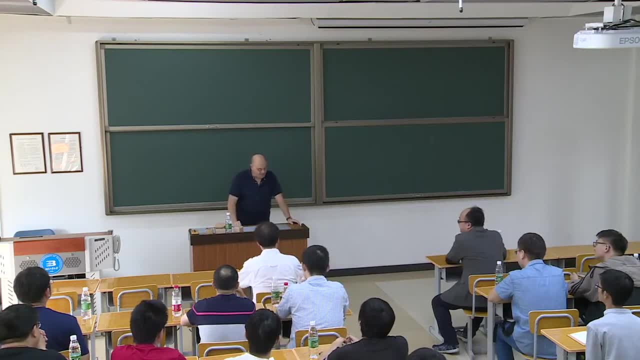 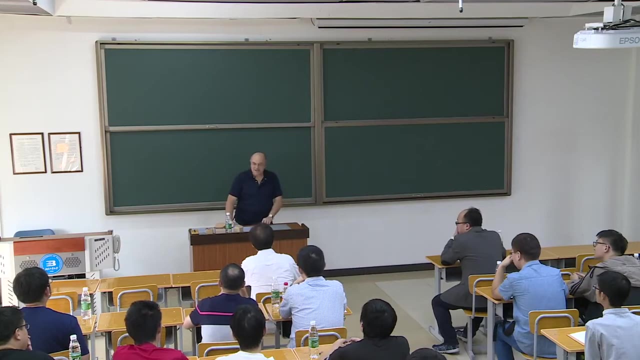 represented here, and Xin Liu, as part also of the Beijing-Dublin International College. I thank you very much because it's a great pleasure to be here and I know I've been always welcomed with heart and that makes me very happy. So thank you for being. 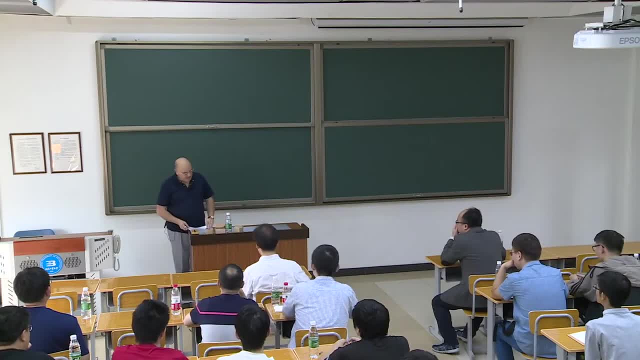 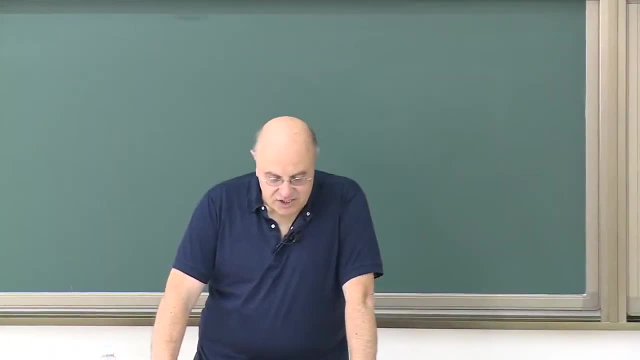 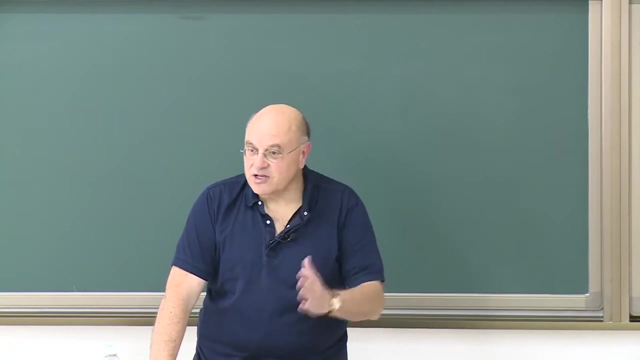 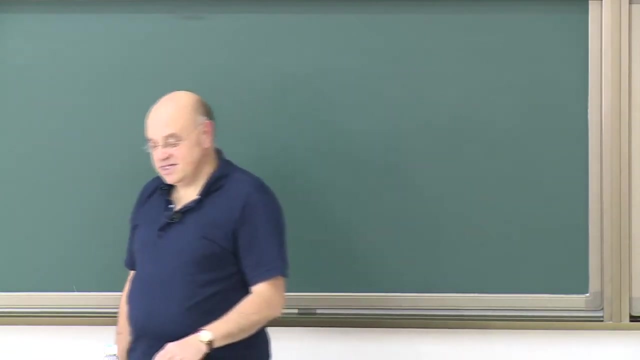 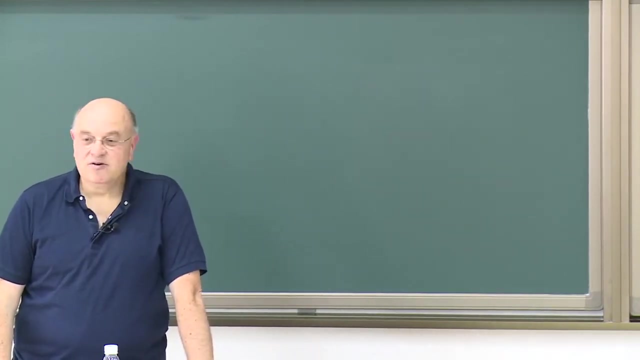 here. So these lectures will follow the kind of new revolution that we are living these days due to the great achievements and successes of recent approach of topological theory to physical sciences. You all know that this has had a great impact in string theory through the work of Ed. 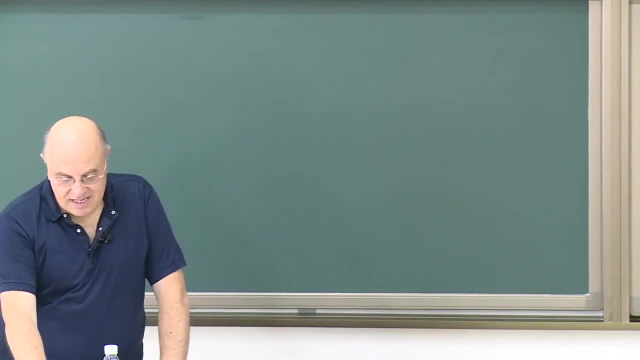 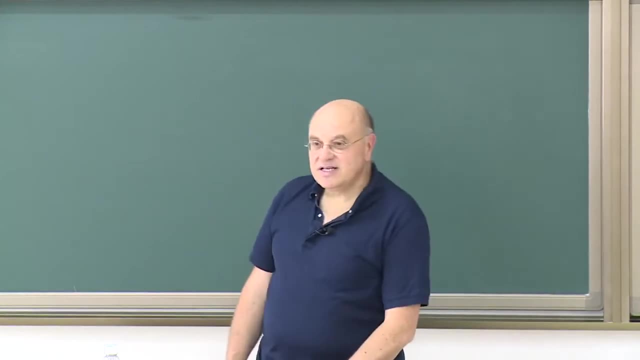 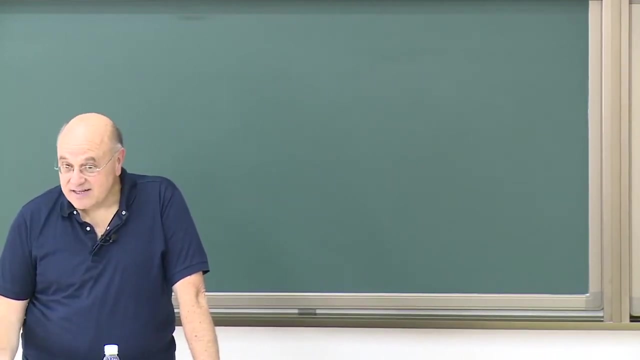 Whiten and others, and I am quite happy to tell you that this approach is actually much older. It is an approach rooted in the work of Kelvin in 1868, when he wanted to present, to produce a theory of everything, anteliteram. 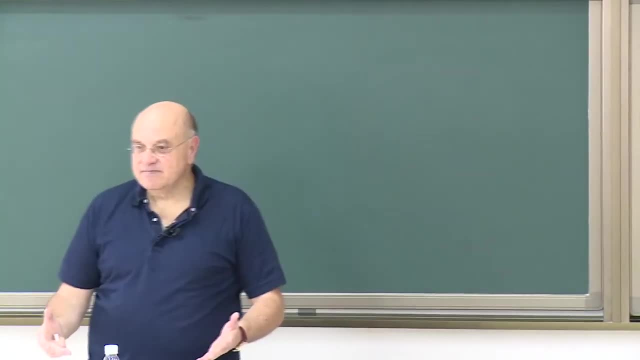 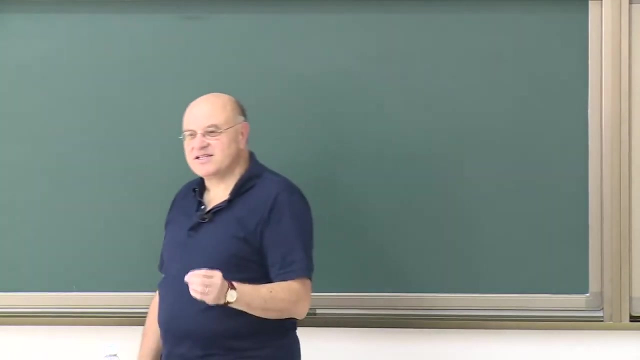 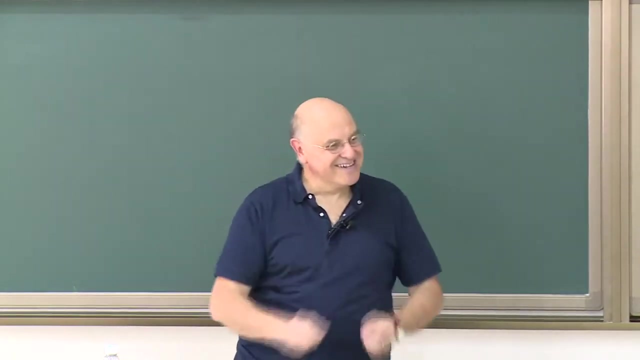 a theory of matter, exactly as we would call it now, a theory of fundamental physics. he conceived the idea that vortices were like infinitesimally small particles. we could paraphrase that saying: that is like a string in a fluid medium is like a fundamental. 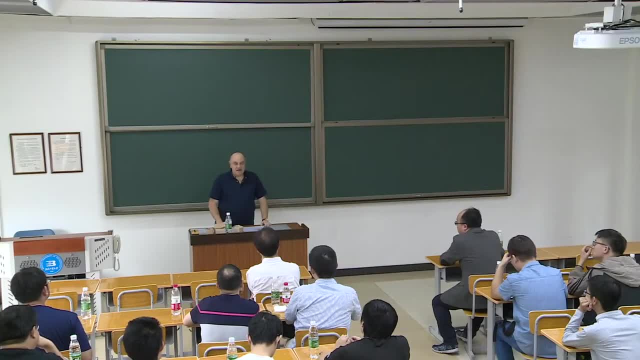 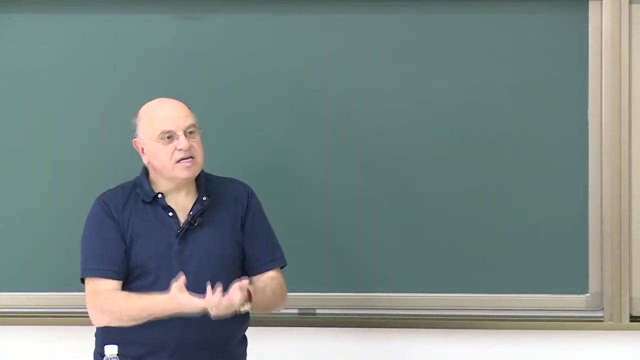 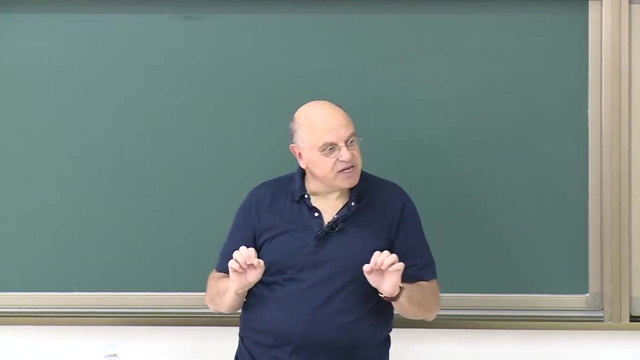 energy field at invisible scale and the idea is extraordinary. the idea 1860s. he had the idea that a vortex ring could link or not in space and because of the possibility of the permanence of ideal fluid, no dissipation, then topology had to be conserved. 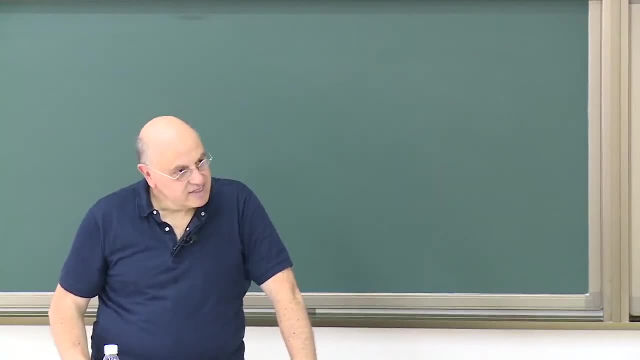 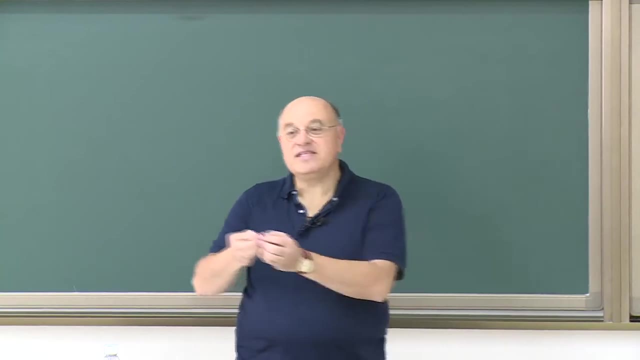 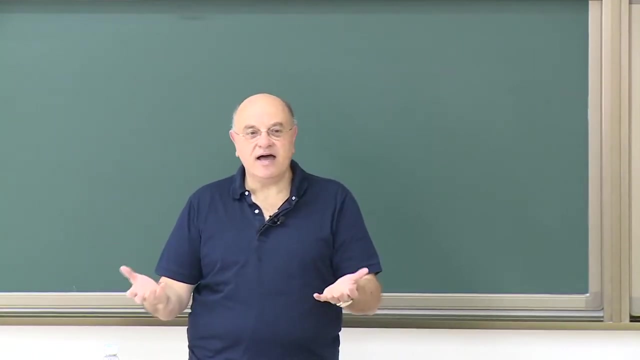 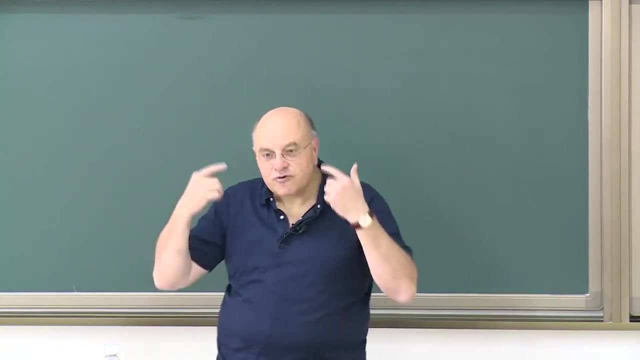 first thing. second thing, if topology is conserved, suppose you have a knot and you have a different type of knot of different complexity. then the two knots had to have a discrete amount of fluid and the two knots of different energy. so through this idea he envisaged: 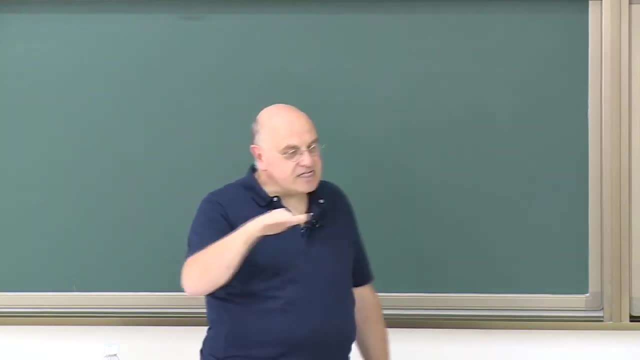 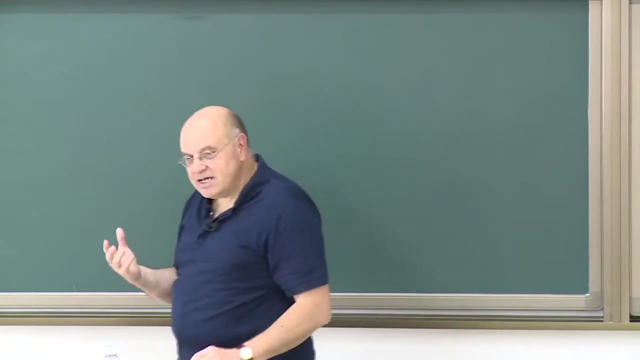 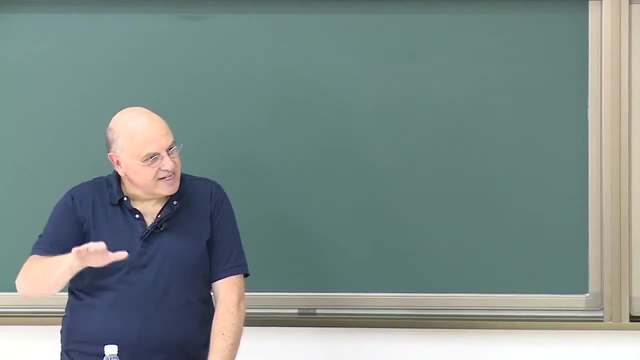 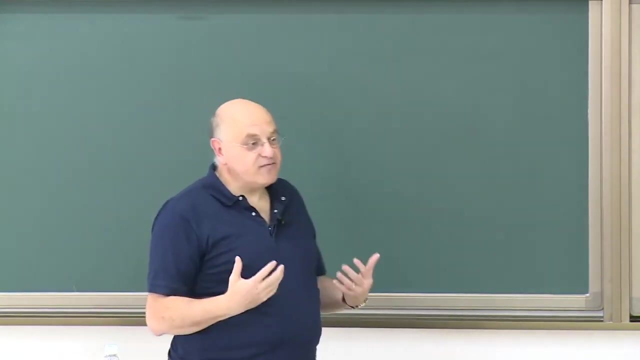 the possibility to interpret discretization of energy through topology. this is an incredible idea 1860s, because he not only understood that through that thinking was possible to determine a spectrum of fundamental energy states, but he could also envisage the possibility that these states were independent from the metric. 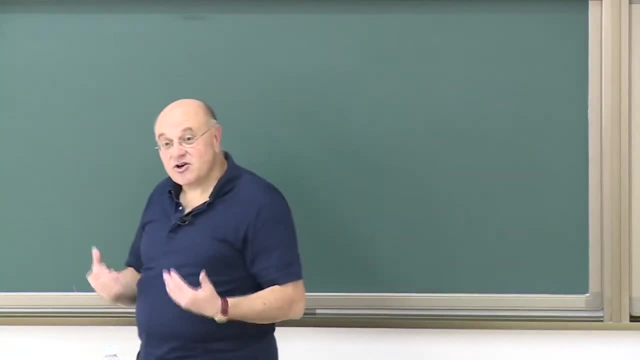 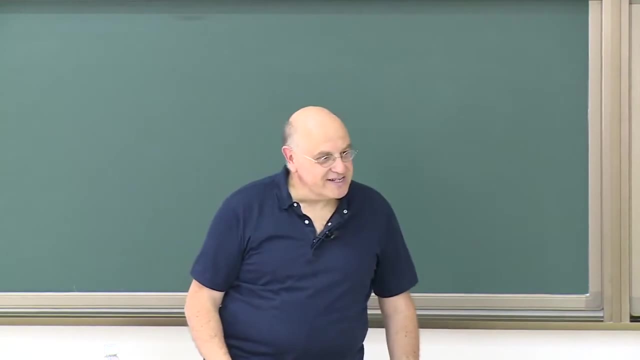 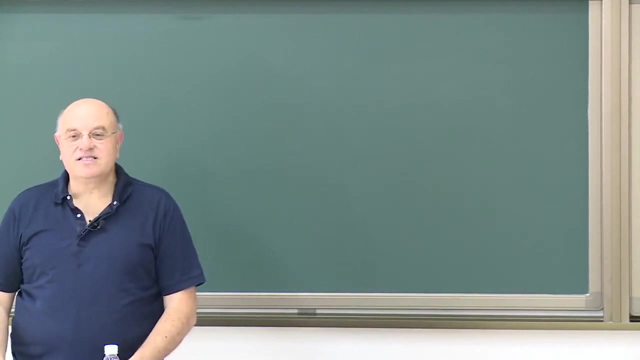 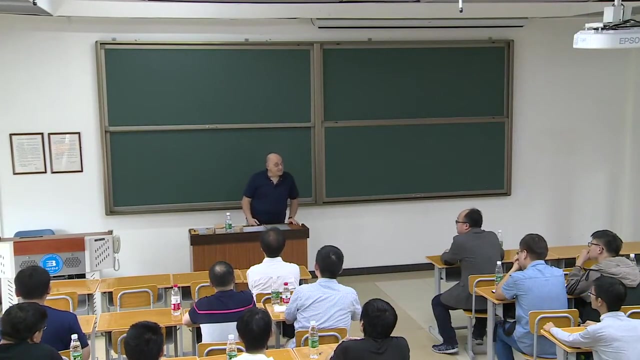 you see so many ideas already there that we now attribute maybe to modern scientists. ok, so we all know that this theory didn't survive in the 18. he had a number of outstanding followers, including JJ Thompson. JJ Thompson was an absolute brilliant mathematician. 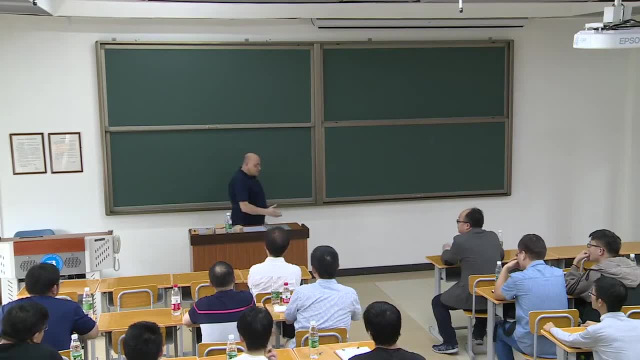 in Trinity and he worked on mathematical aspects of this vortex- atom theory. 20 years later, 1880, and the more he was working and the more things came uneasy and finally he dropped the theory to become a physicist and in 1906 he got the Nobel Prize. 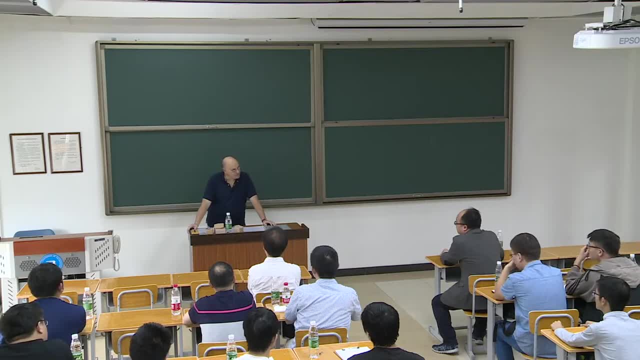 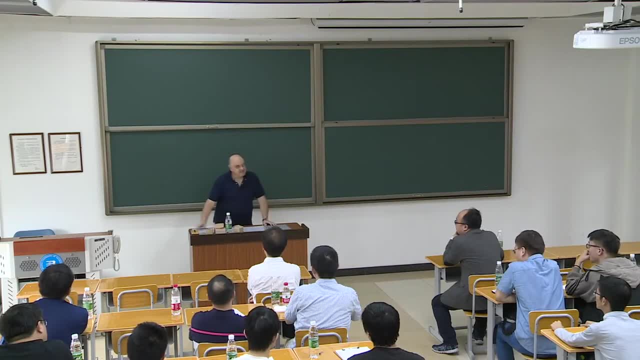 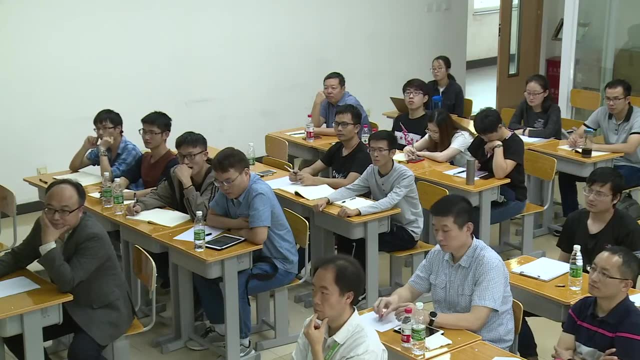 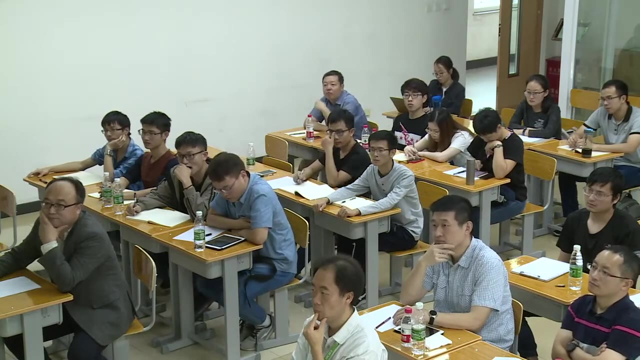 and he was the first to do so- the vortex atom theory. So this is very briefly the story about the topological fluid mechanics. that has gone shadowed, has gone down after that period because of the great successes of physics and the other interests in fluid mechanics. 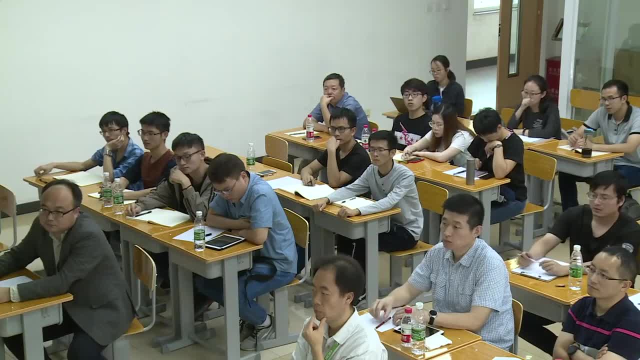 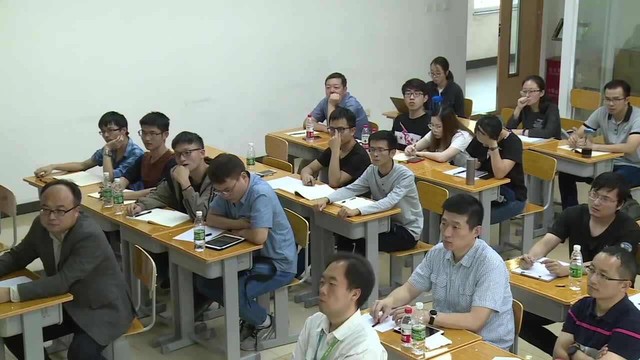 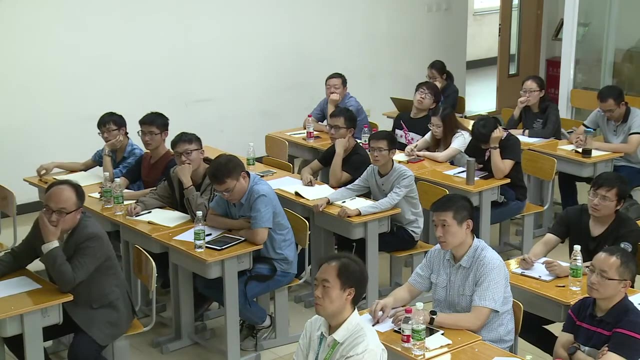 aeronautics, etc. etc. etc. But we inherit from that time this approach, The approach that through field theory, as we say now, we can investigate fundamental aspects, if not of the fundamental nature, but at least of nature. So I'm going to present 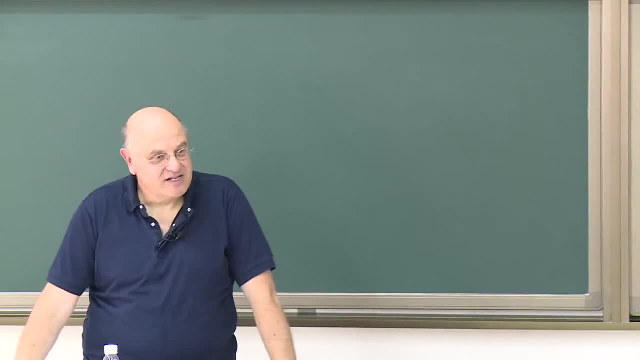 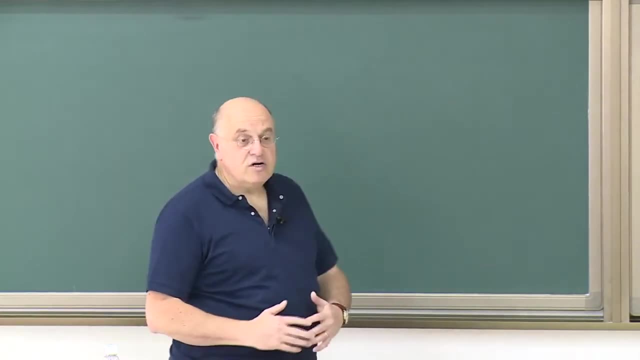 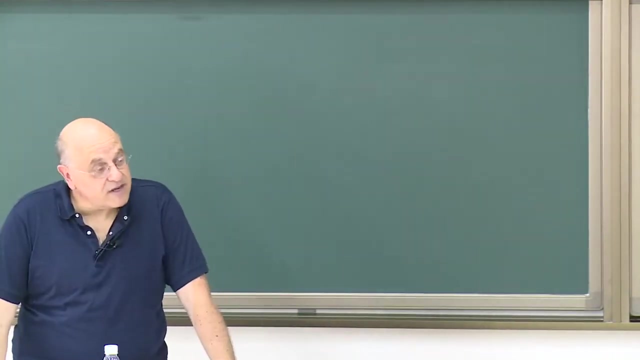 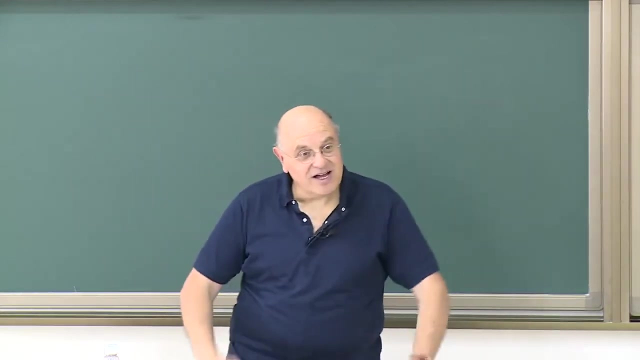 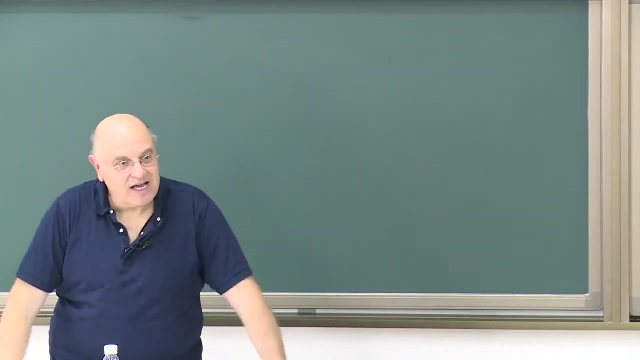 you just the introduction to this field that is now very rich. These years, in the last 20 years, we saw very exciting new discoveries coming from very, very talented young mathematicians and physicists, And so this field that survived through periods of ups and downs is now resurrecting. 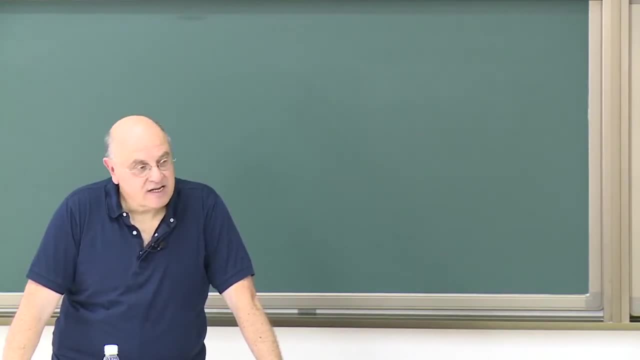 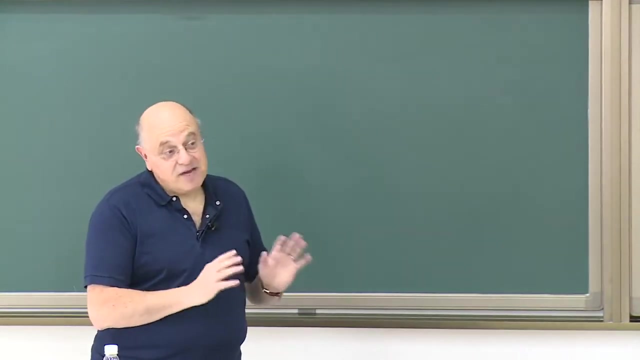 and has great impetus. Now I will draw your attention to a number of facts that are also relevant for mathematical problems, and I apologize if I will focus on mathematical aspects that are interesting for physical problems but are more mathematical in character. So 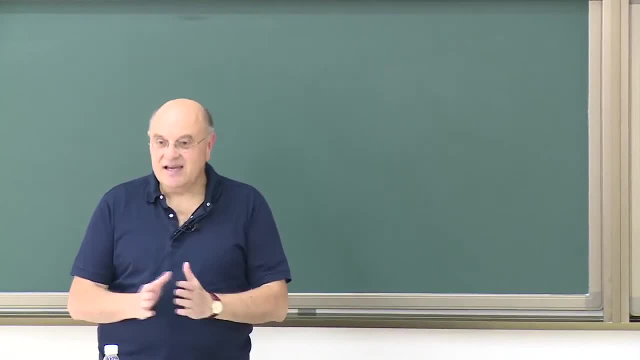 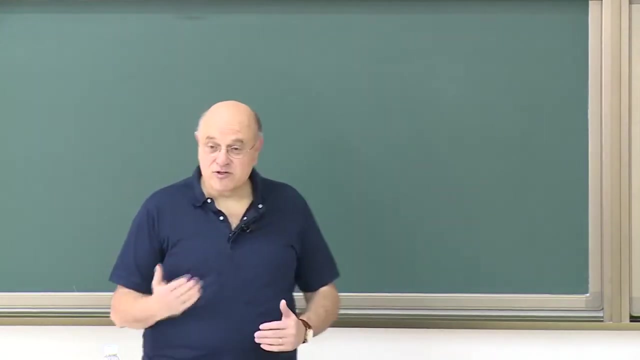 forgive me for this Being a short course. I need, however, some background material, so I am obliged to start from scratch in order that everybody is happy with what we are going to do. and then paste will increase after the second day, so from tomorrow. 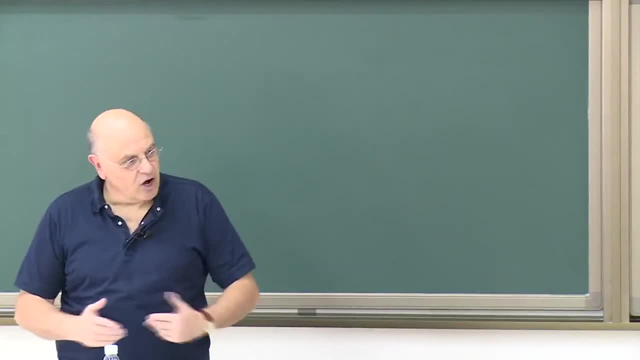 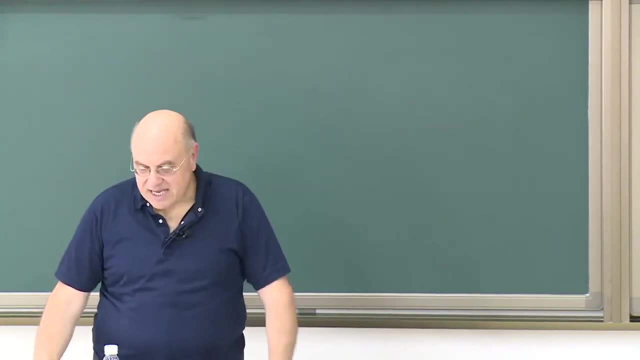 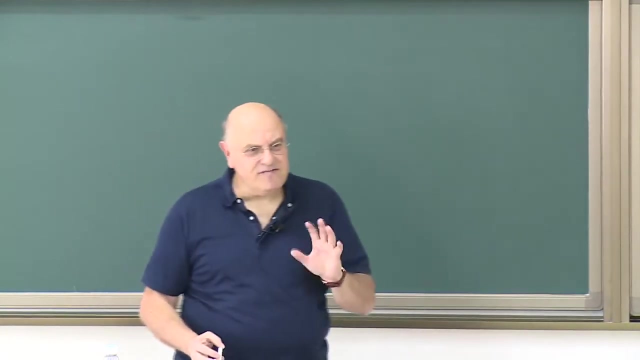 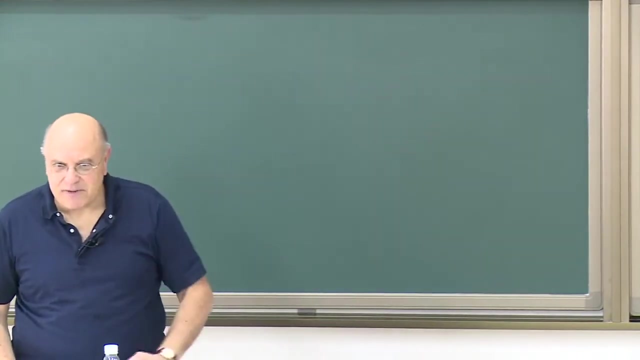 onward. we go a bit faster on more recent results. so forgive me if I start from really the beginning, and the beginning is a material that you find in standard books but has been revised, so I'm not going to present really the standard way of some of these topics I will try to present you. 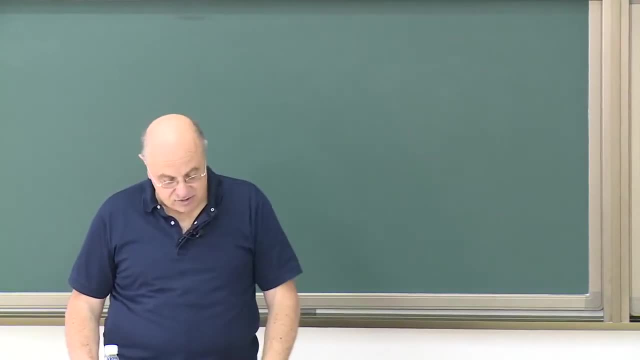 emphasis on aspects that are relevant later on. so I'm preparing notes, lecture notes, for you. so I still, uh, have to prepare my last lecture and I want you to have all the set ready, and since the set starts with an index, the index is not ready yet, and so please wait for a few more days. 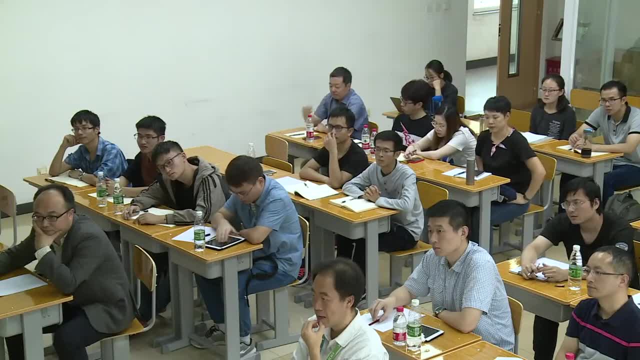 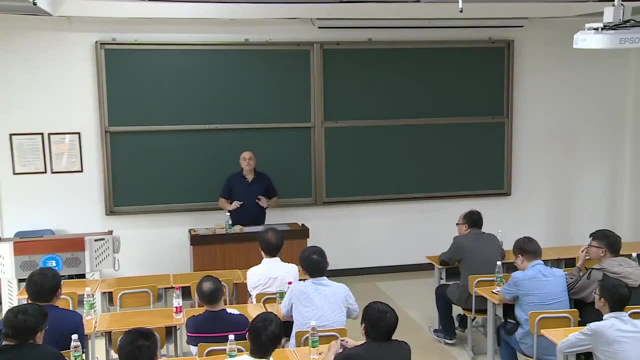 and you will have all the lecture notes. now. the lecture notes contain full proofs of what I'm going to mention, so there'll be much more material than what I can present to you. I will skip some proofs, I will dual on some proofs, but in the notes you will have a much deeper 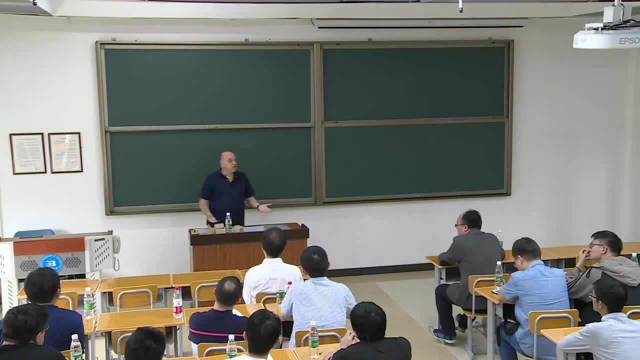 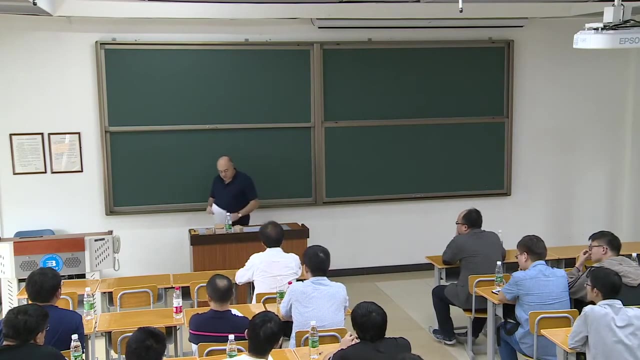 presentation. so also historically, I told you what I wanted to say. there is a little bit more in the notes. I will skip some basic definitions, but I want, I want to dual on some proofs, so I'm going to. I want to give at much more detail. I mean a development perspective, at least if you know what you're. 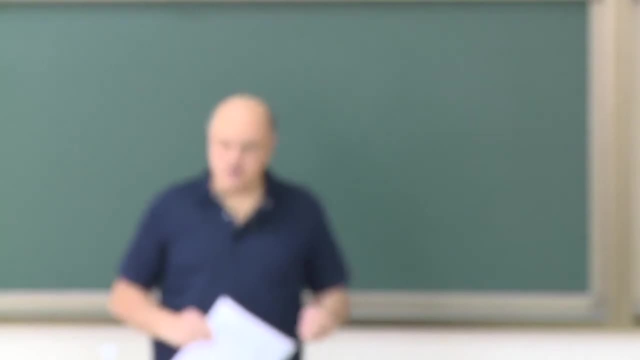 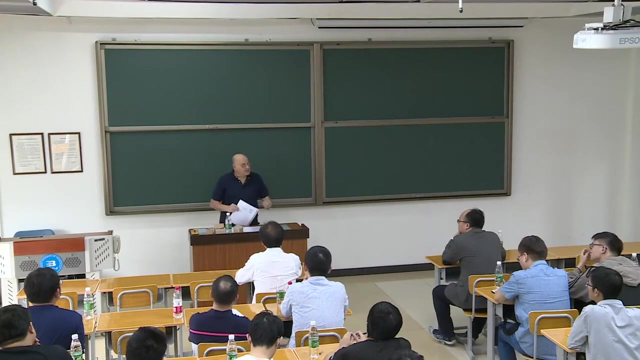 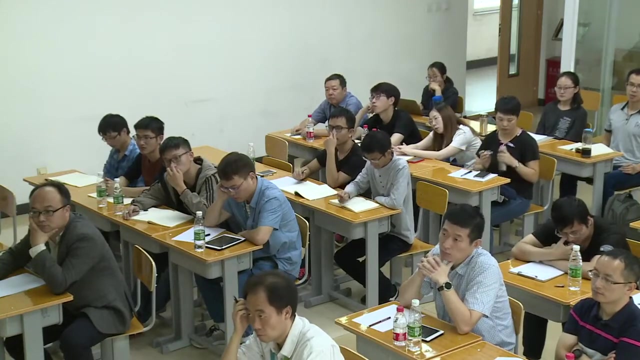 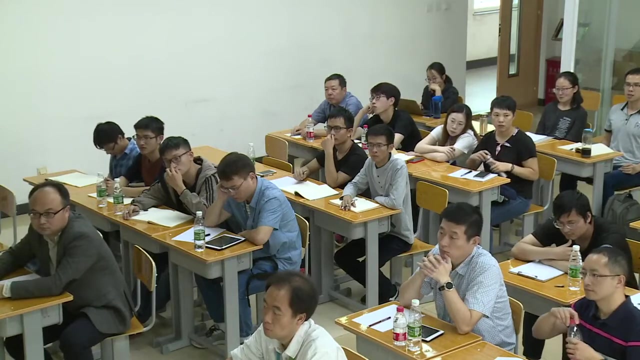 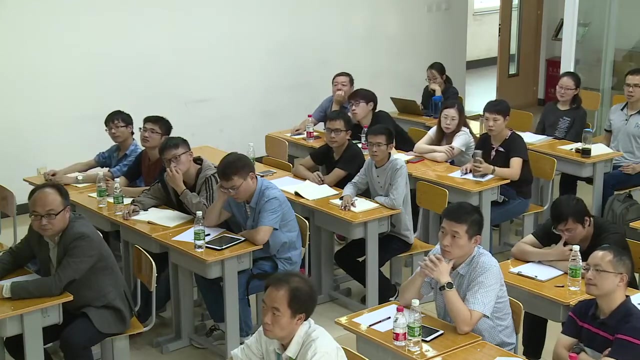 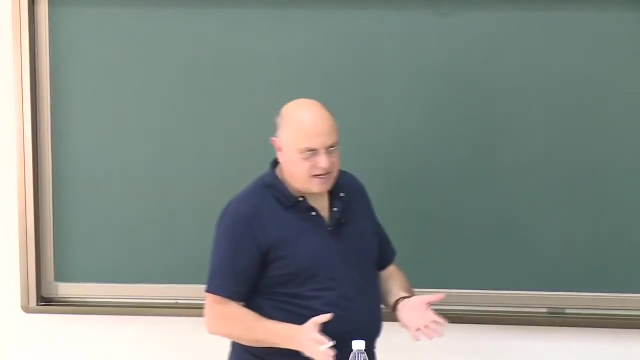 thinking. if you're working on some theoretical Inspector method, for example, make your. your are stimulating our imagination. So suppose we have. I will be extremely unprecise at the moment, just to give you an idea of what we want to tackle. One problem is: 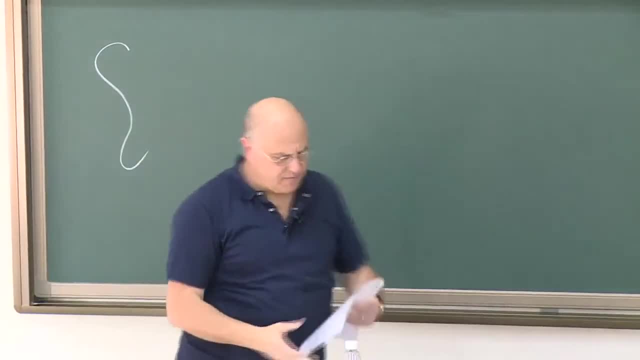 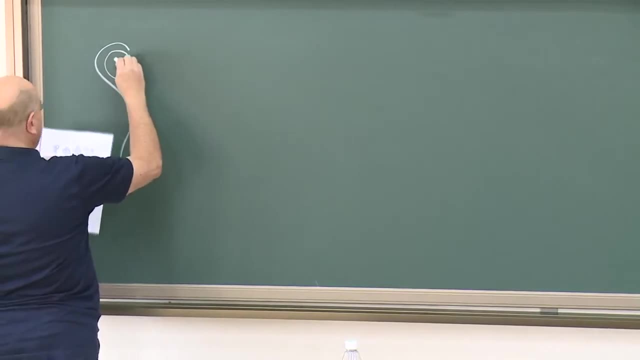 for instance, something like this: I have to look at my pictures because I don't draw things very nicely sometimes- And we have something like this, And these get linked with this part, And it goes back like this: Okay, Suppose you have. 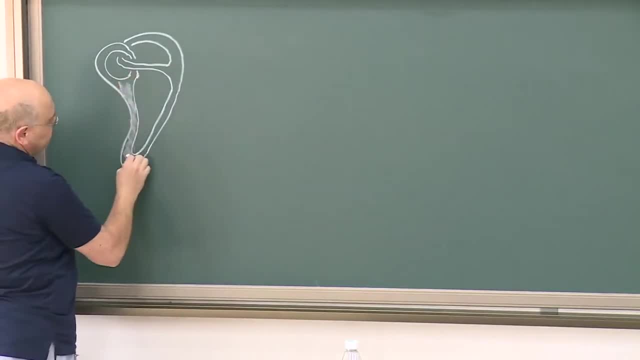 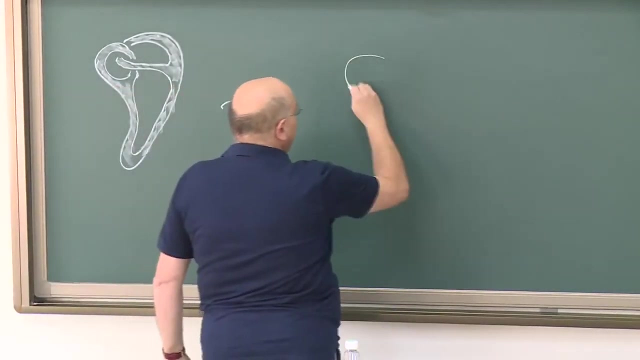 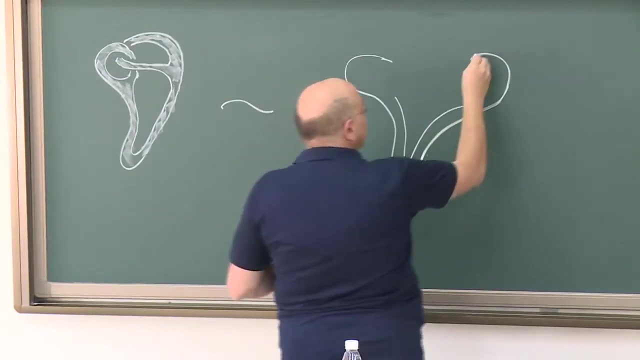 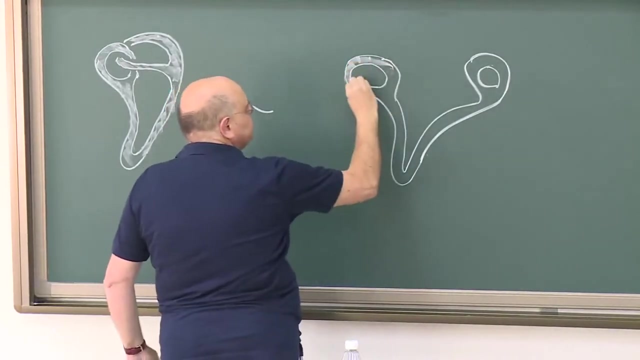 something like this, And imagine that this is made of some material, Maybe plastiline. Okay, You can deform it. And you want to play with this material by deformation, Continuous deformation, And you want to reduce this material to this material- Okay, 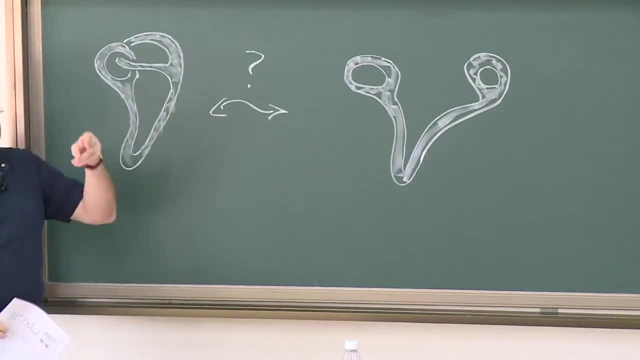 Can you do this without any cuts? No, You think No, Right? So the answer is that you can. You can. by continuous deformation of this material- imagine it's plastiline- you can deform this to this. So this is a challenge, right? 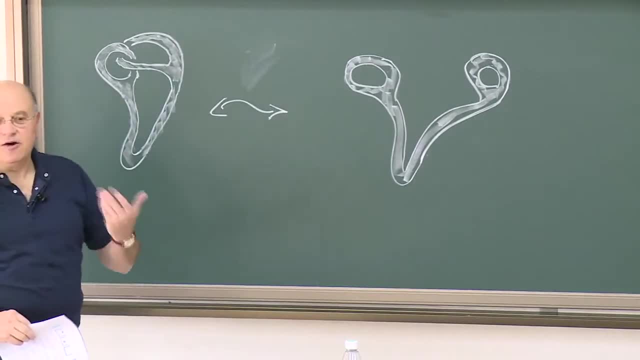 It's a challenge because it defies our imagination. We believe it's not possible, But it is possible. You can deform continuously, without cuts, this structure to that structure. And well, one way to do it is to you know you can deform this. 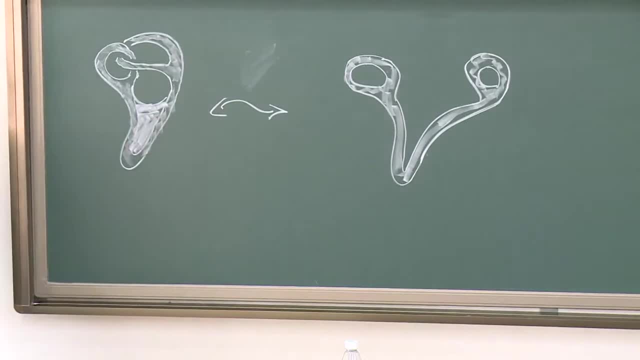 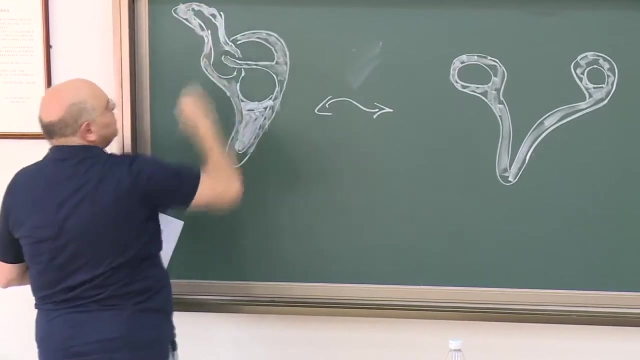 to make it very thick, Very thick, Okay, And then, well, we can use this to enlarge it a lot. You know, we can make it very, very, very large, Very, very large Through here and here. Yeah, 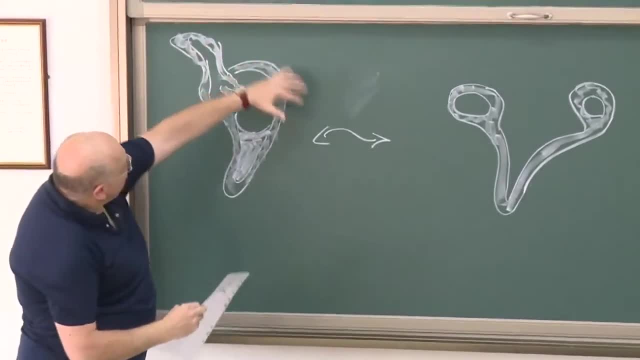 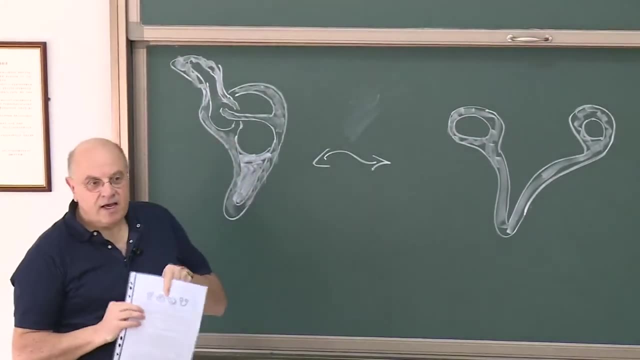 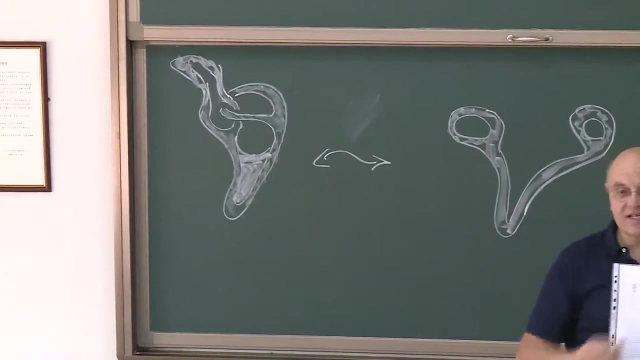 And then we can go this side all around the other and reduce this to this shape. I have a sequence here, much better drawn than what I did, And I'm sorry you cannot see it, But it will be in the notes, So I prefer not to waste time. 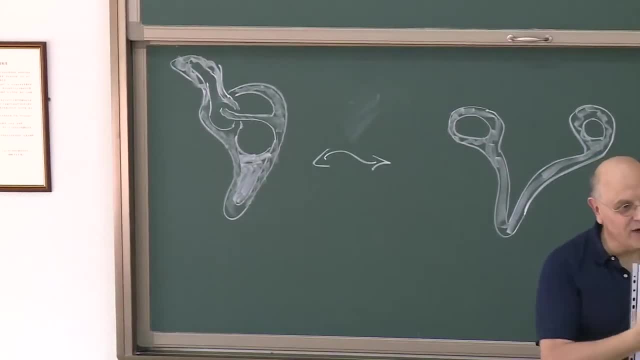 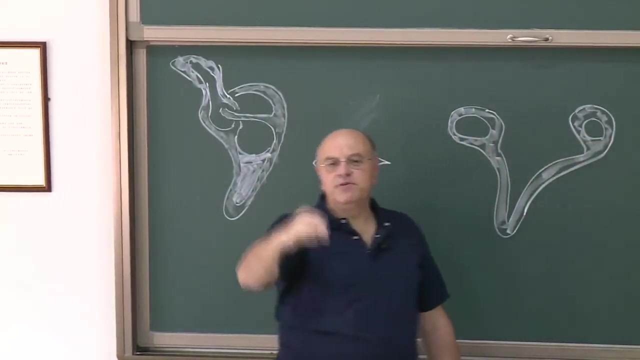 to leave you the curiosity to have a look at the drawing And, step by step, how to deform this to that. Well, there is another situation: Continuous deformation. There is another situation where we may start with fluid and we may put some light fluid on top. 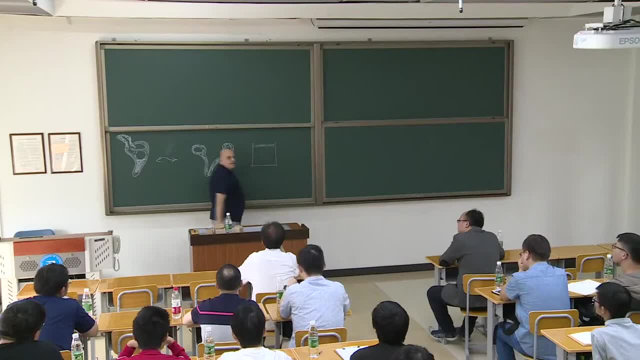 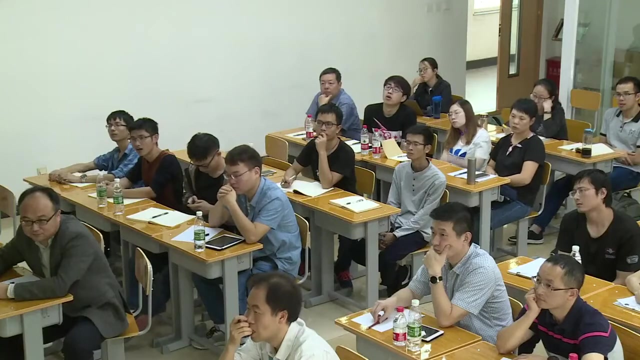 So suppose this is light fluid that stays on a heavier fluid. If we reverse the situation, this is stable, right, Because gravity is a pool of gravity working downwards. And imagine now that this part of the fluid is made by a heavier fluid And for some, 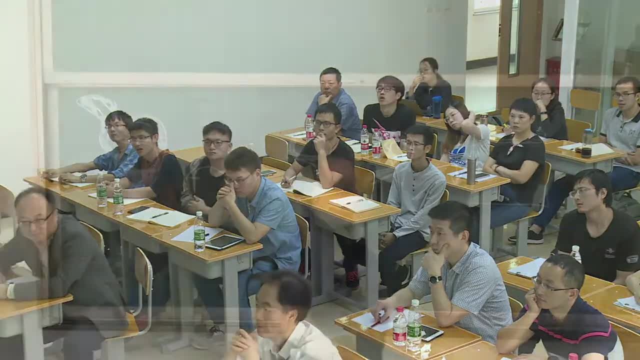 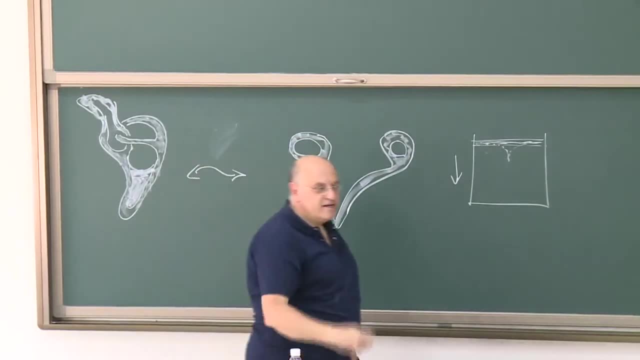 simple reason for simplicity, we assume that at a certain point this collapses. Okay, We know this. Oil and water, or vinegar and oil, etc. etc. We know that the two liquids, oil and vinegar, are hardly miscible If we want to mix them. 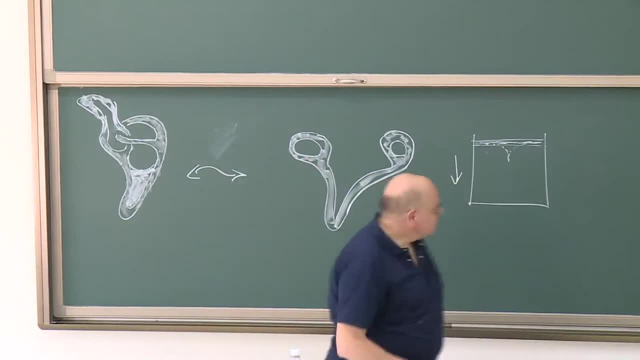 we have to stir them up a lot to put a lot of energy. Okay, now suppose that this fluid is heavier, but not so much so that after some time, as time passes, the fluid collapses here and at a certain point floats on in the bulk of the other fluid. 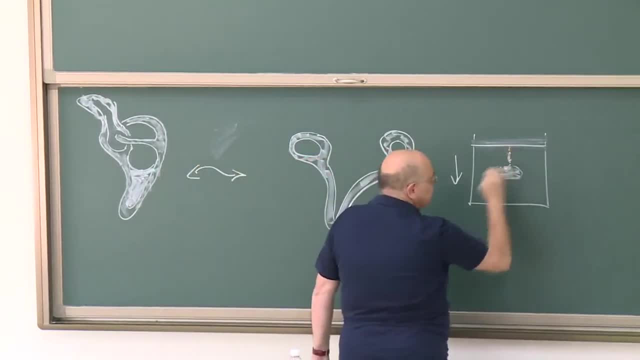 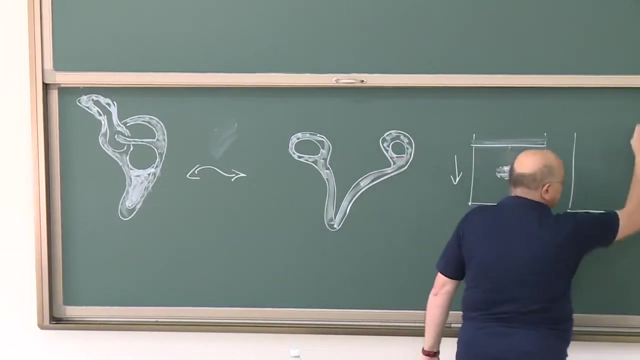 of the lighter fluid. Then there is a trace, and then this trace, as time goes to infinity, disappears. And suppose the fluid is heavy enough to be balanced by gravity at this stage. Then again, if you look at the situation at the beginning and at the end, 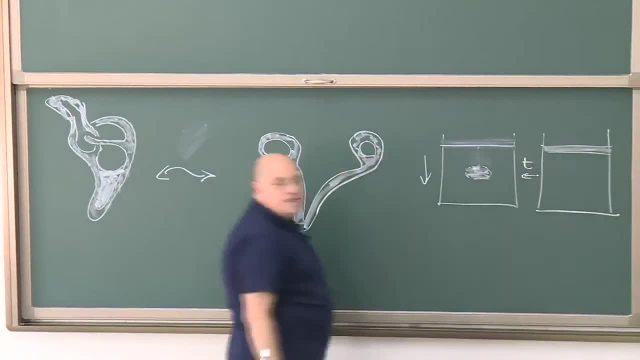 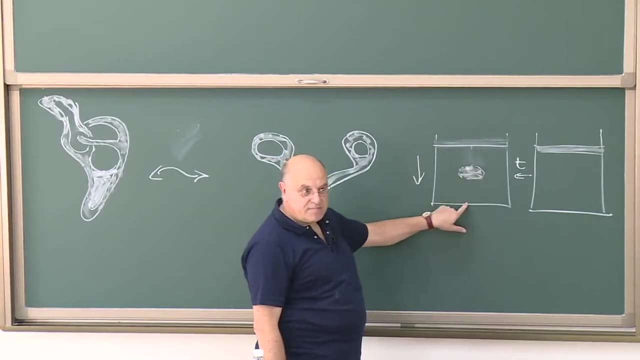 with the fluid here. that goes down like this: as time passes, then you have a change of topology of this ambient space Without cuts. How is it possible? It is a continuous deformation. There is another famous example, and this is quite recent and has been done experimentally. 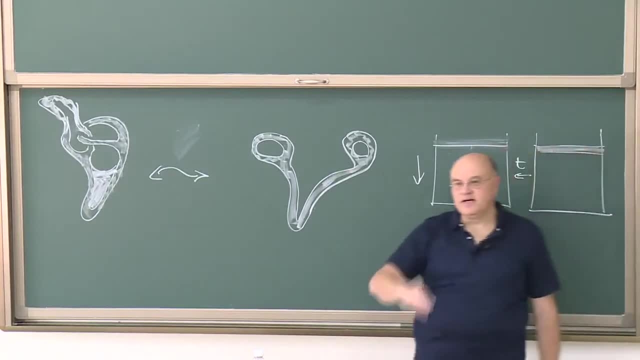 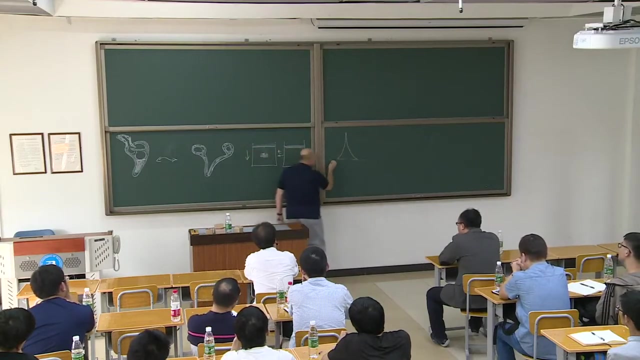 and this is, you imagine to drop something, a drop, and this drop goes into the water and then there is a reaction and you get a reaction from the water. so this is water and there is a cusp forming and by changing, is air. air and maybe some particular liquid. 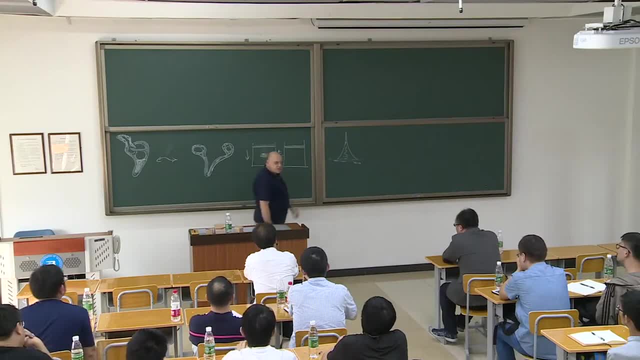 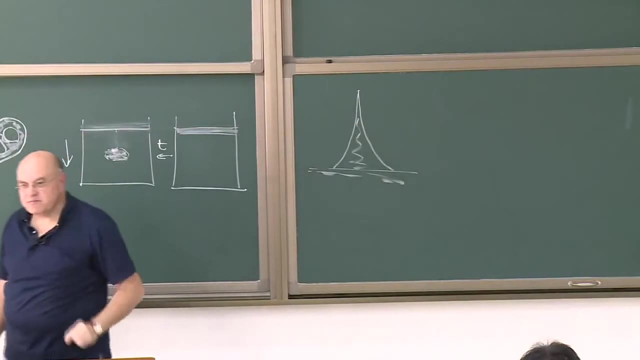 is not entirely water. you may put some glycerin, you may change some particular physical properties of this, but you can get a cusp, a cusp, and this cusp can be infinitely thin here, with an extremely thin radius of curvature. these problems share a common aspect. 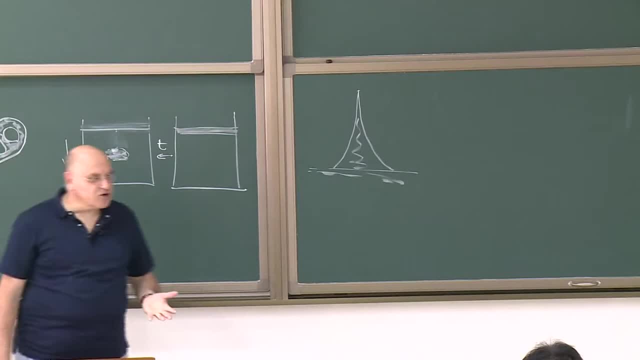 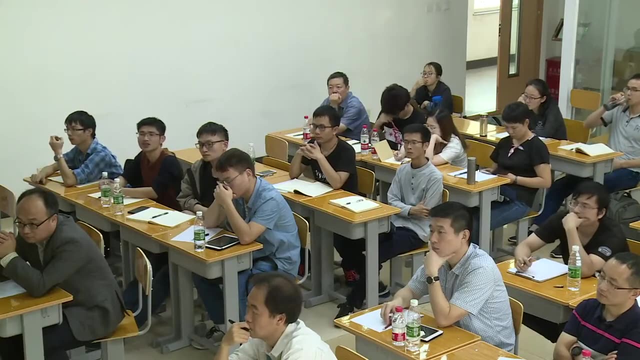 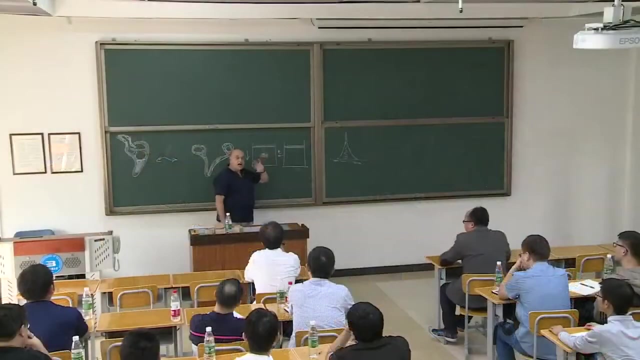 one aspect is what in mathematics is called singularity, singularities, singularities. they share also the problem that in this case there is no change of topology. here there is no change of topology under certain assumption- and here there is no change of topology- that there is a cusp. 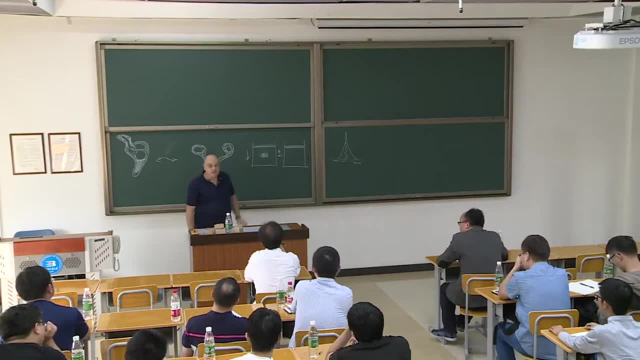 there is a point in space where the radius of curvature can be extremely small, extremely small. how small? oh very small: 10 to minus something meters. so small that we go to scales of quantum physics, so that classical analysis gives you the wrong answer because you get to a limit. 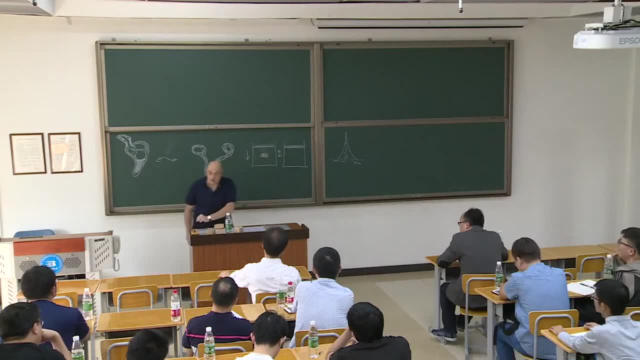 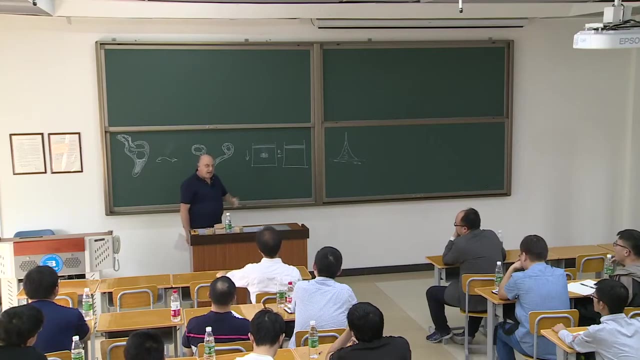 where you get wrong numbers for quantum aspects, you go below certain scales that are absurd. now, all these problems share common features: continuous change of shape without cuts and emergence of singularities in finite time. maybe so these aspects are central to modern research in mathematics, and indeed the problem of a singularity. 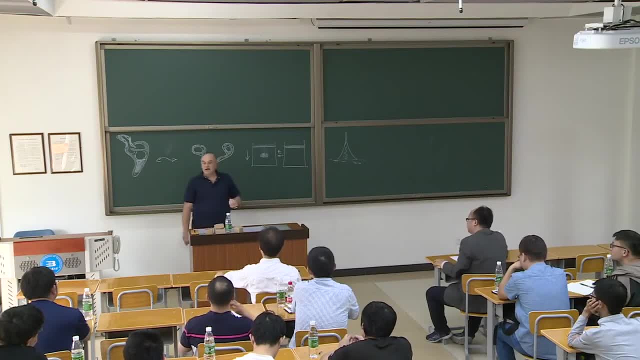 formation in finite time under equation of fluid dynamics is a well known clay problem of the clay institute is one of the eight unsolved problems, or seven unsolved problems of the millennium. it's a one million dollar prize for this. ok, so this is just to give. 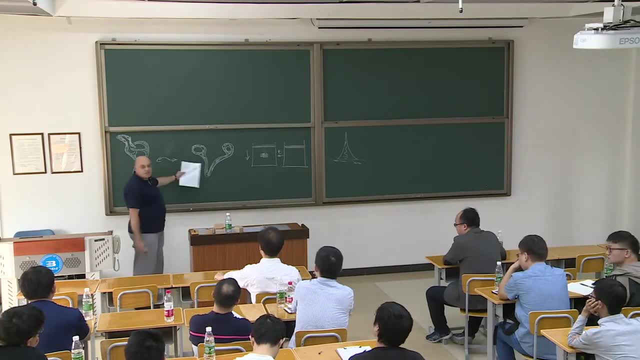 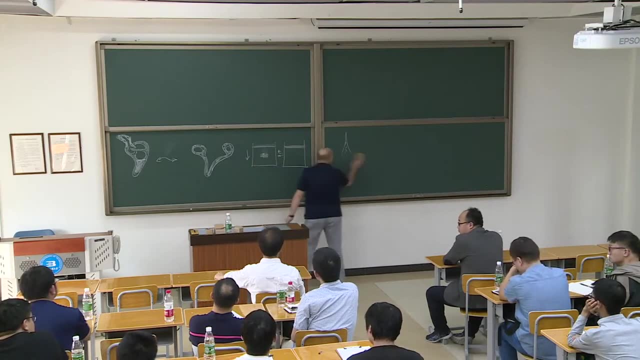 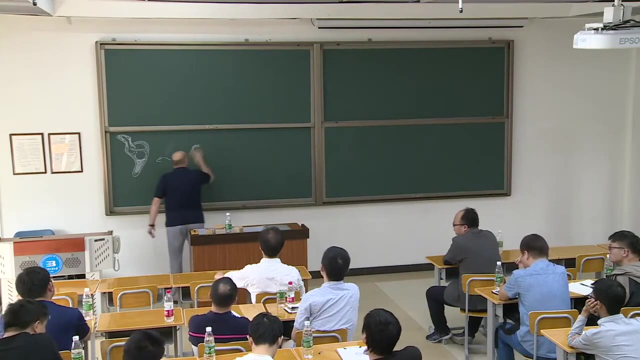 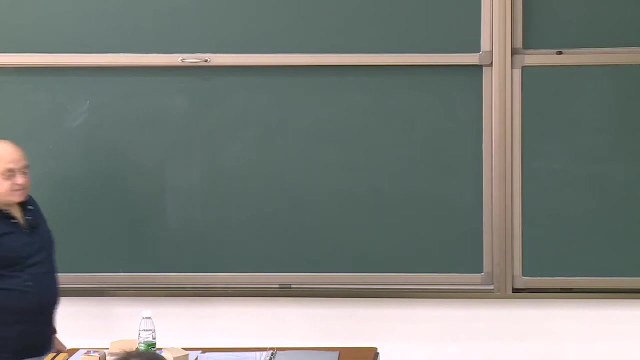 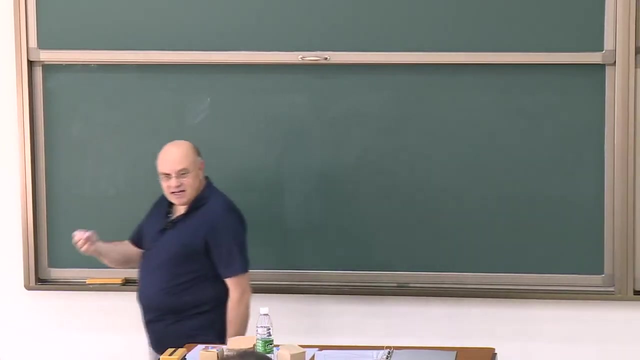 you an idea that these are challenges and represent all these phenomena, challenges for mathematics. so let's introduce some tools. first of all, I will focus on- to keep things simple- on ideal, fluid dynamics, ideal context. ideal is, of course, an idealization of the real world, but we may capture phenomena. 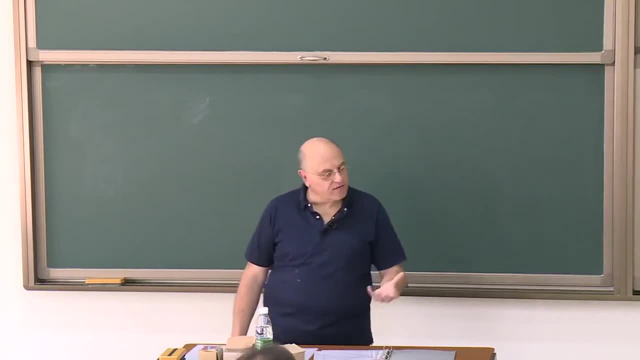 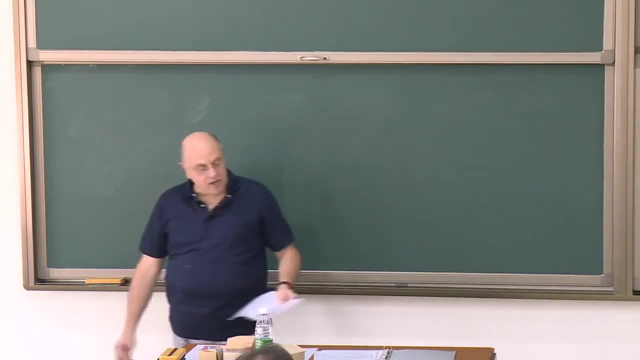 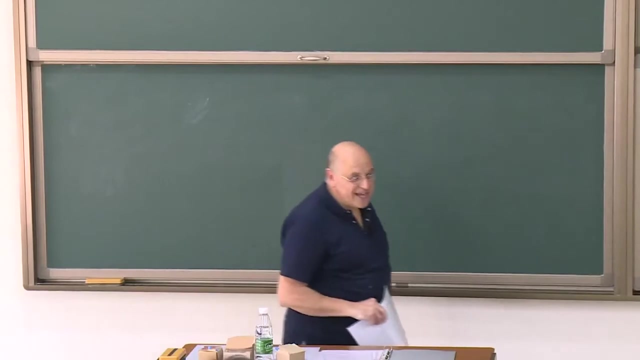 that, to a certain degree of approximation, are relevant for finer aspects. so I will assume a continuum hypothesis: everything is continuous till a very small scale. how small? any scale, we like any scale. so you know the problem of viscosity. if you go below a certain scale, then can we define viscosity? 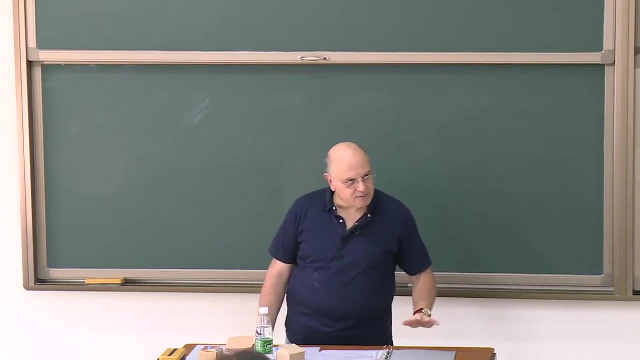 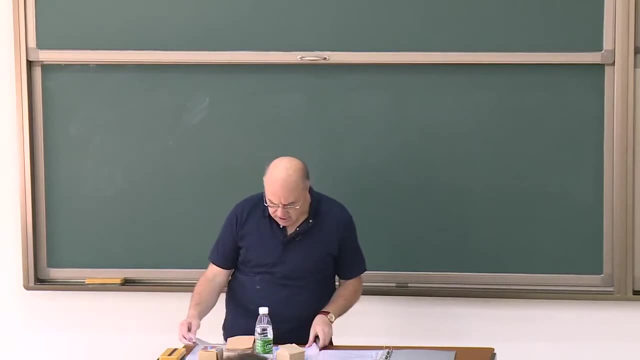 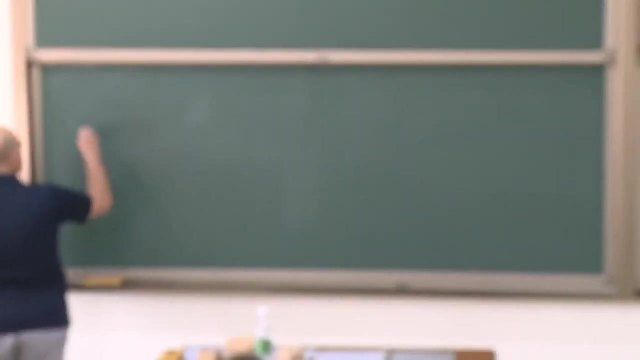 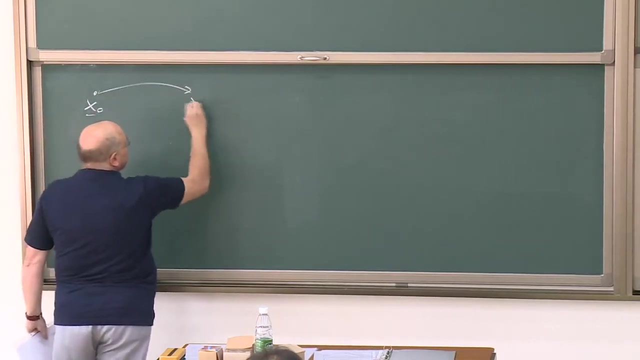 ok, so this is the first assumption: continuity and associated with that. let me just catch very briefly. what I wanted to stress is that we will focus on certain flow maps, so I will consider the motion of a fluid, say, from a point x0 to a point x. 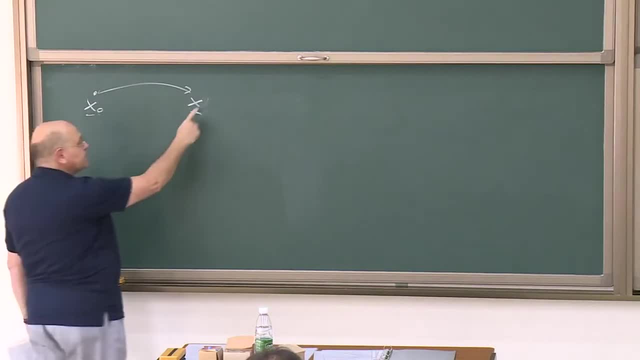 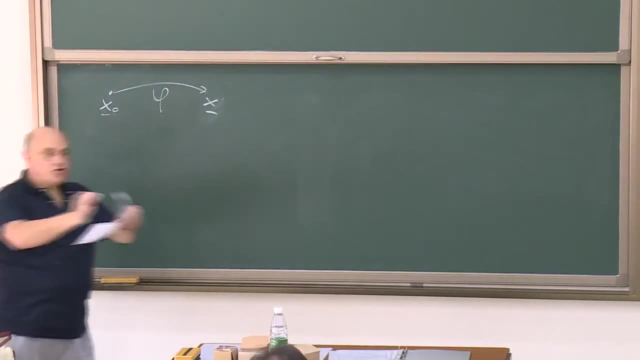 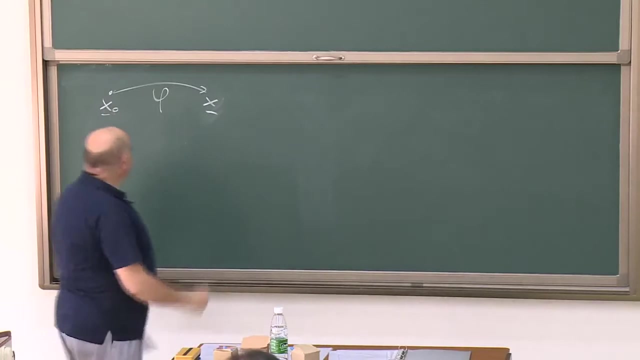 and x0 denotes the initial position, x will be at a certain time. and this is a flow map that transform a structure, a vortex, a magnetic field, something brings a point in the fluid to the new position. now this flow map. I constrain myself to work in a set of 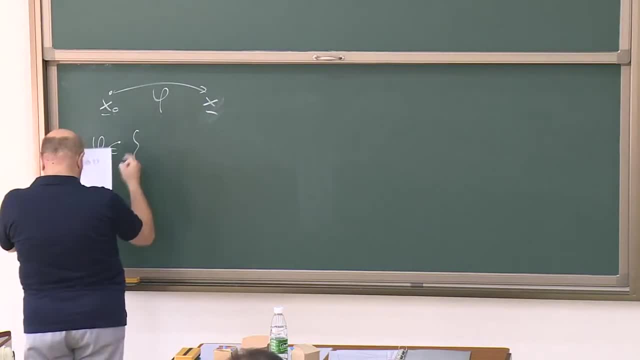 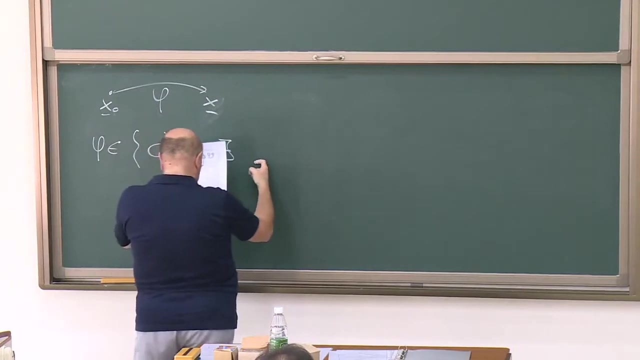 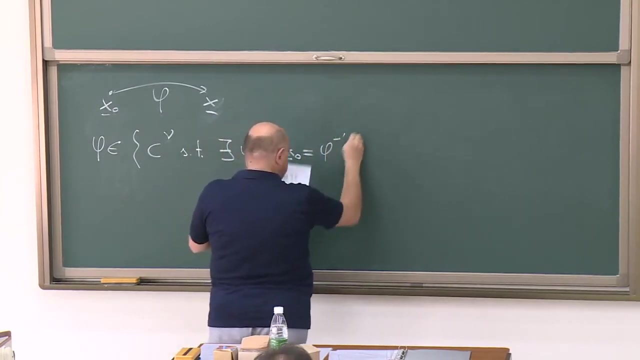 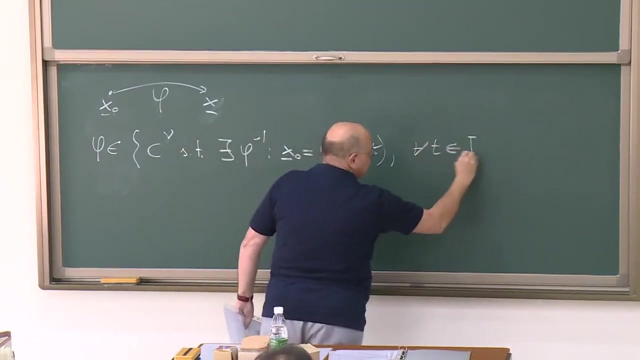 flow maps that are like this. I take these flow maps to be continuous, smooth, with new large enough so that we have a inverse map phi minus one that gives me x0 through the inverse map x and t. if we have t- and this is for any t finite in a, 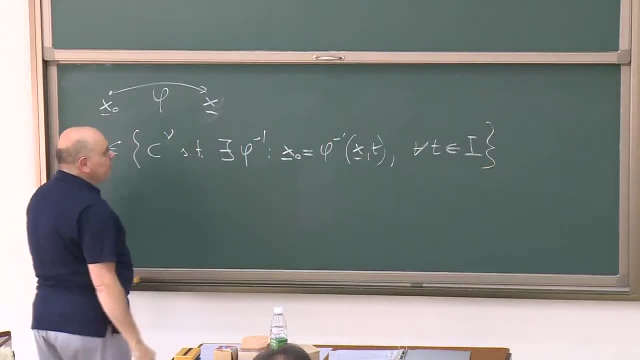 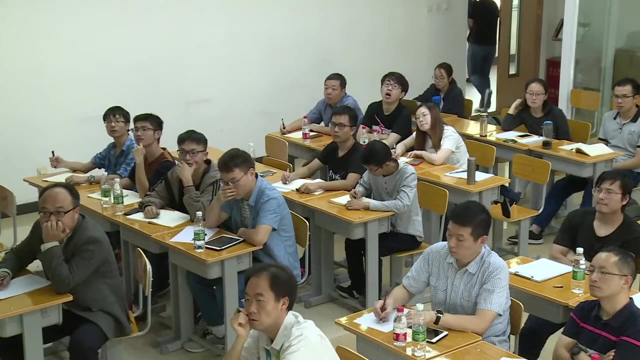 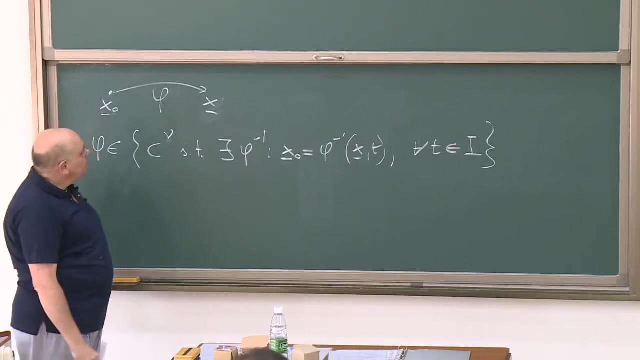 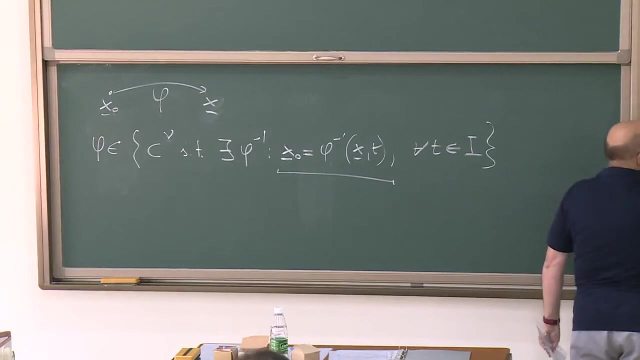 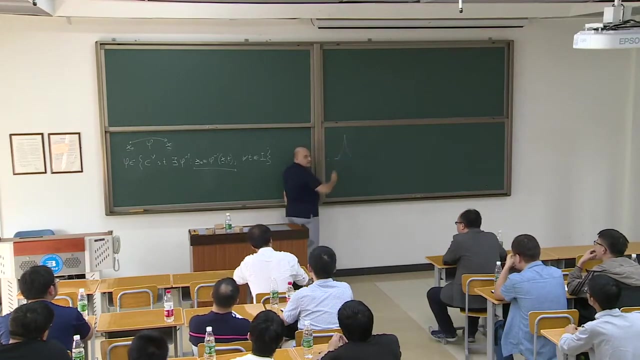 finite interval to new, to a number. yeah, yes, yes. now, this means this means that we can always go back to x0. right, we had this problem of the cusp. remember each point when, when the surface produce this cusp, each point of water goes up, up, up, up. 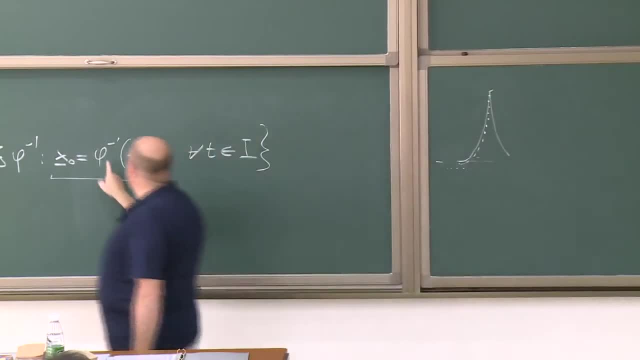 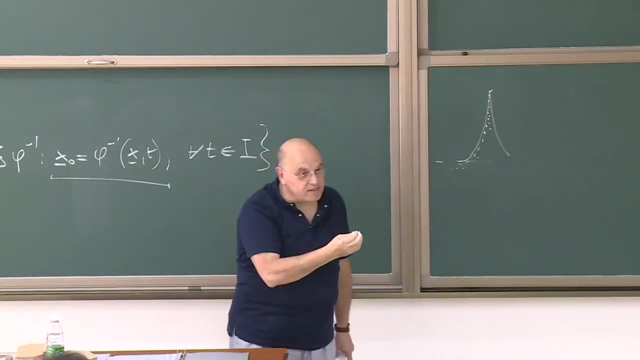 and at a certain point we should be able, from this phi minus one, to distinguish here every single point that collapses to one point which contradicts what I said. you can reverse this experiment with the usual experiment. you know tap water. you shut up the flow of water. 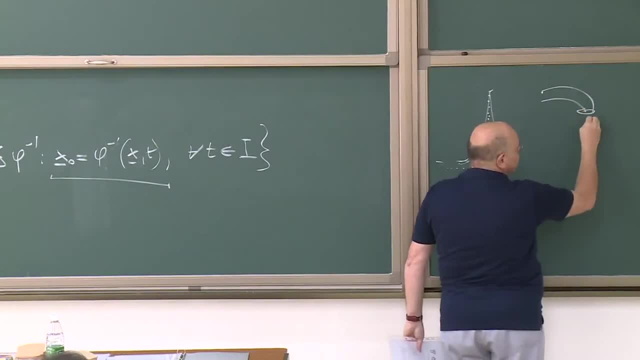 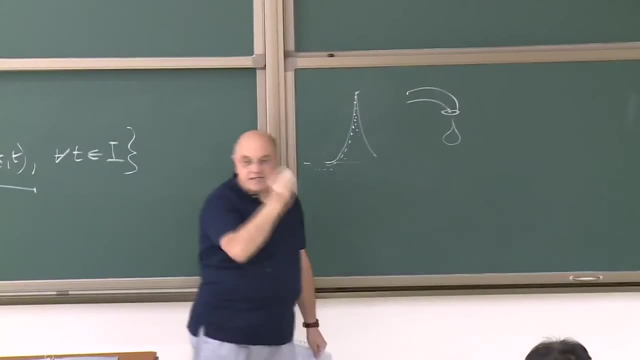 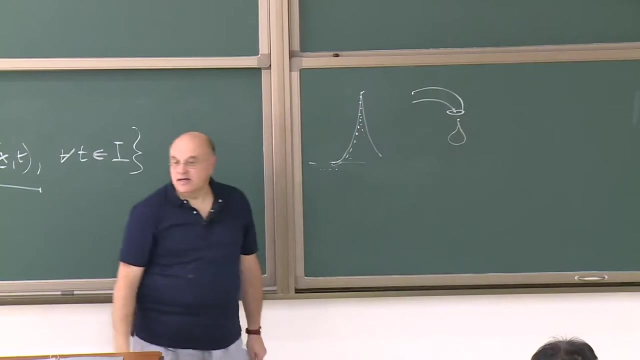 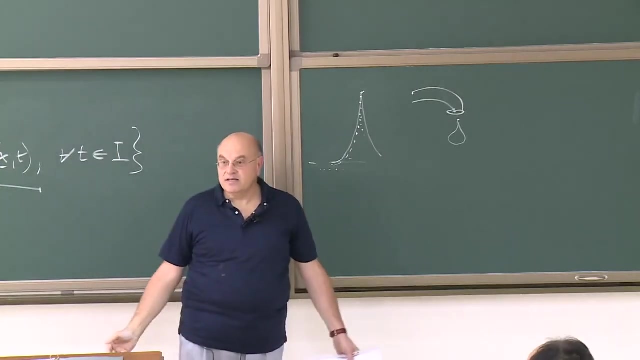 and at a certain point, from the water forms a drop and there is water here. at a certain point the drop start to detaches from the fluid. what happens to this point? this breaks down. we have no longer inverse mapping well defined. we have problem with the inverse map. 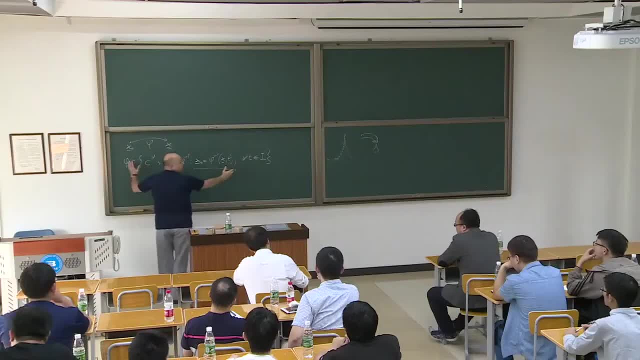 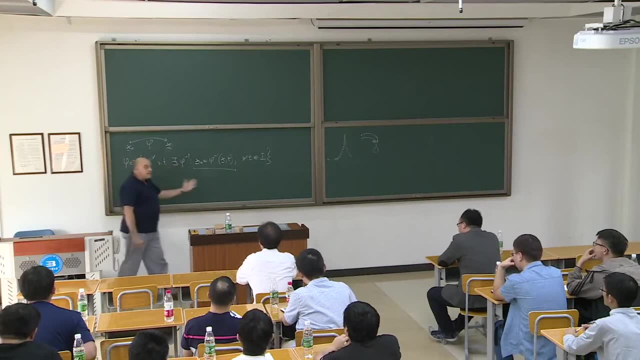 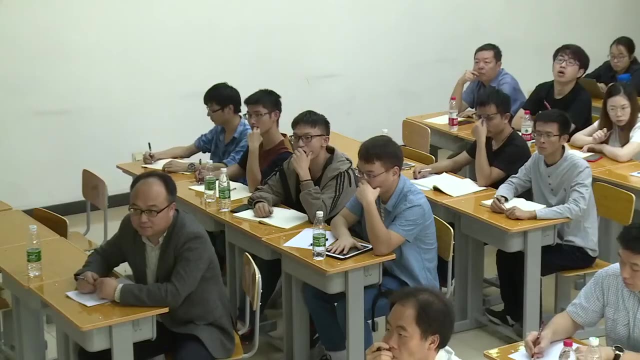 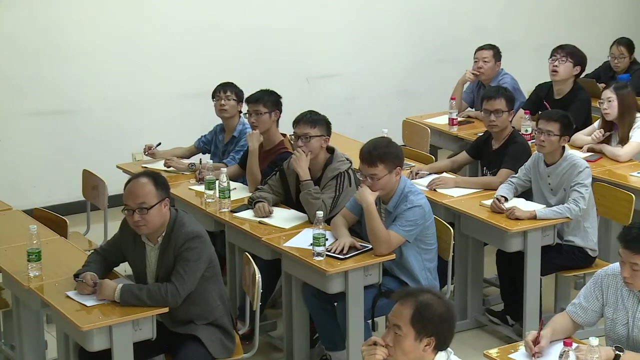 so you see, as we define our fluid to be continuous with the inverse that exist at all time, we immediately cut out many, many important problems, many important problems of real life, but also mathematically. mathematically, here we may have problems for a singularity, for the inverse of the flow map. 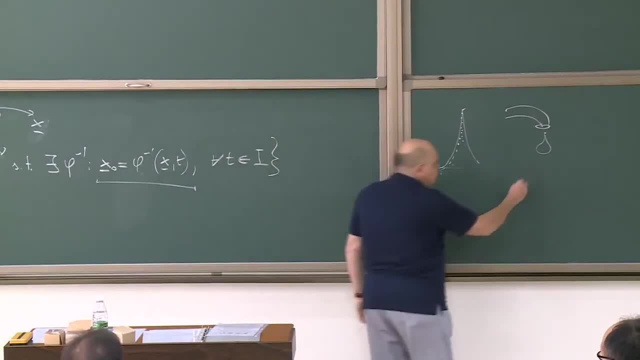 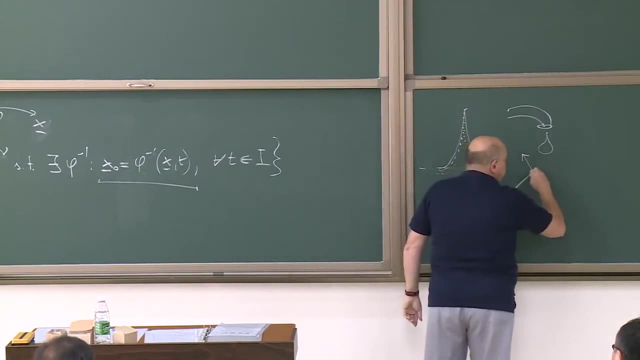 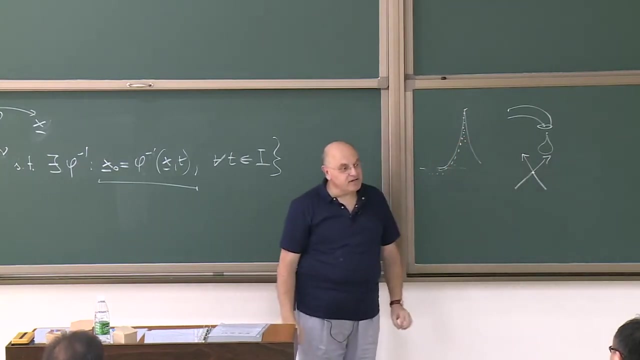 that is ill defined or even worse, in some natural circumstances. we have, instead of a cusp, we have an angle, and an angle is, to some extent, is same problem. where is the tangent at the angular point is ill defined. we have a problem there too. ok, so I will. 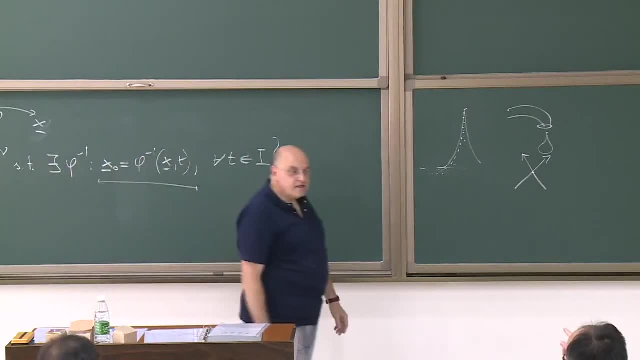 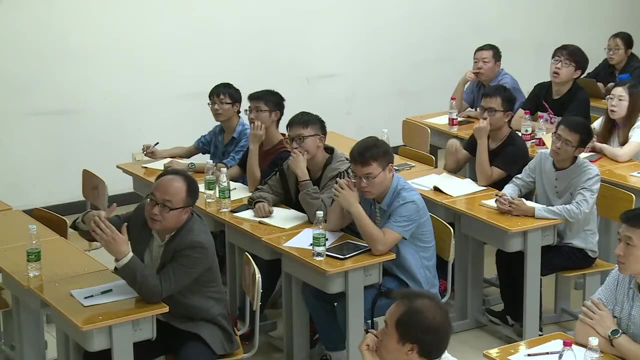 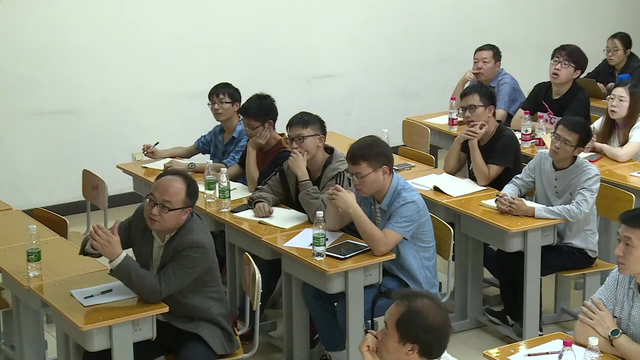 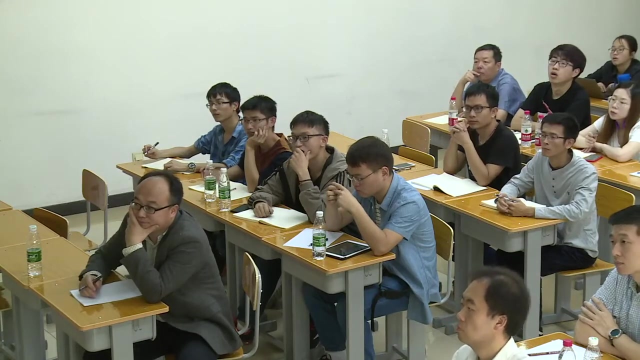 confine myself. it must be a singularity. oh, sure, sure. why it must be a singularity? it can be. it can be perfectly well defined. yeah, I know, I know, it depends on the context. it depends on the context, ok. so what you are thinking about is: 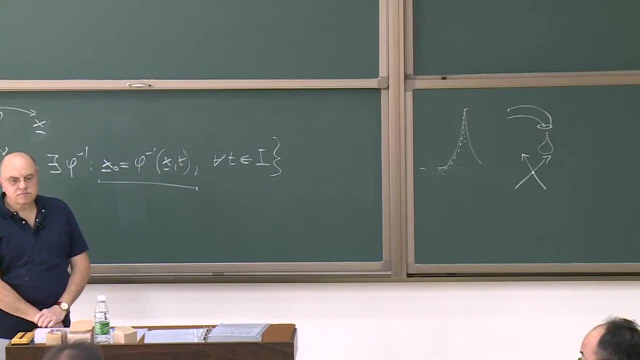 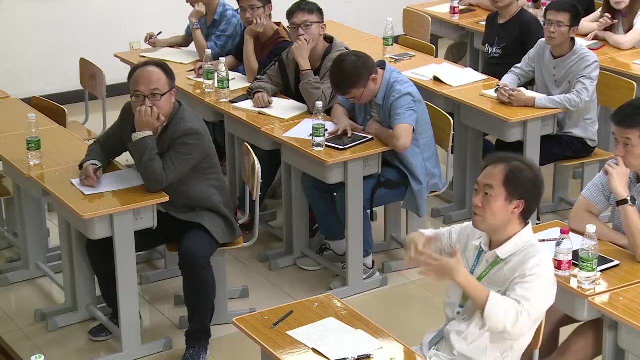 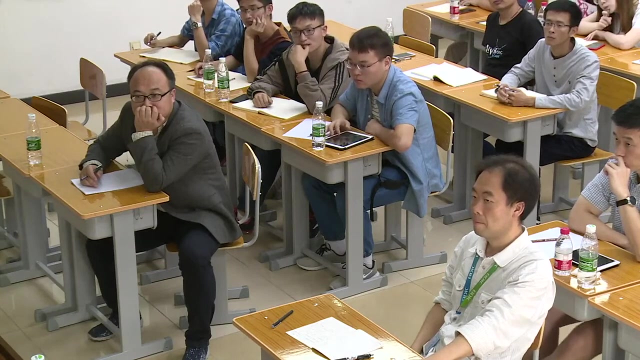 we just study the peer rate, topology is conserved. so that just means the very moment topology changes. so we just throw away that case. exactly what I am saying is that, what you will see, we take this as our working set of flow maps and by doing this we cut. 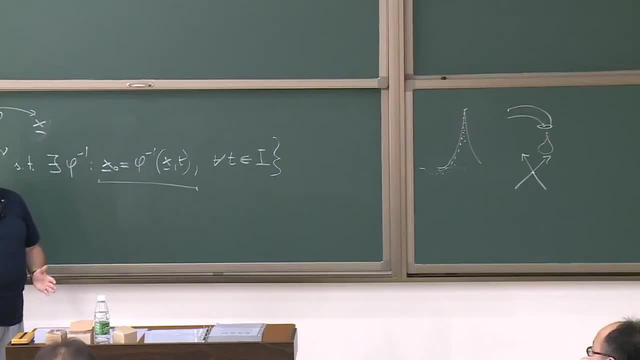 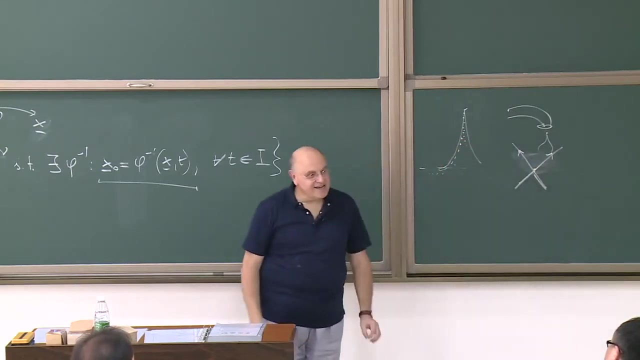 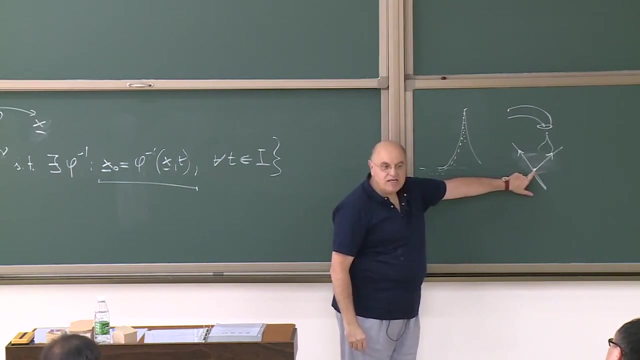 out many, many, many problems that we don't know how to handle. how to handle? let me go back to the point. suppose we have two field lines that intersect exactly. what is the physics there? what is the mathematics there? can we talk about the tangent at a point there? 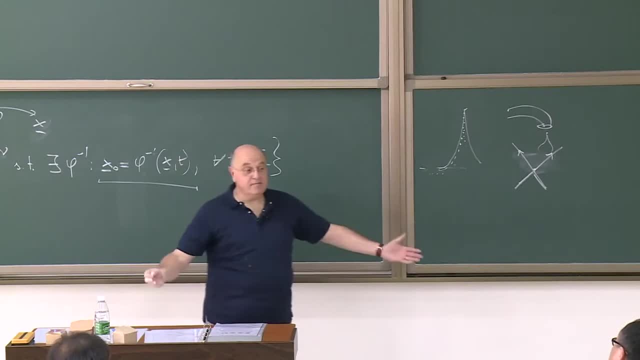 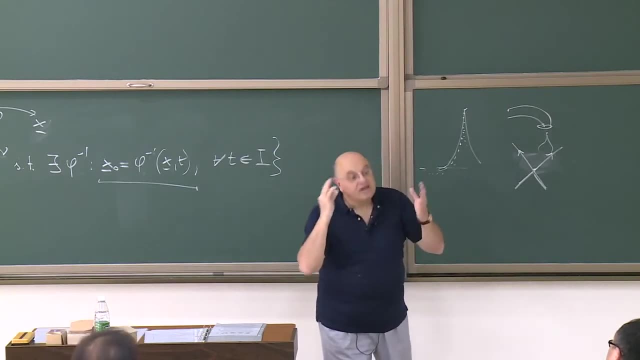 this is normal problem tackled by many context of physics is called reconnection the state of a field line that goes through the other at the instant of the intersection. there is difficulty to tackle this problem because we don't have the mathematics, so my emphasis here is that we are using 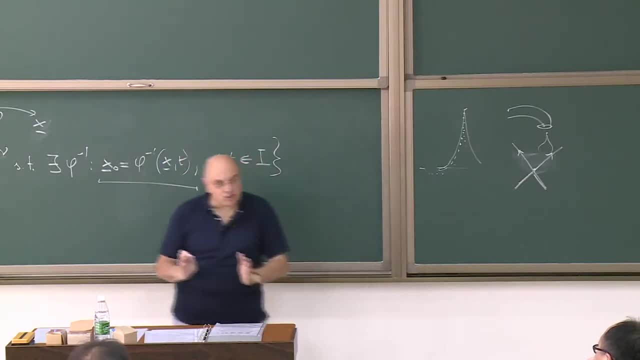 old style mathematics, but we need also to think at the same time of something new in mathematics, to have new techniques to handle these problems, problems of singularities that are associated with changes of topology. ok, before I mentioned in the first diagram, I told you there is no change of topologies. 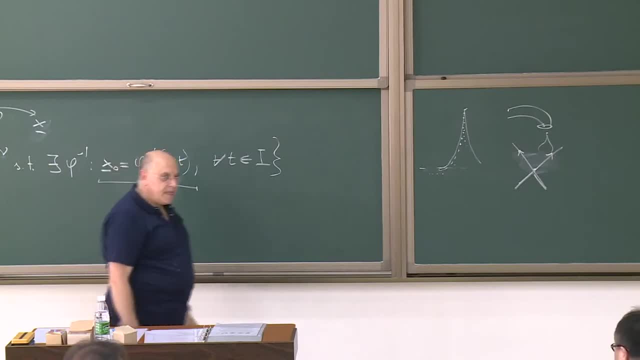 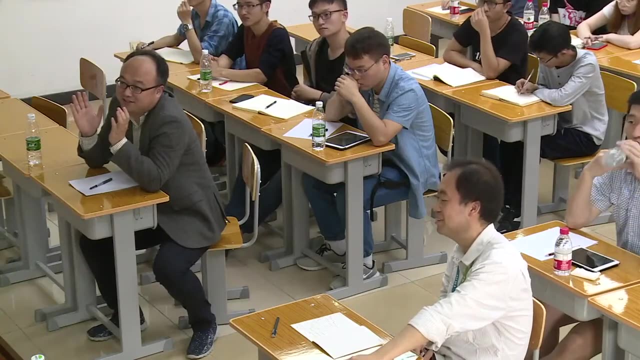 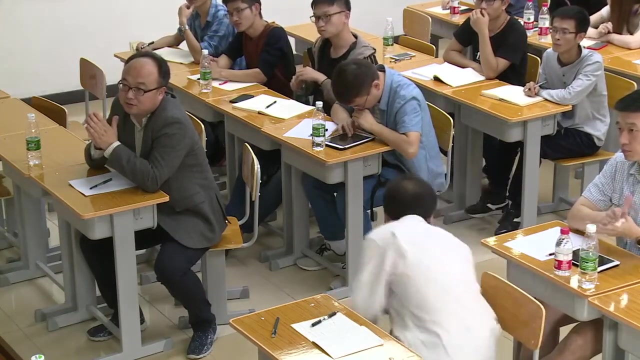 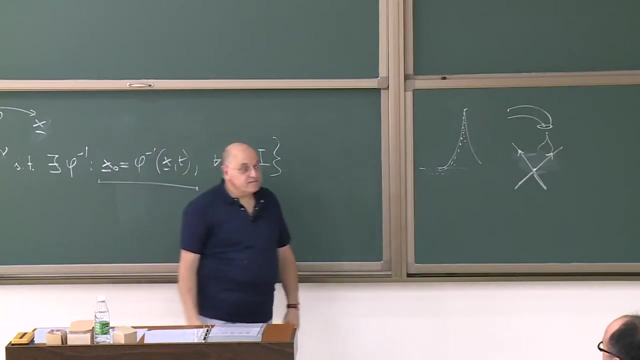 continuous deformation at all times. what is a singularity? it depends on the context. it depends on the context. yes, it depends on what you are talking about. there are many ways to talk about singularity, for example, when this breaks down, when the inverse breaks down, when there is no. 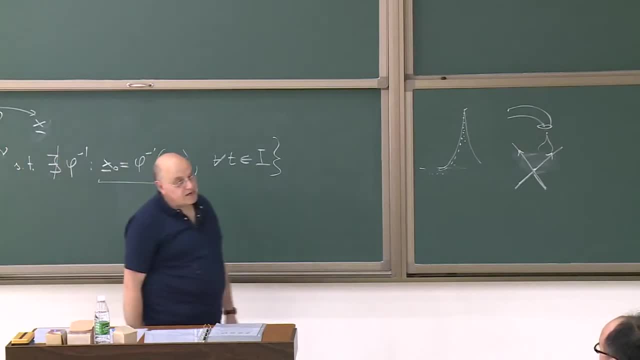 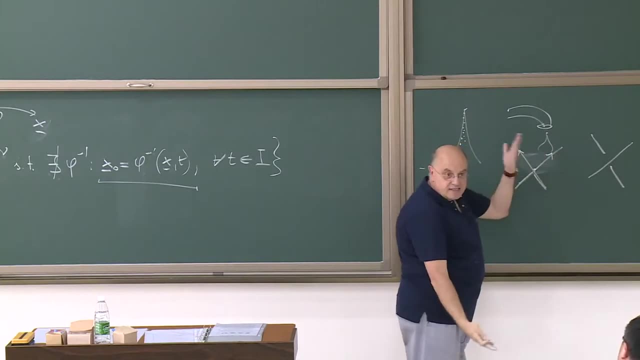 inverse to the flow map. then you have a singularity because you cannot identify. suppose you have a system like this: two field lines. suppose you orient these field lines and suppose that now they touch. can you go back to here or can you go back to this situation? 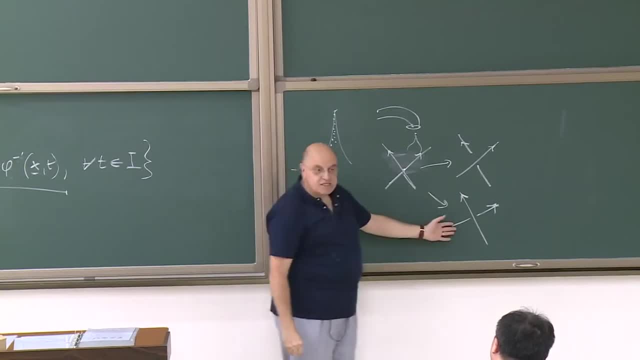 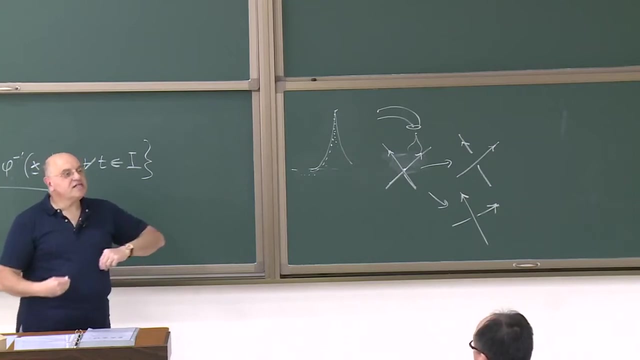 which one. this is maybe previous time, this is after time, or the other way around, but there is no way to know it from this, because you have no inverse. yeah, this is one of the key points of singularity. yeah, losing the inverse, and so it's a diffeomorphism. 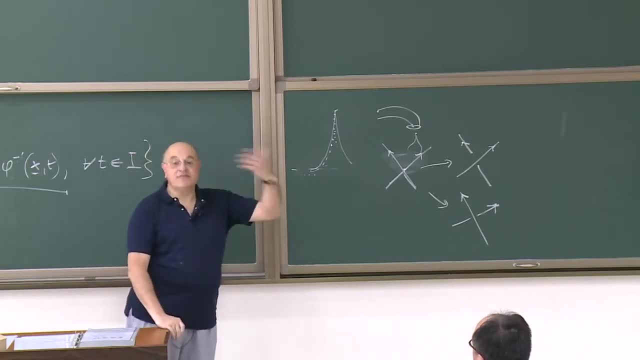 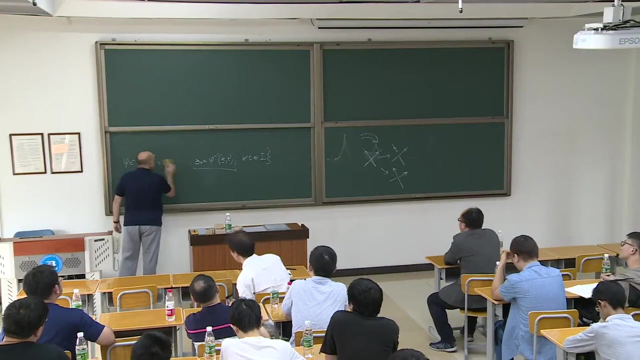 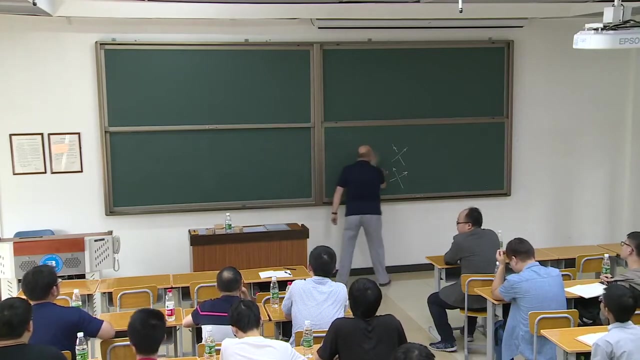 is a continuous deformation that is differentiable at all times. so diffeomorphism, but diffeomorphism may not have the inverse map, alright, so this is just a little preamble. ok, let's start with the first tool I told you we are going to use. 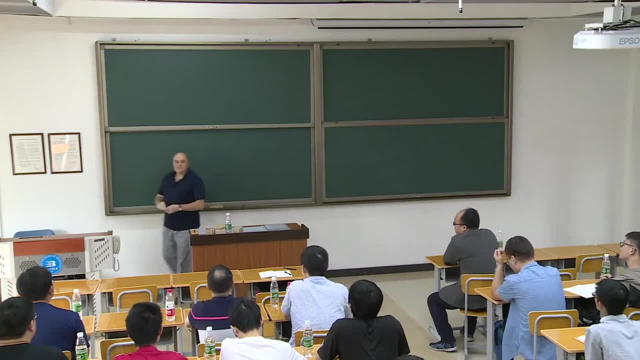 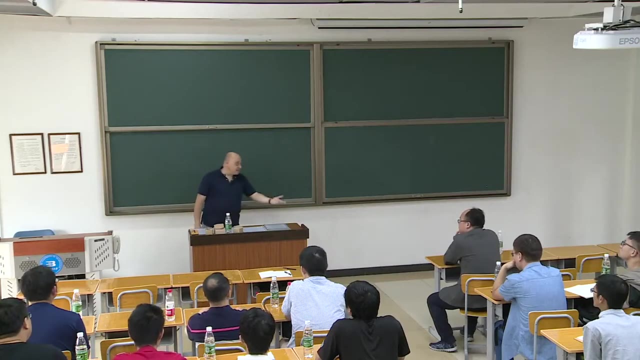 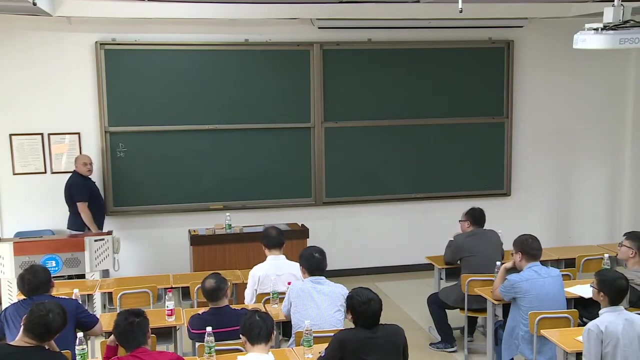 some tools. I have no time. everybody is at home with the concept, of course, of velocity, of acceleration, acceleration. we know how to define acceleration in space and time in classical physics. I will use this notation: d for the total derivative of a quantity. suppose that I consider x as my space variable. 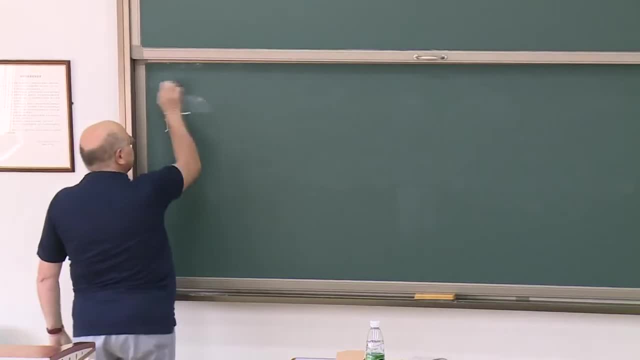 and I consider this dx dt, then dx dt, then dx dt will be, if x will be a function of, say, a arc length and time. suppose I go to velocity I take acceleration, it's the same thing. suppose I take the velocity u, it's the function of. 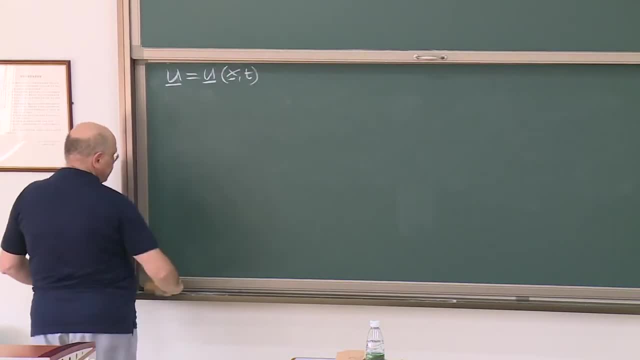 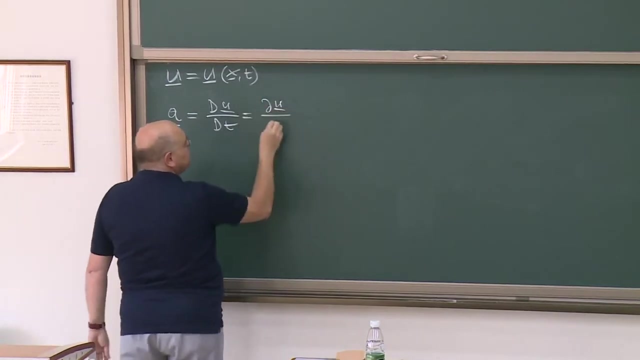 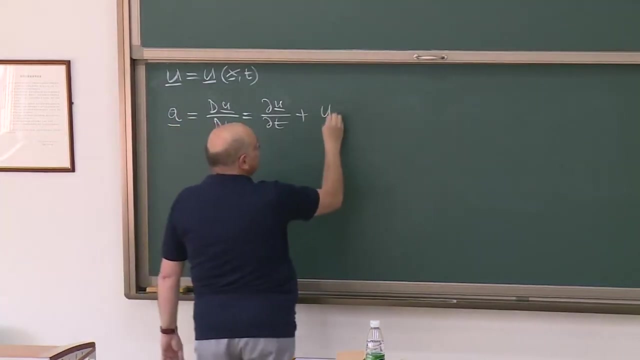 x and t. then I have acceleration a, defined as du dt, and this du dt is given by two contributions, as you know, we have a contribution in terms of time and a contribution in terms of space. alright, are we happy about this? we have u dot rad u. 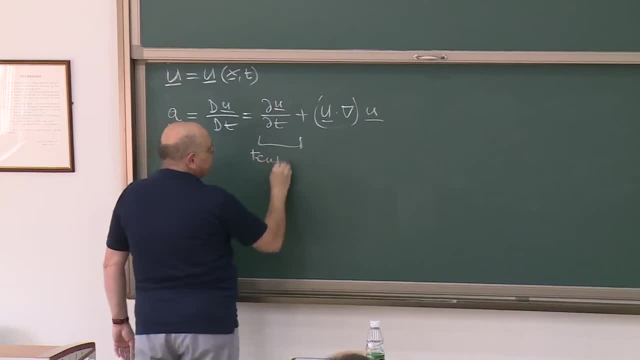 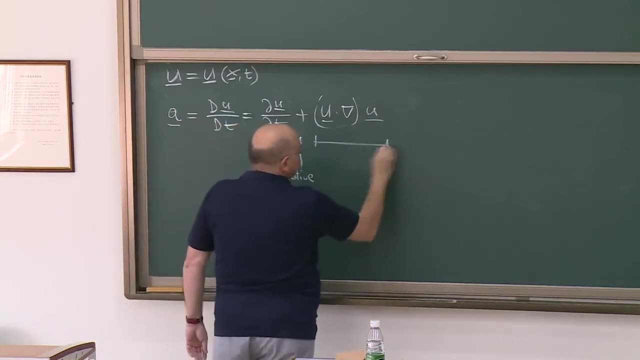 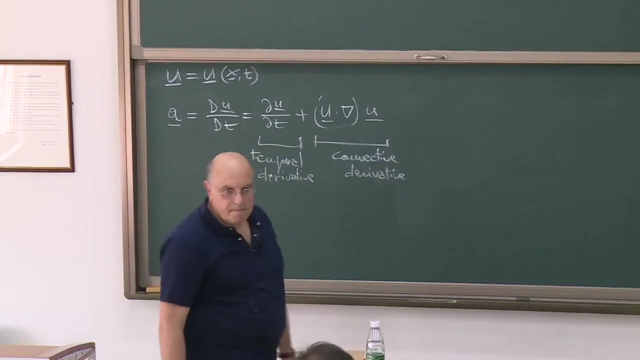 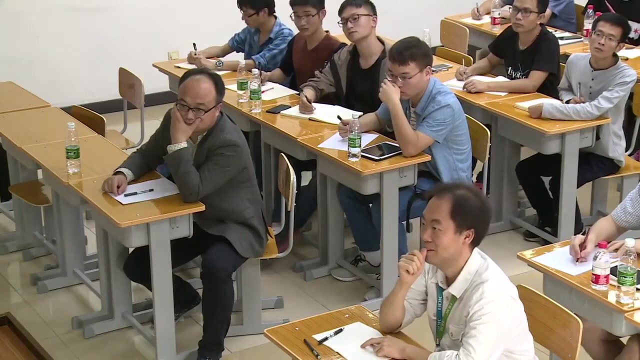 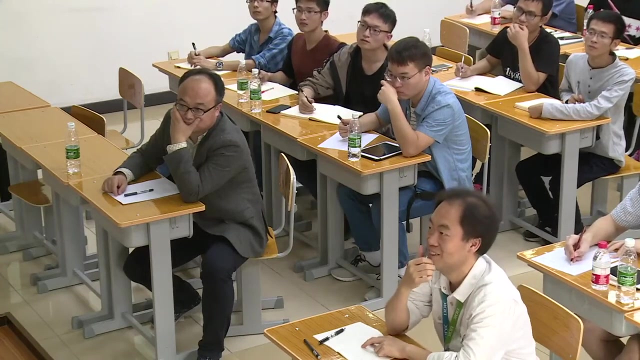 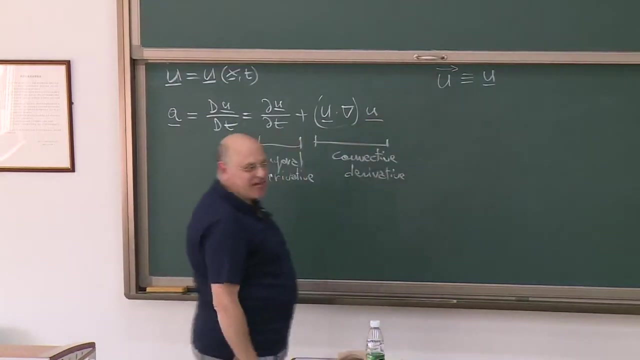 this is called temporal derivative and this is convective or transport derivative. ok, this is standard. yeah, I have to tell the students your underlying u, this is our u. you use this notation perhaps? yeah, ok, ok, alright, I will use. I will use this one. I will try to use that one. 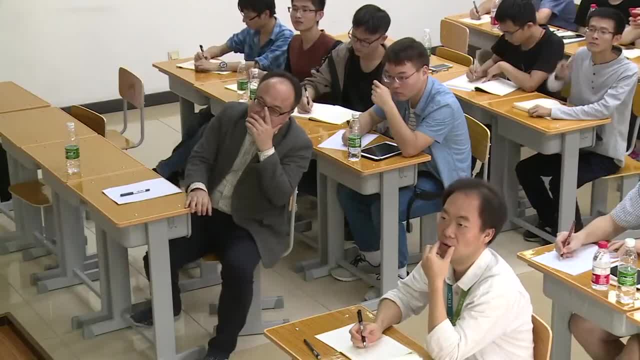 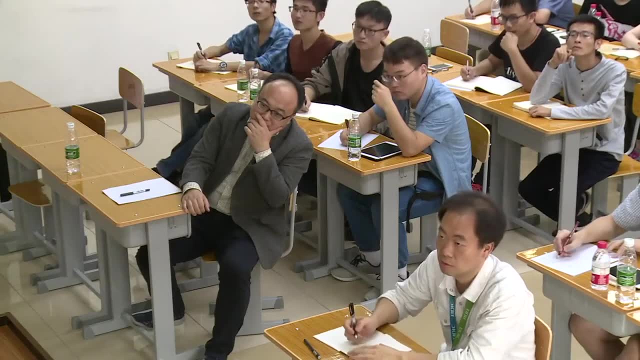 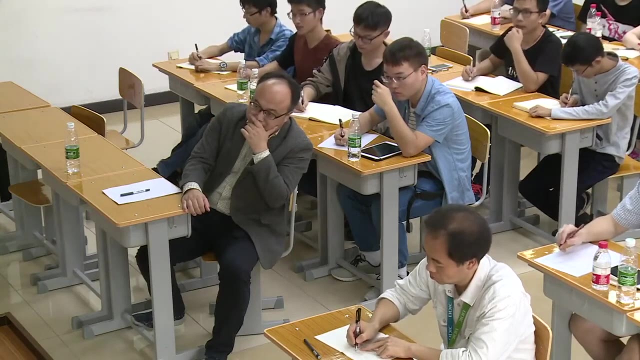 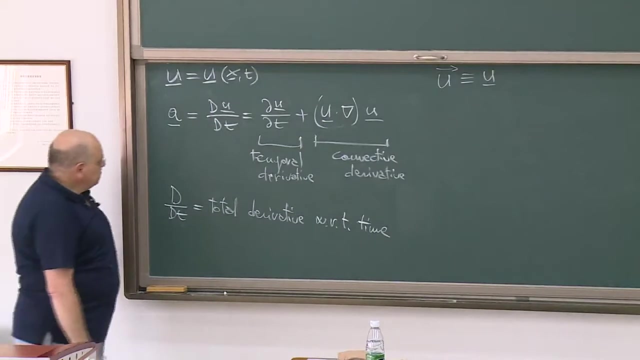 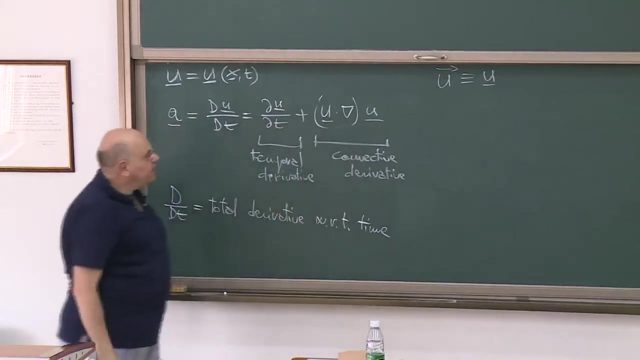 alright, this is- yeah, this is the total derivative d dt. total derivative with respect to time. ok, so this is important, right, because there is a non-linear part, and the linear part this is the transport of u in space and this is the transport, so to speak, of u in time. 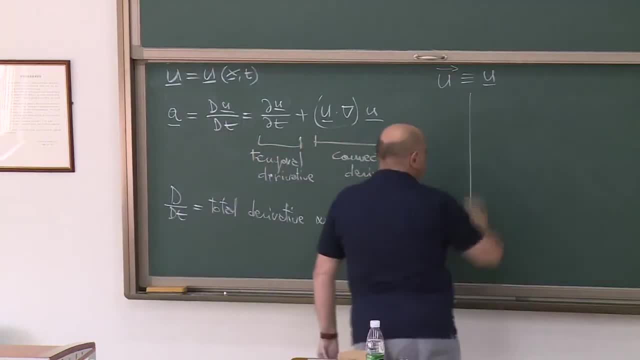 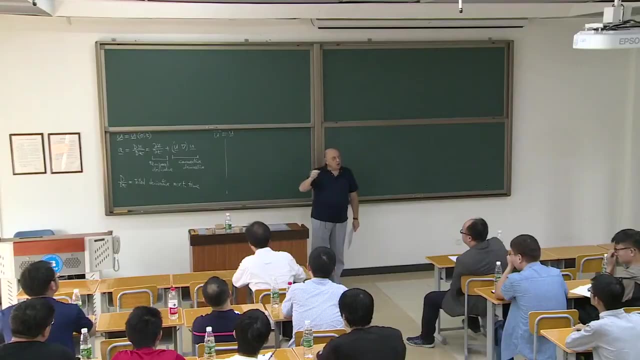 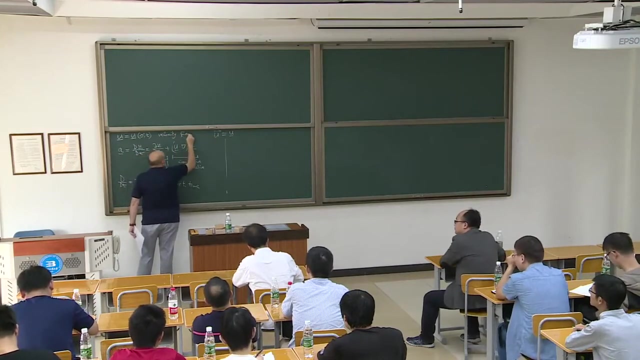 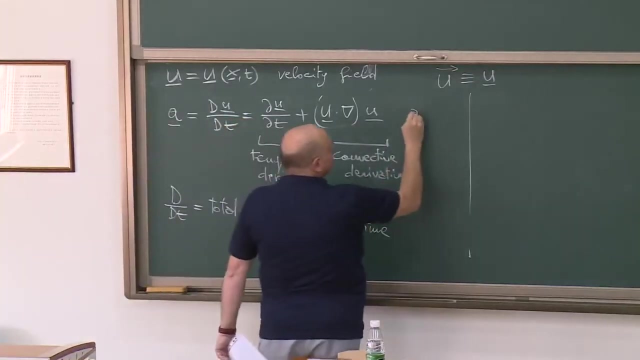 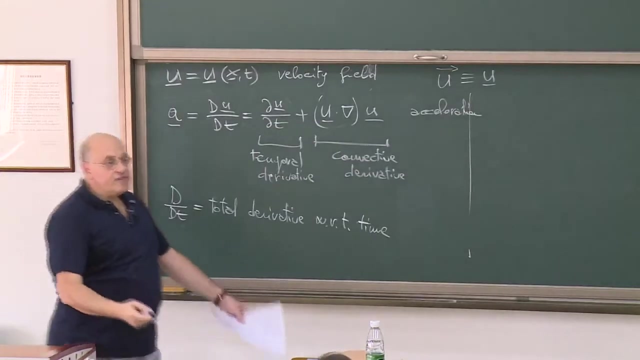 ok, one other basic notion is the notion of field line, so I will stick to u. u is the velocity field. velocity field- this, as I said, is acceleration. ok, the other, the other fundamental concept, is the concept of field line. so let me use velocity, I will. 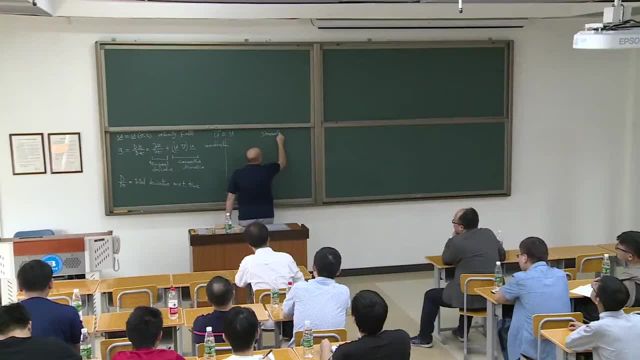 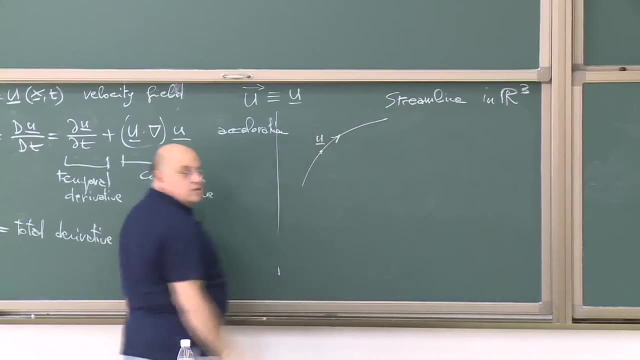 call streamline. I will call streamline a line in space in R3 where at each point, u is defined to be identified with the unit tangent. ok, so if we prescribe the unit tangent at each point, at each point of this line, say this line c, we have the unit tangent. 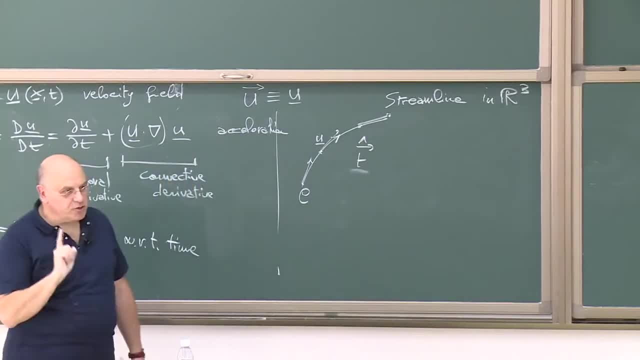 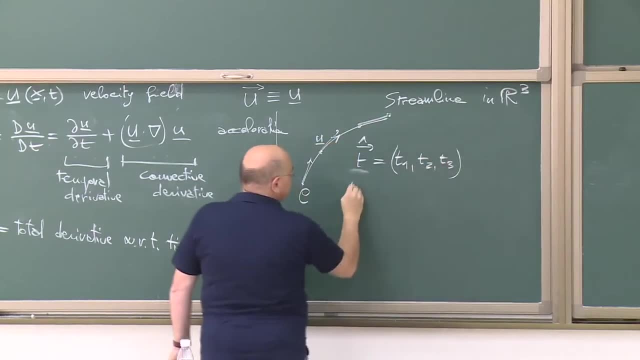 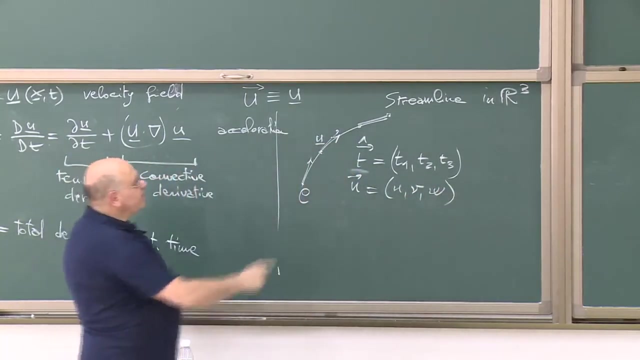 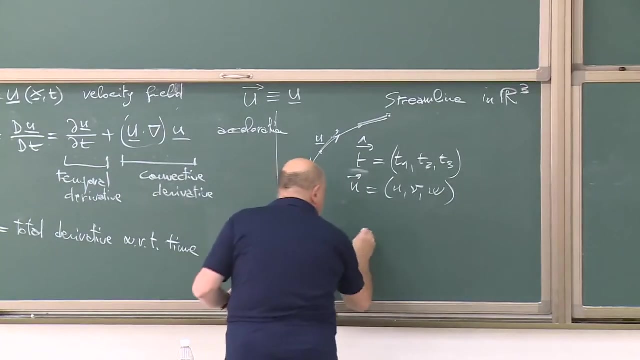 t, t hat, because it is unit, and t hat is made of three components: t1, t2, t3, then u will have three components: little u, v and w. then the definition of a streamline, a velocity line, is simply given by u over, if you like, dx. 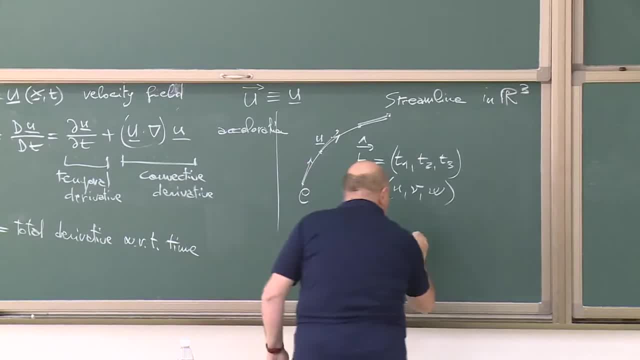 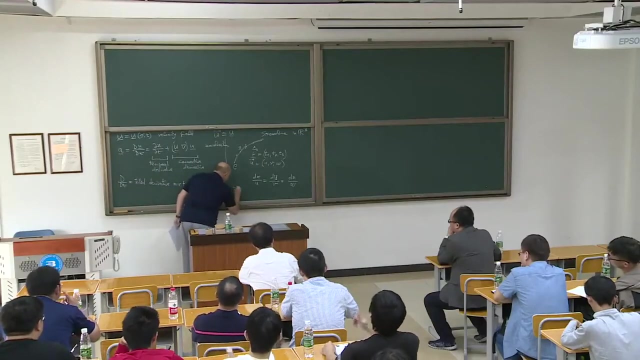 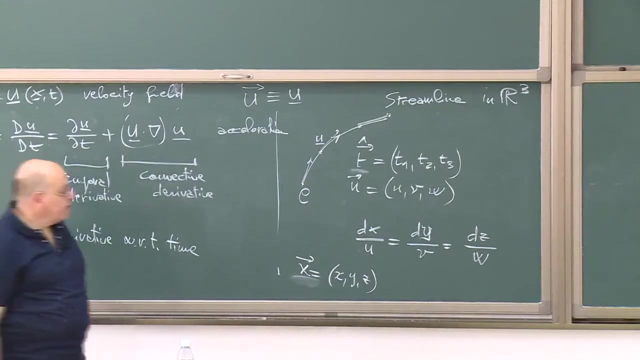 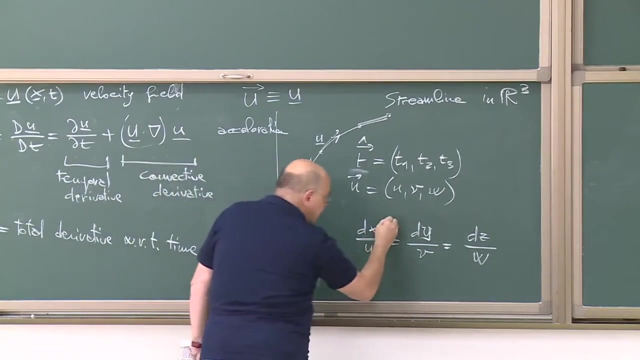 over u, equal dy over v and this is equal to dz over w. if, if the space x, x is given by xyz, this is the definition of a streamline. ok, now notice that we may divide everything. we may divide everything by ds, ds, where s is a coordinate, is a coordinate. 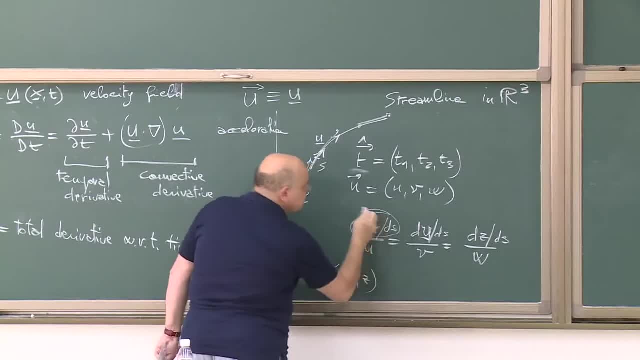 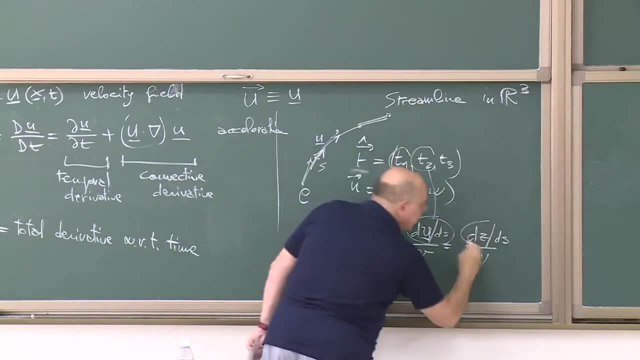 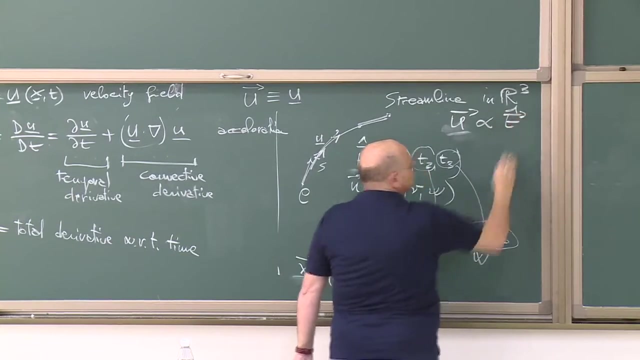 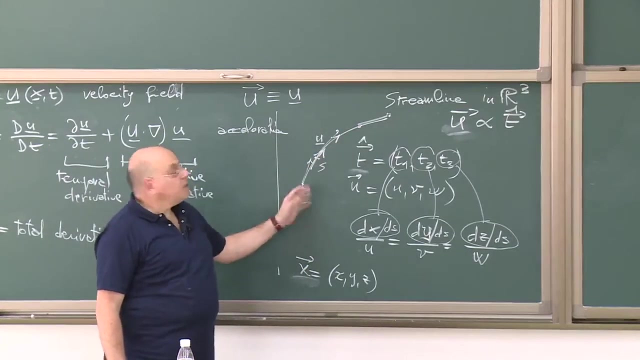 here and we get dx ds as t1, dy ds as t2 and dz ds as t3. so we identify, as I said, the velocity u with the unit tangent t. ok, so this is a vector field line. I use it. the word streamline, I use it for the velocity. 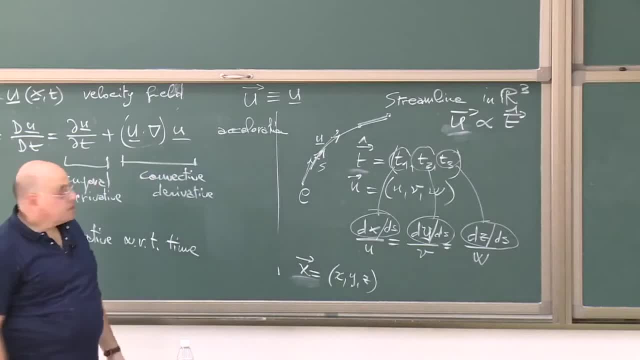 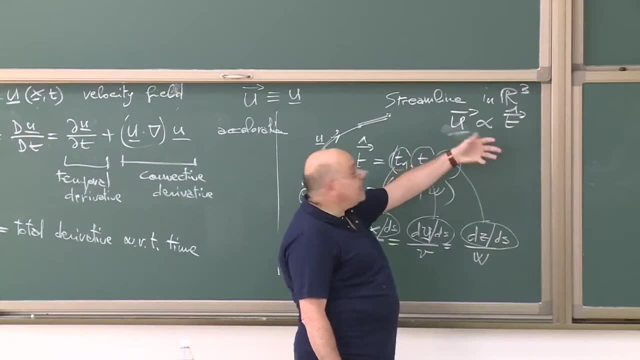 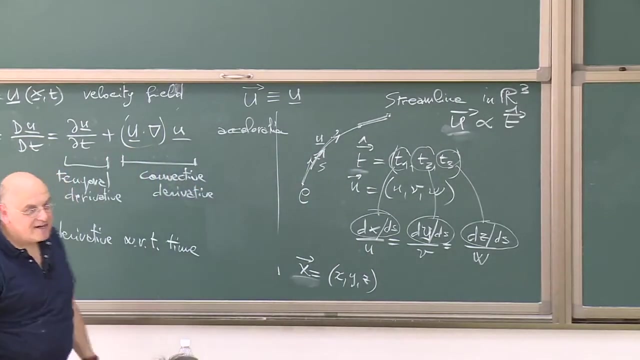 I can use any vector field, magnetic field. so how do I define a magnetic field? the same thing. I have a, b, the magnetic field that is identified with the unit tangent on a curve c in space. I'm cutting short a little bit of, a little bit of. 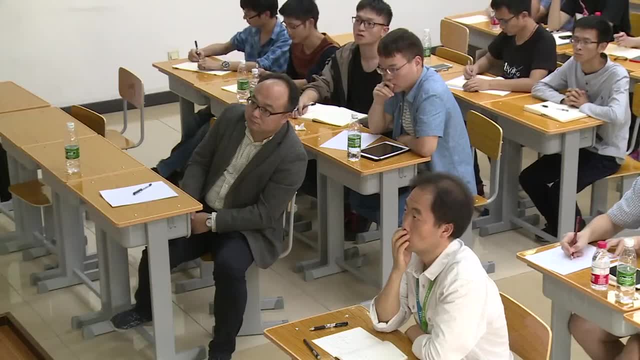 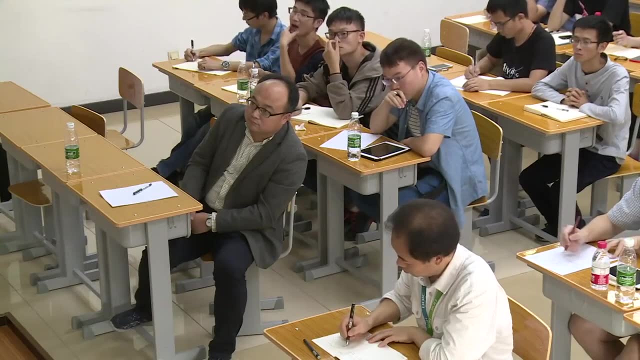 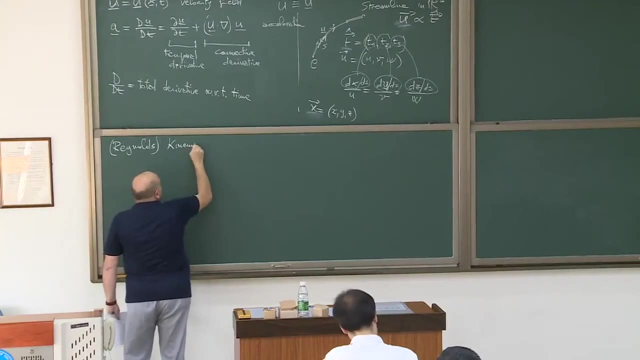 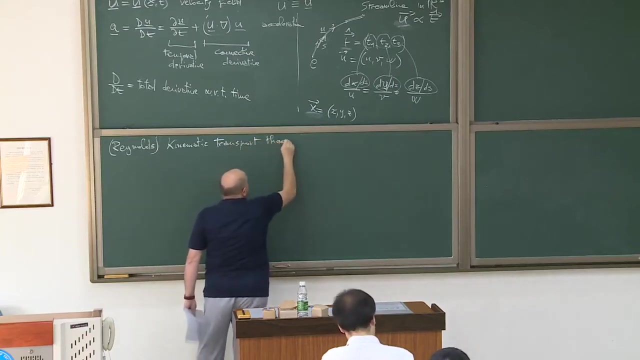 introductory notes on this. so field lines will be very important for us. we will talk about the collection of field lines and now I'd like to introduce you a kinematic result due to Reynolds. so this is a kinematic transport theorem. this is useful because we want to 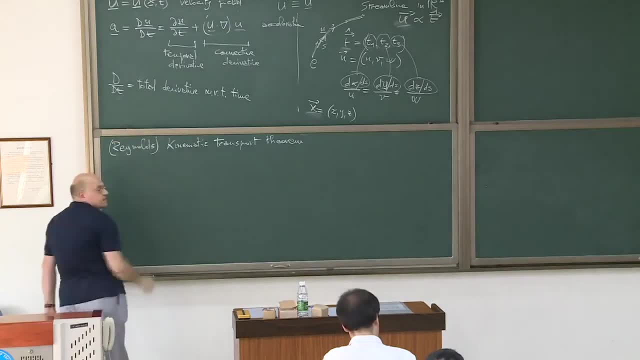 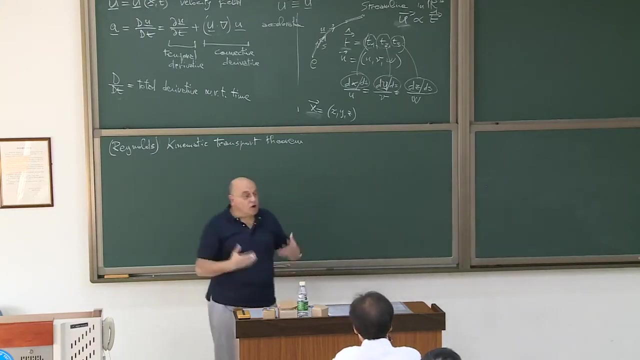 apply this derivative, the total derivative, to quantities, for example mass, but defined through an integral. ok, mass is just the integral of the density over the volume, and we want to use this derivative on integrals, on integral quantities. so we want to know how this quantity works. ok, so we need this theorem. 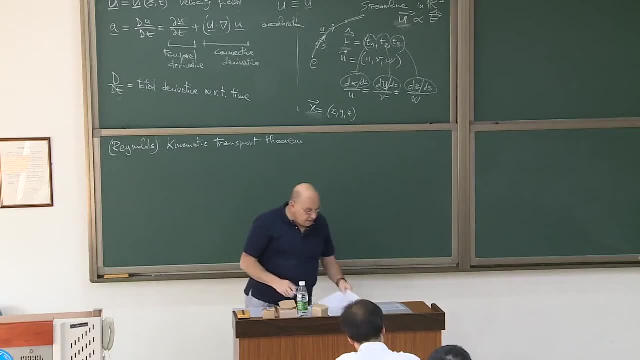 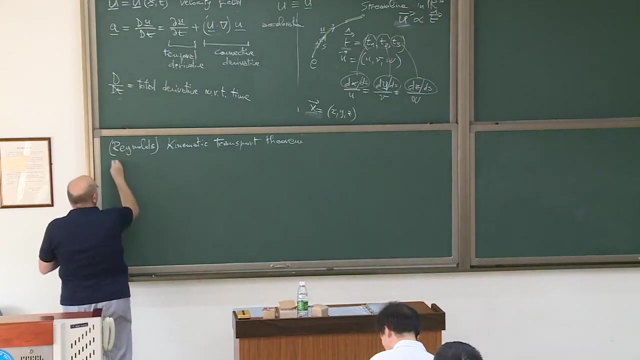 and the theorem. I want to to give a little proof of this because it's so fundamental. so let me is based on is a development of Leibnitz rule, so it's not so extraordinarily unrelated with the typical integration. so the theorem says the following: let 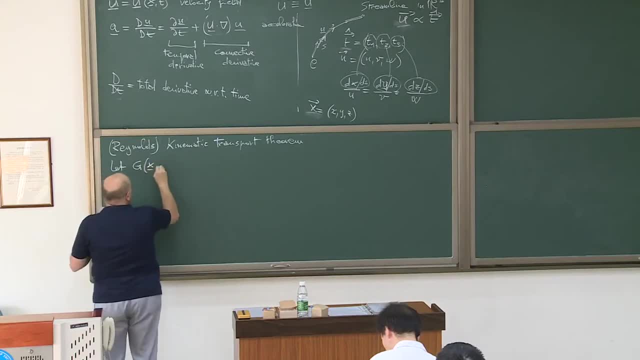 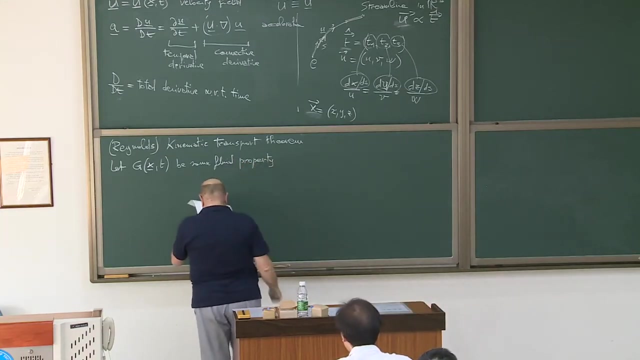 g, a certain quantity function of space and time- we are in R3, of course- be some fluid property, unspecified for the moment, and we take it per unit volume. then the standard derivative d, dt of this quantity, g of x and t in d3 x. sorry, you follow me if I keep using. 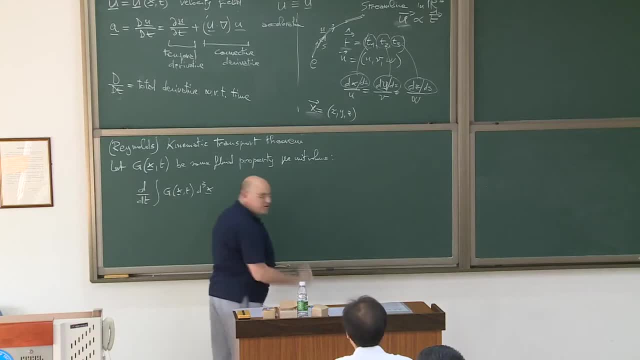 this. otherwise I tend to- I tend- to confuse myself continuously. well, for instance, it's not so necessary at the moment. I just want to show you that what we are going to do is that this derivative enters here and we have a partial derivative, dg dt over the volume. 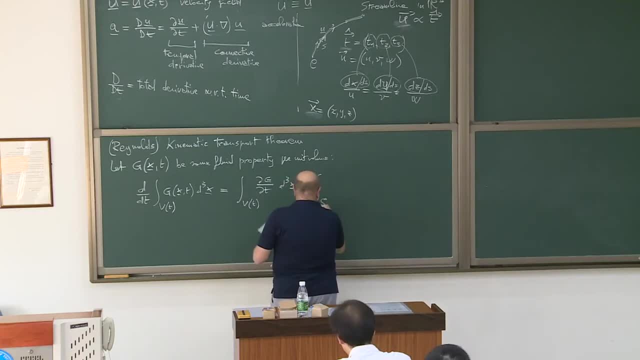 d3, x plus the surface at t of this volume, g times. of course. this is always the same. g times say w. w is like a velocity at the moment I'm not thinking exactly as a fluid velocity, u. that's why I use a different letter. it's just a theorem of kinematics. 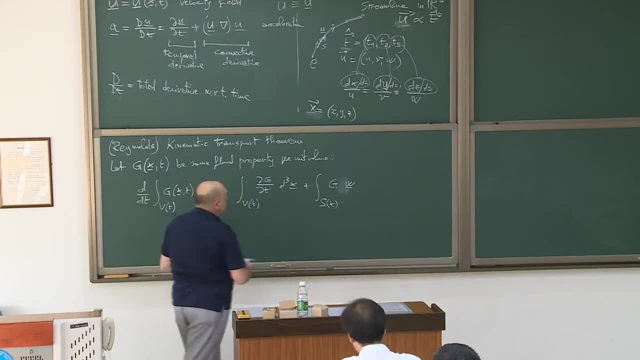 of mathematics, it's not of physics. I will apply it to physics in a moment. some velocity v, unit vector nu, d2 x. okay, so this: I will give you a little proof of this because we need this and after this proof we can move quickly on applications. 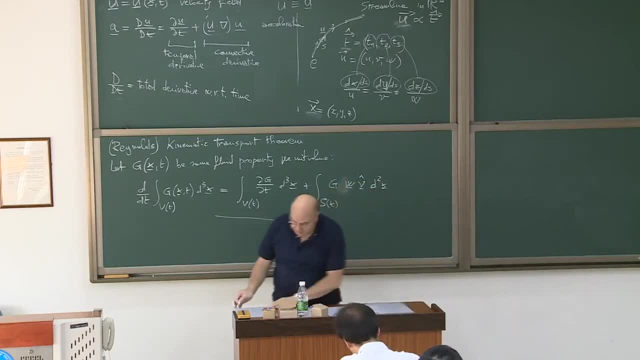 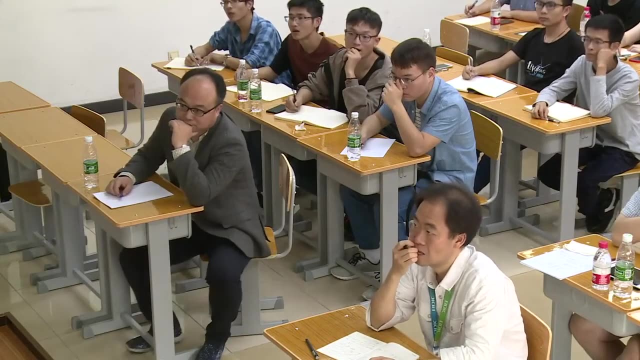 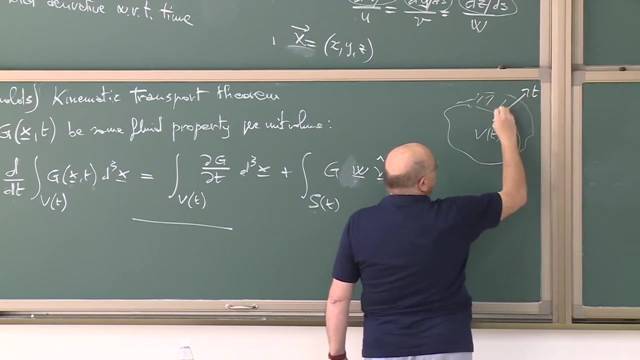 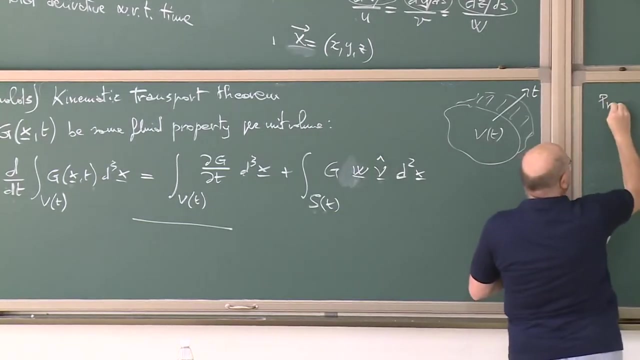 so the proof of this is just rather elementary. and you have to consider the volume, and this volume is a function of time. it changes, and as time changes t, then there is a new surface that is formed at time, t plus dt. so the proof of this is rather simple. 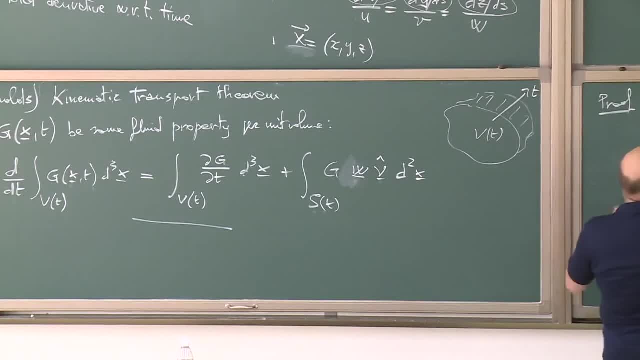 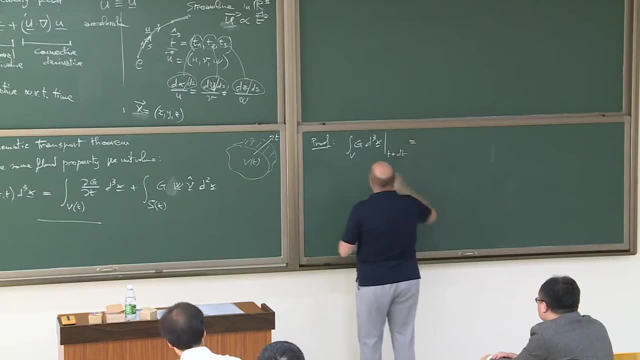 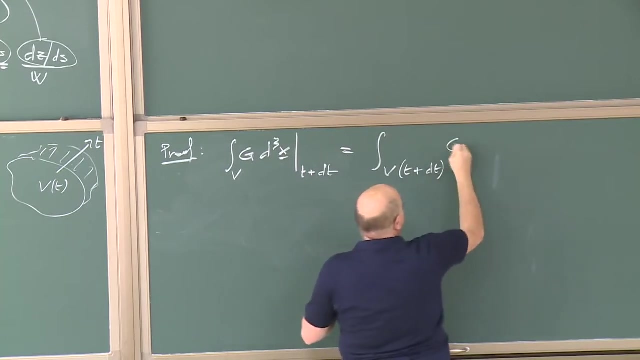 you have the integral of g v on d3, x and this is, at time, t plus dt. okay, because we want to construct the differential dt working on this system. so we have the integral on the volume that has now changed, t plus dt of this g. that is now. 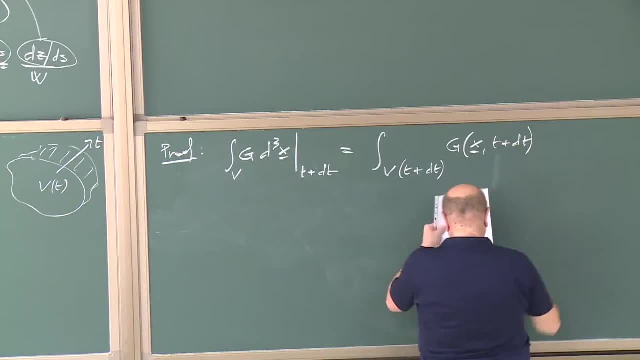 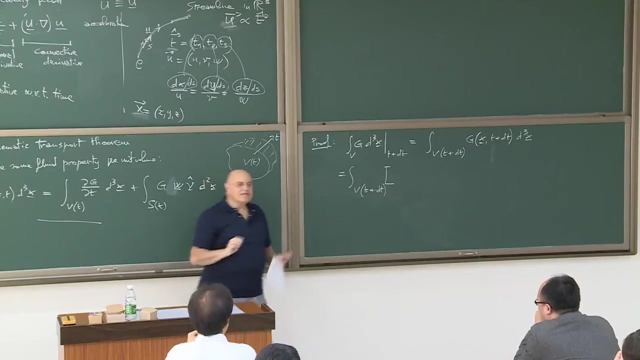 x and t plus dt in d3 x, and this is the integral of vt plus dt, of what well? we expand, Taylor expansion. as normal folks, everybody does this. we Taylor expand. this is the first, very first time that I have to stop, slow down and tell you: remember, we Taylor. 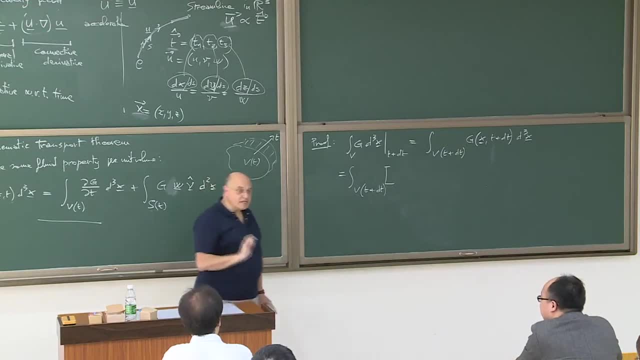 expand. we assume that we can Taylor expand. always remember that problem of singularities, etc. etc. you see how creeps in in the fundamentals of what we are doing. we just started few minutes and we already noticed that we expand. we will have a tool. we use this tool. 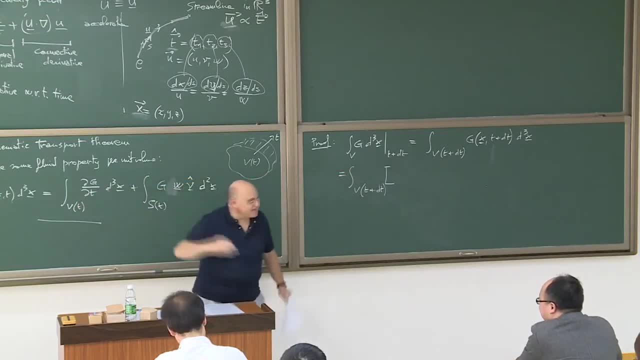 everything is fine: books and books, and books. but if here we have a problem because there is a singularity, somewhere, immediately we have a problem of the foundations in the tools we are going to use for the rest of the course. okay, so we Taylor expand that, and this is: 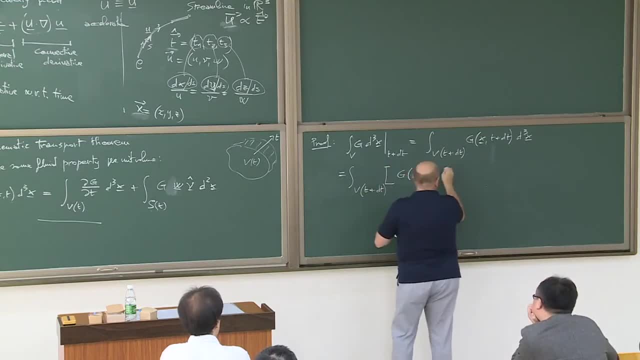 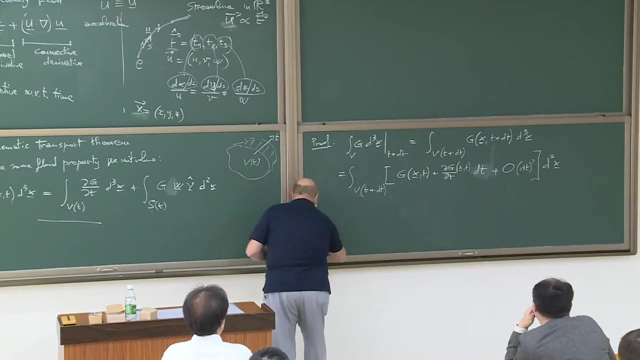 g of x, t plus dg, dt, xt, xt plus. well, we can, dt, sorry, dt plus an order of magnitude of this, dt squared, okay, something like this: and this is d3x. now we need, we need to evaluate this integral and so the v at time, t plus dt. 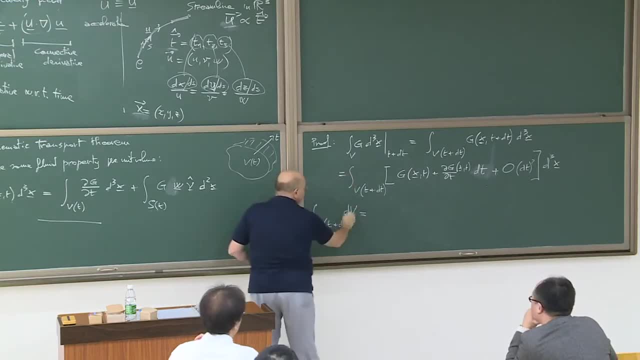 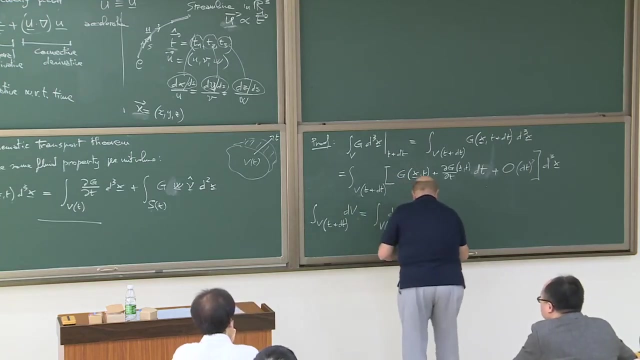 is so this I will call it just the volume, just to focus on this part. and this is just the integral on dv of v of t, plus the contribution, the variation of v, t in dv. and this is just the integral on dv of v of t plus. 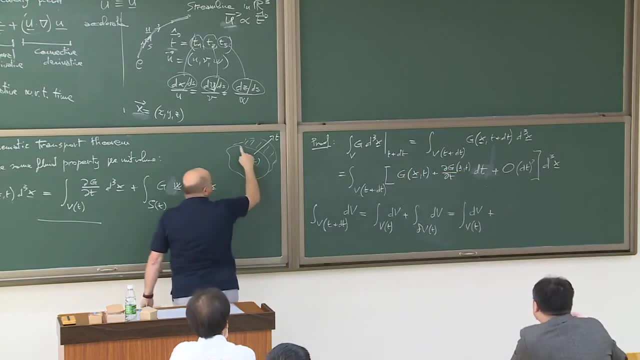 now, this variation, the variation of the volume, is due to the variation of the surface, and so we have to take into account the surface contribution. so we have s of t, and this is just some velocity v, not necessarily the fluid velocity, because the volume may deform due to some other reason. 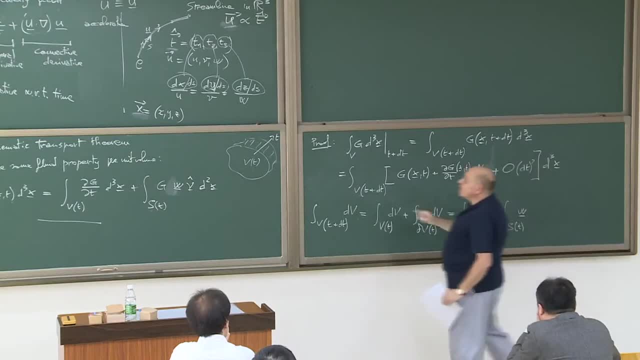 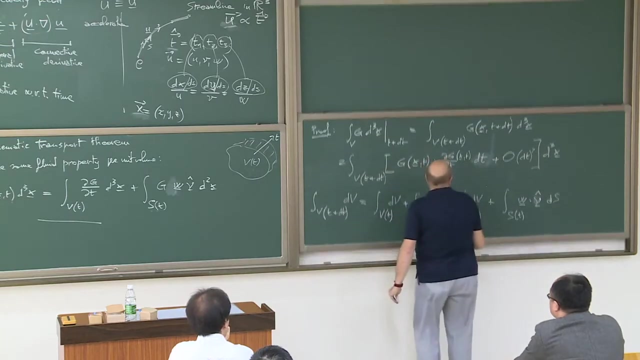 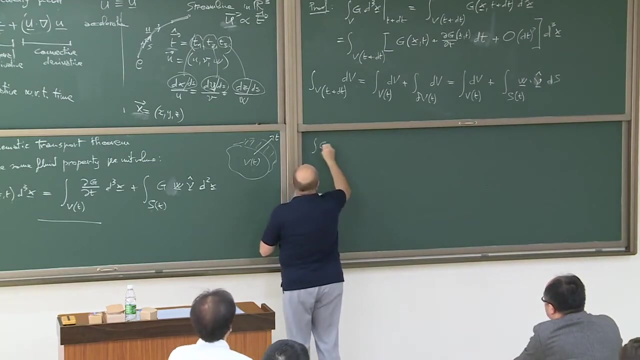 so v, which acts on the unit vector that I assume is pointing outwardly. so let's say d2 um, ok, and this is d2 ds, ok. so we put all this together now. so we have integral of g over the volume, v, x and t in d3x. 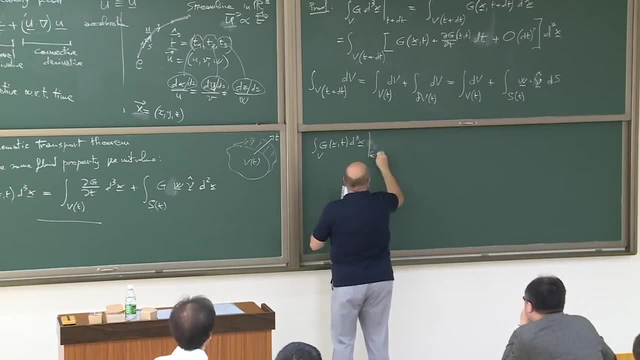 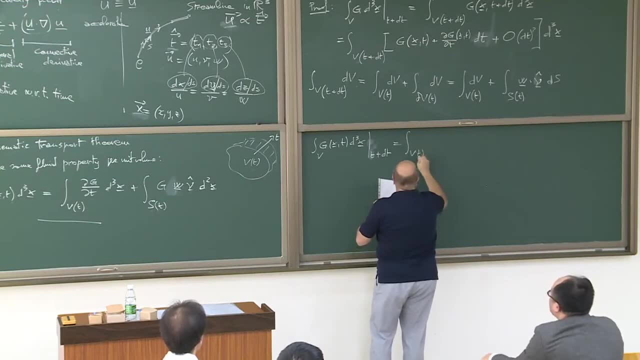 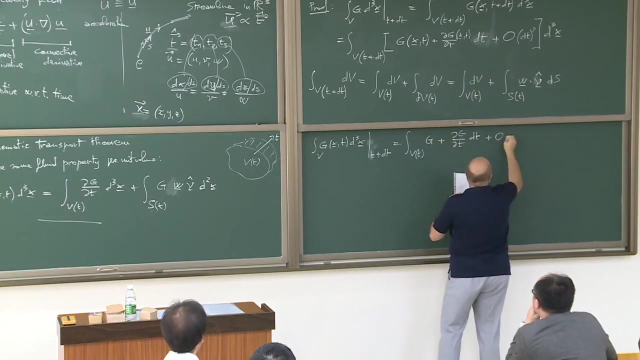 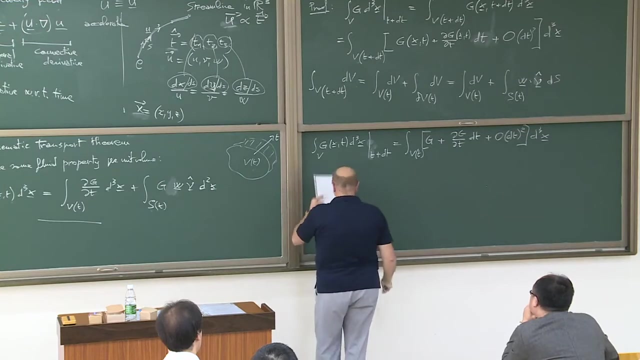 this becomes. this is at t plus dt. this is the integral dt of again the Taylor expansion we used before. let me write it as g plus dg, dt in dt plus the order dt squared. and this was on d3x, not yet it will. yeah, ok, and then we have what. 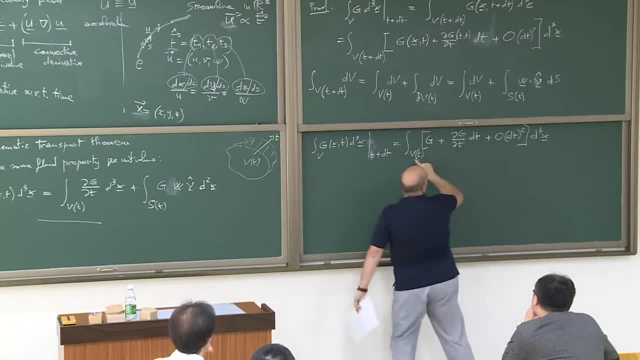 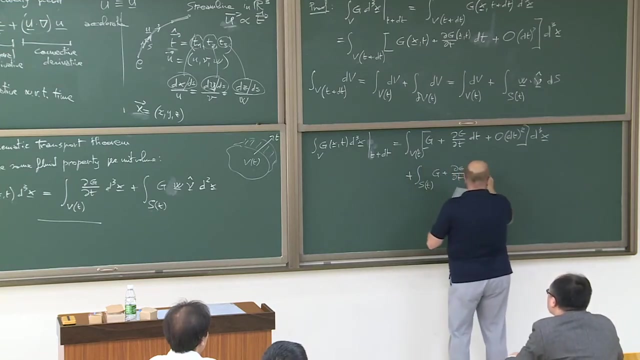 we have. this is on v, and then we have to move on on s, so we have plus integral s of t dg plus dg dt in dt, plus the order dt squared, and this is d3x, and now we can conclude integral over v of t g. 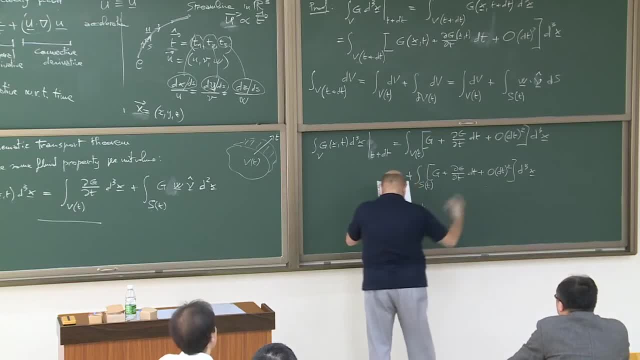 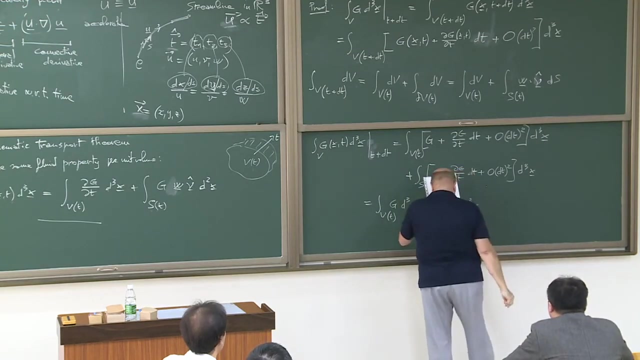 plus, plus the higher term contribution, dg, dt, dg, dt in d3x, plus the surface s t, g times w, dot, nu. I will emphasize, I will put it in this form over there. and this is ds, just to keep this differently. and this is dt plus an order, dt squared. 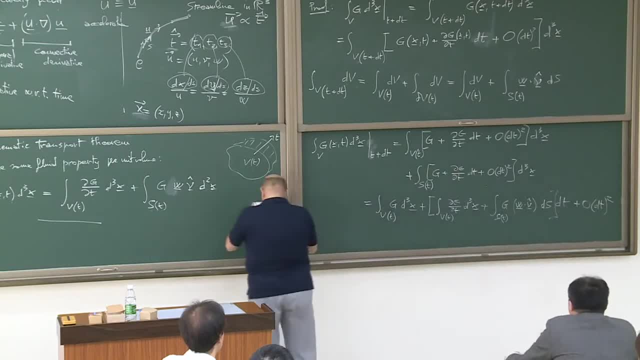 you know what I'm going to do. I'm just taking the limit. so I'm taking the limit, I have t, I have v at t dt and then I'm doing minus the v at t, as delta t goes to zero. so we have the following d dt of: 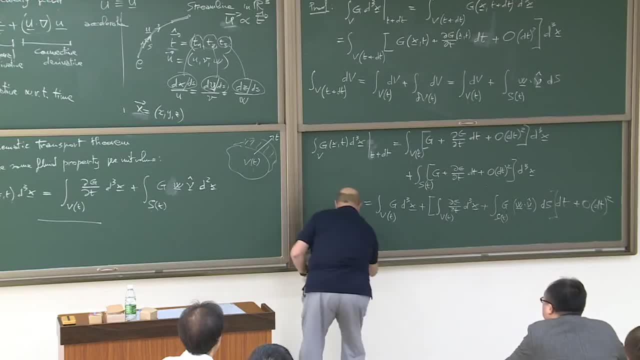 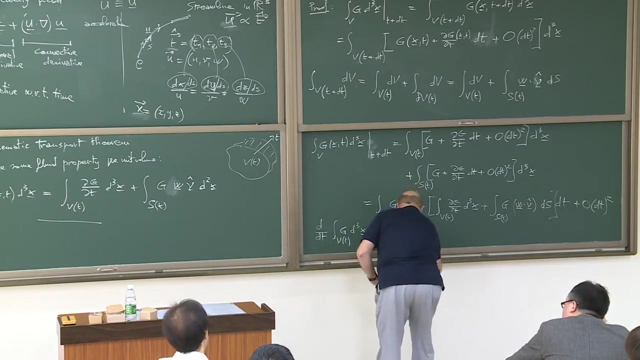 integral of g exactly the statement d3x over v of t. this is the limit, as delta t goes to zero of one over delta t of that difference, and that difference is the integral on v of g, d3x minus this, calculated at t plus delta t. 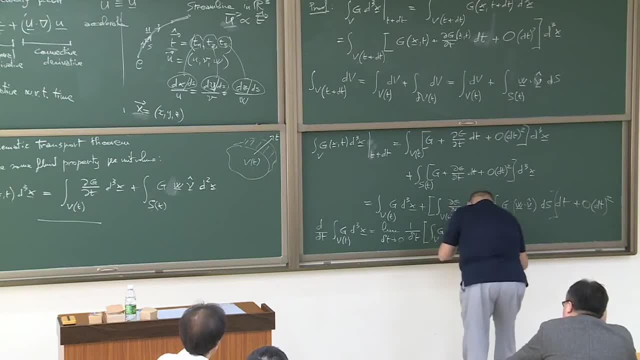 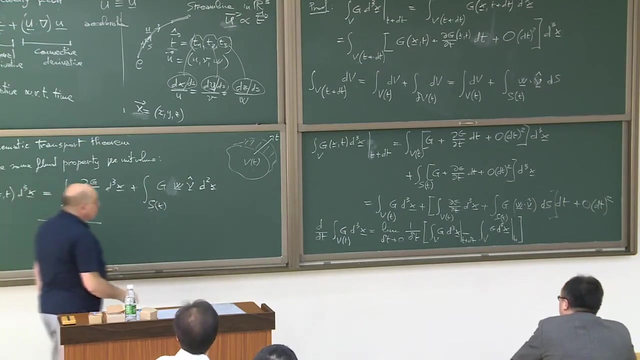 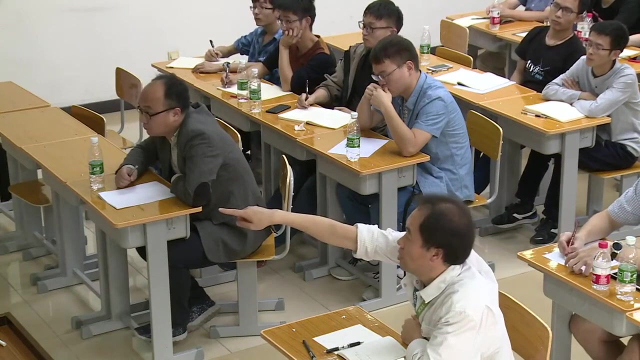 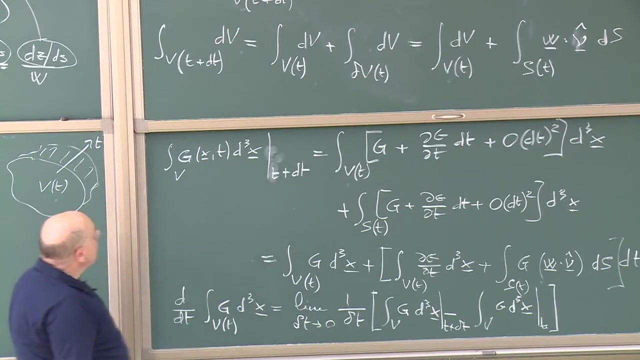 minus the integral on v of g, d3x. okay, and this is calculated at t. so we proved. so we proved this statement, we proved this statement. so the second second line of that, this one, that one comes from the last term, yes, this comes from here, this part here, 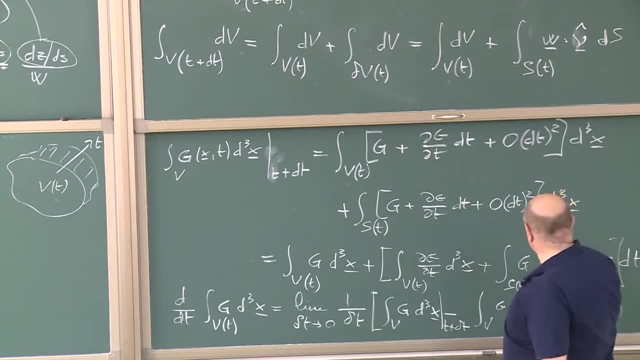 comes from here. this part here is just is just, I'm grouping up g. sorry, I'm grouping up dg dt here and g in ds, if I'm correct. let me see if I might have escaped. sorry, I lost on the notes what I've done. okay, here and this: 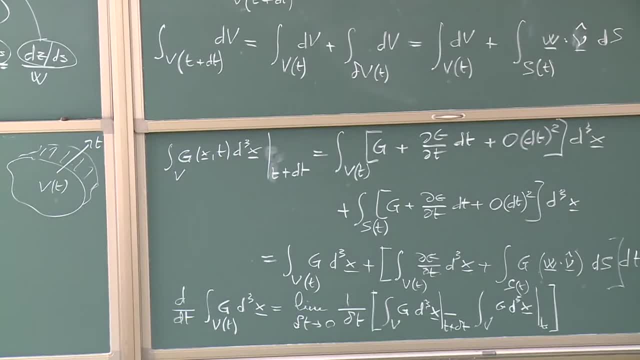 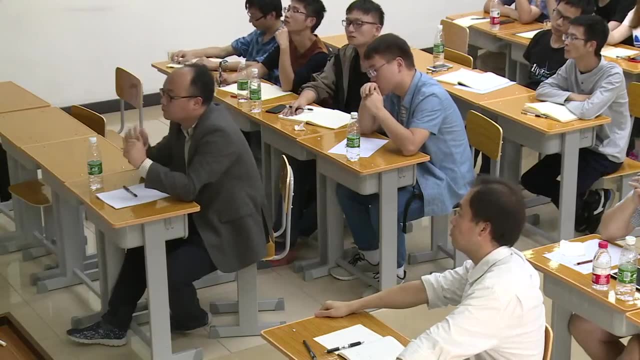 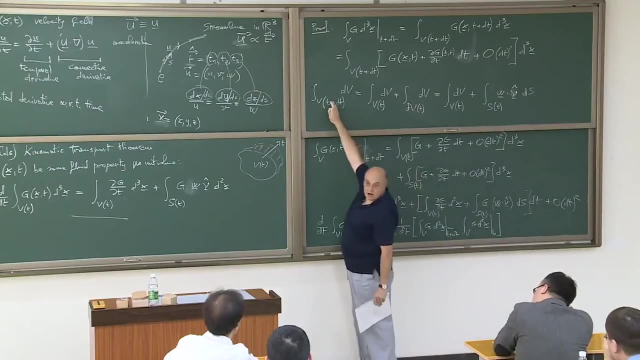 in dt plus the rest. yes, so that means for w dot v hat. yeah, it is an argument of g. yes, yes, this is. I omitted here all the expansion. yeah, I just showed that that part is due to the movement of the surface, because the volume changes and then 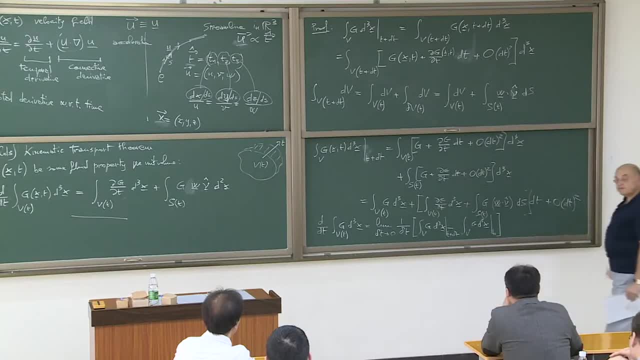 I apply this argument to the g expansion, omitting I order terms, because this is a d2, ds is a d2x in dt, so it's I order and I I order. so in your theorem here it should be w dot v hat. oh sure, sorry. 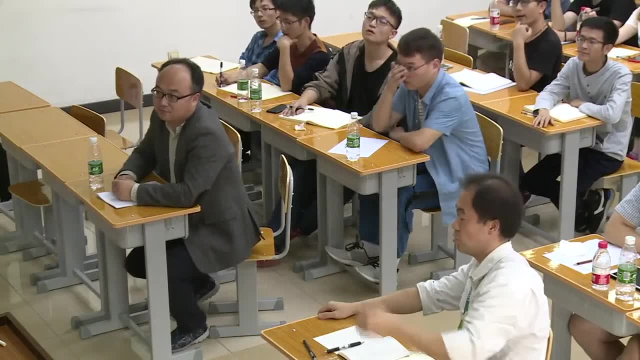 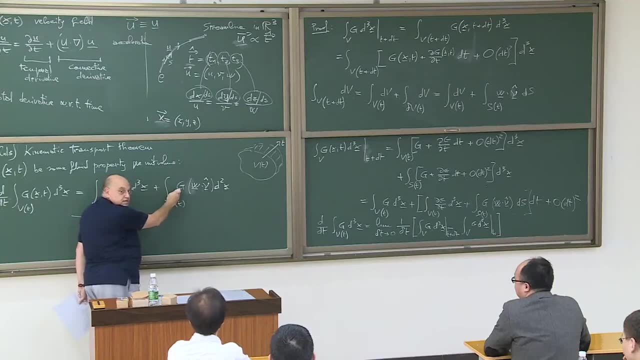 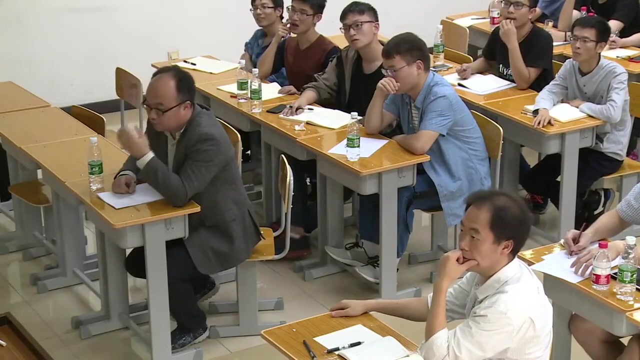 yeah and yes, yes, ah, no, no, no, no, no. this is just the product of g times, the scalar product of v nu. what's the w here? w is some is arbitrary at the moment it will be. velocity field at the moment is just a field that makes. 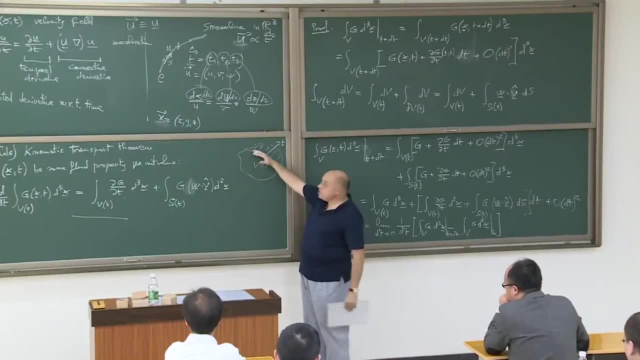 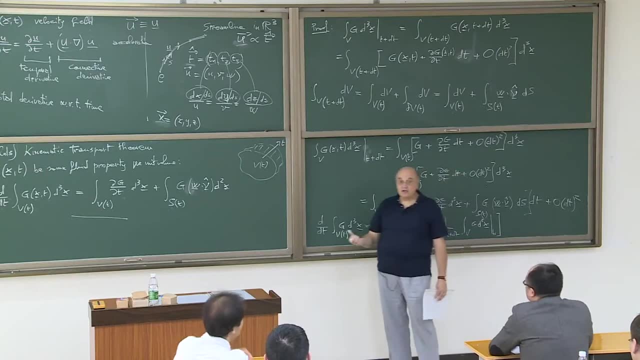 makes the volume changes. so imagine that the volume is subject to motion that is not necessarily coinciding with the fluid motion. you may have a fluid that behaves, suppose is charged. then particles go in one direction and the fluid goes in the other. the fluid has a velocity, u, and the particles 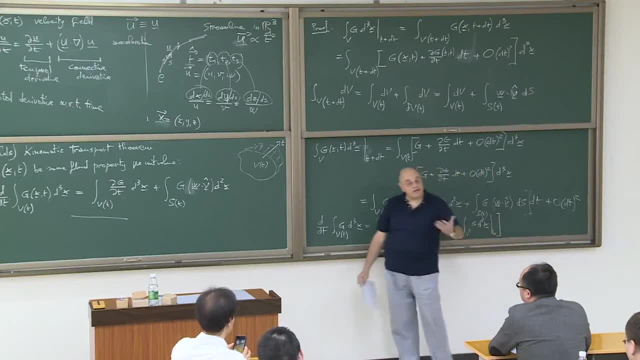 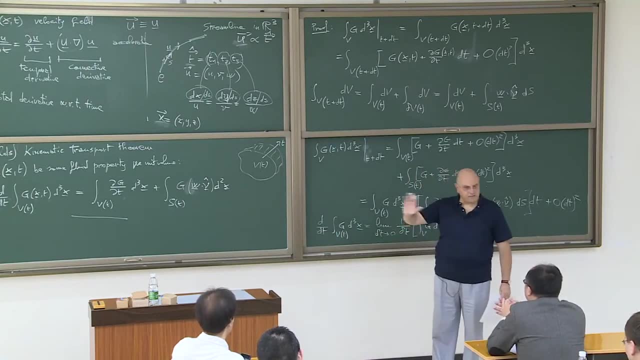 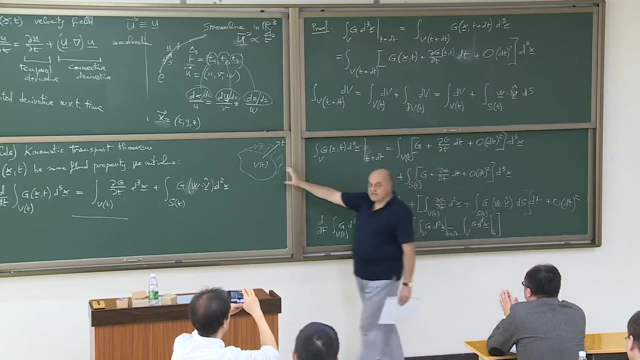 may charge, may react to some electric field or magnetic field. so for the moment, for the moment is just a vector field. then, for simplicity, we identify this vector field with u. I can do it instantly, in a moment, and then you give a sense of this change of volume. 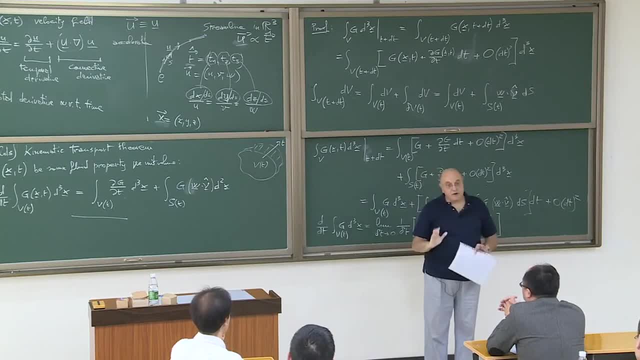 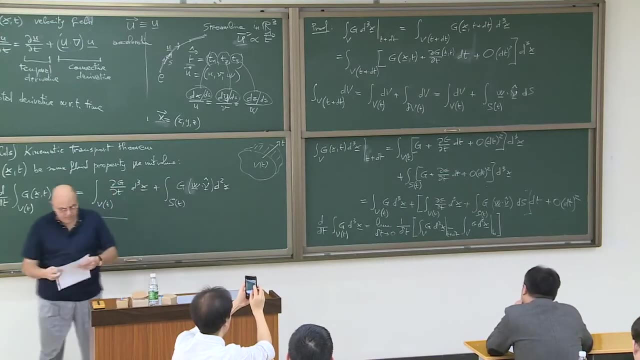 due to the motion of the fluid, a fluid that is not electrically conducting. I'm not considering magnetic fields, I'm not considering electric fields, I'm just considering neutrally charged, if you like, neutral fluid. ok, let me remind you. well, if you take this theorem and 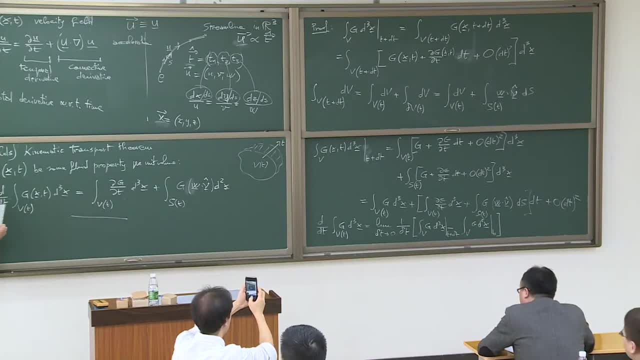 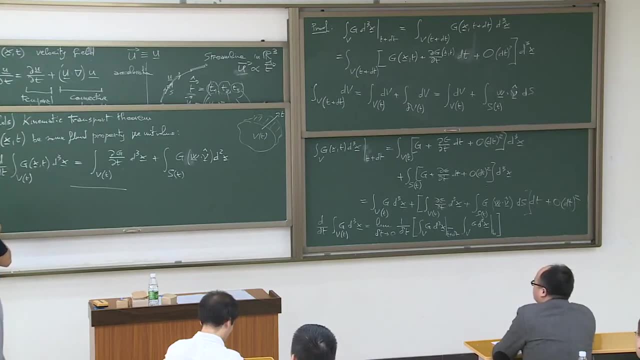 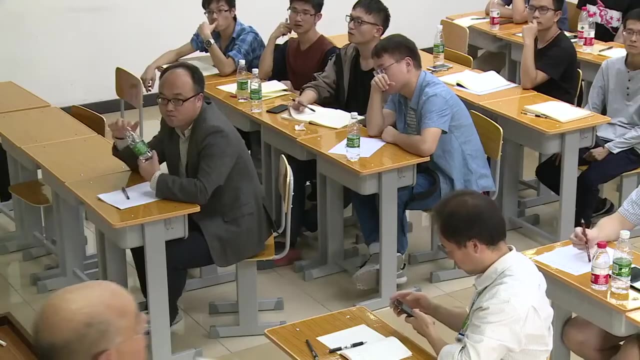 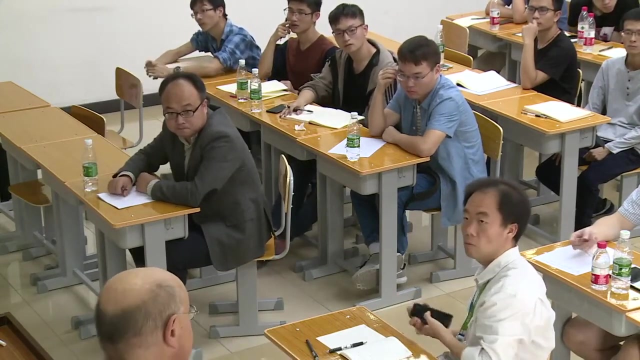 you consider. I want to leave it there and I want to just give you the idea that you may now consider v as a material volume. ok, a material volume meaning in fluid mechanics a volume made by the same particles all the time. imagine that you color. you color with ink. 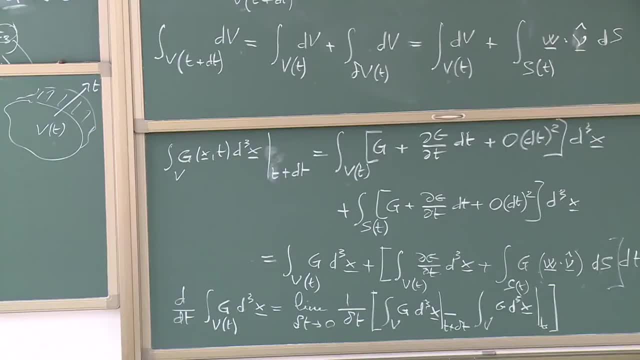 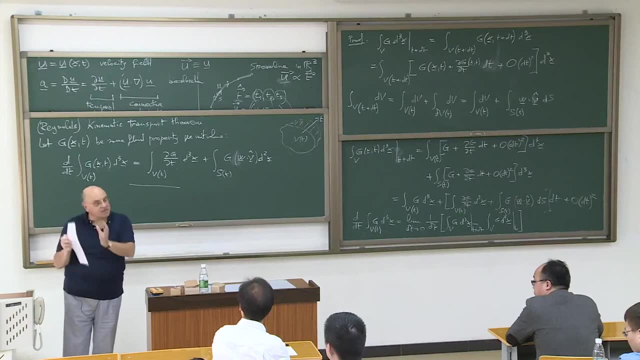 this particle or this particle are like coffee powder, then they remain the same in the volume. the volume is a material volume, so that these particles that have certain property, for example, are colored by blue, they remain always the same with the same blue. this concept is very important and useful. 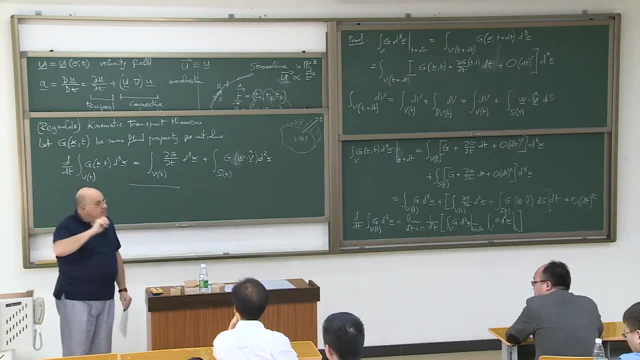 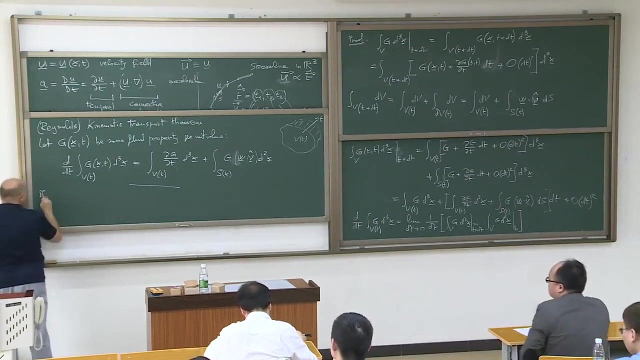 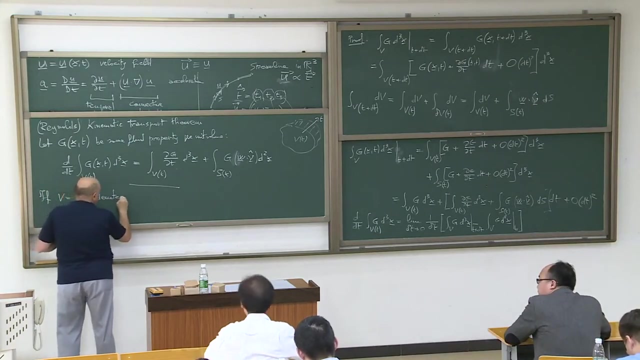 because we will talk about field lines that remain, with the property of being streamline, of being vortex line, of being magnetic lines, forever made as material lines, but the same properties all the time. so if, if v, v of t denotes material volume, material volume, then of course we can extend this. 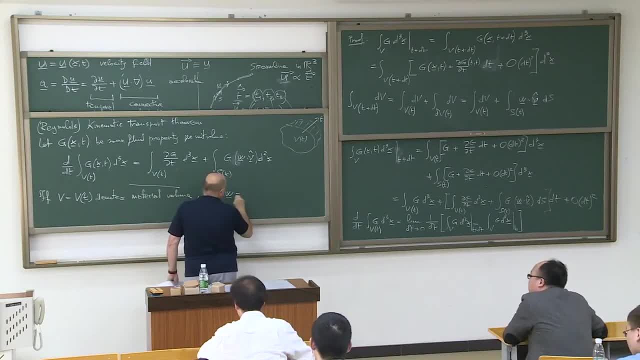 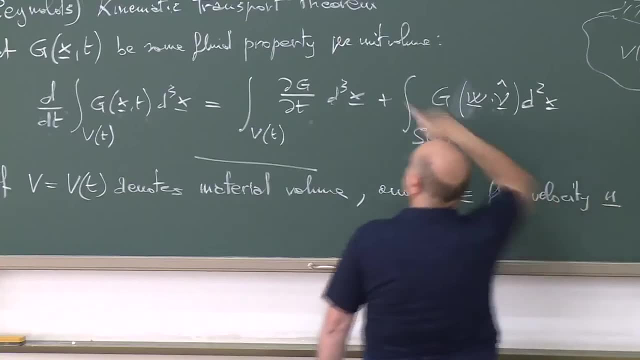 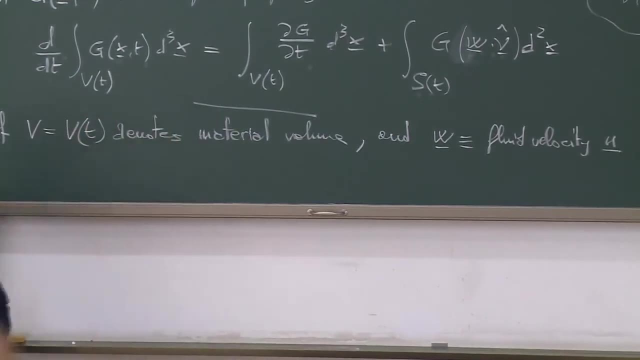 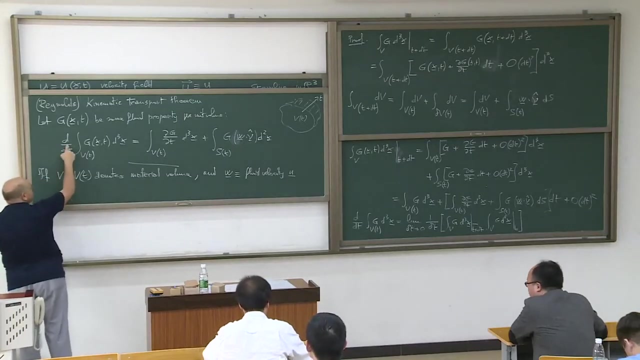 and v coincides with the fluid velocity u, as I give it before, then this immediately becomes the transport theorem for classical fluid mechanics, where v is a material volume. so we still have the same. now the d dt becomes the d dt, in this case, becomes d dt. 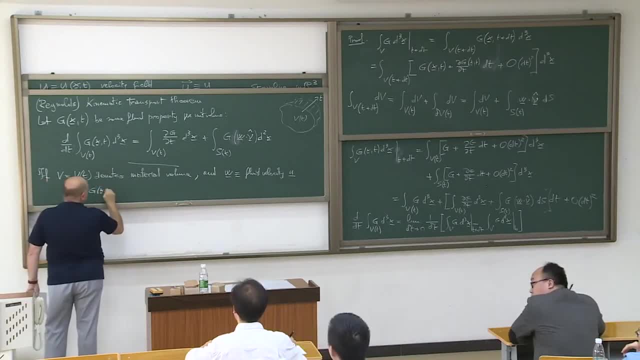 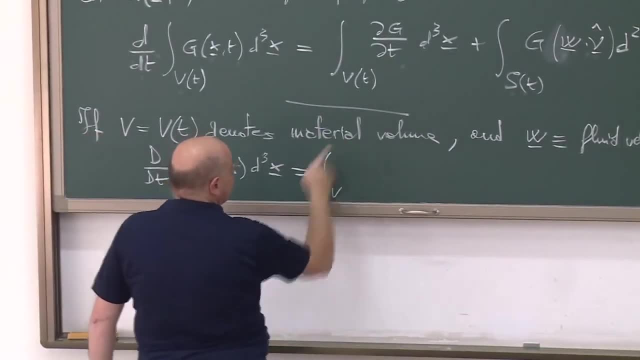 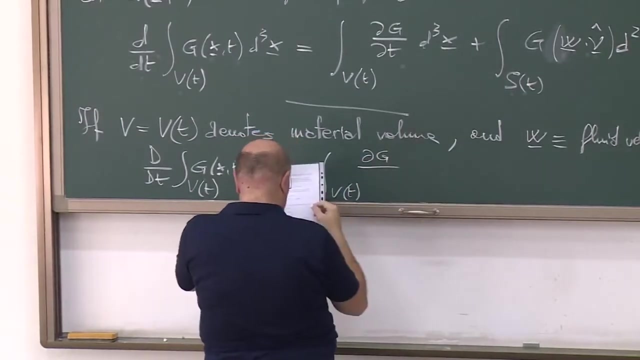 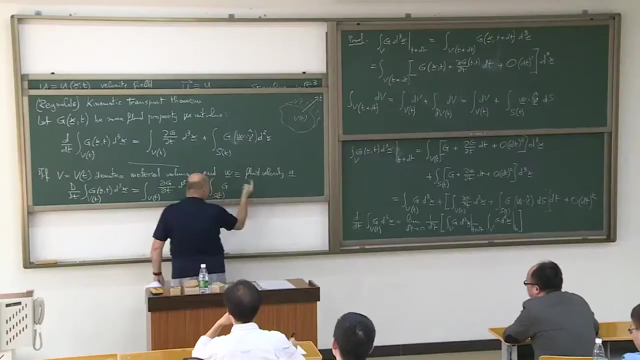 of g, of xt, in d3x volume, vt, and we will almost the same, with this exception of understanding that now u is the velocity field and and v is is a material volume. okay, st, and this is g times, for the moment, is a scalar, still a scalar, but I will show you. 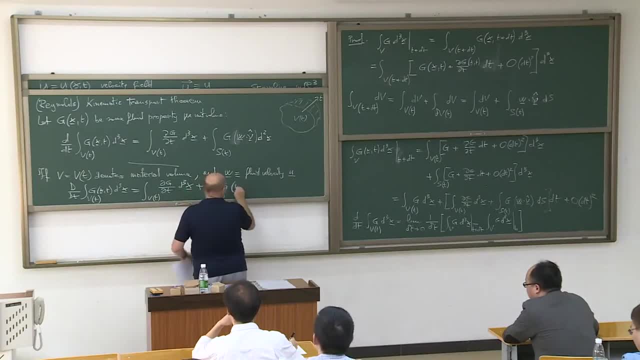 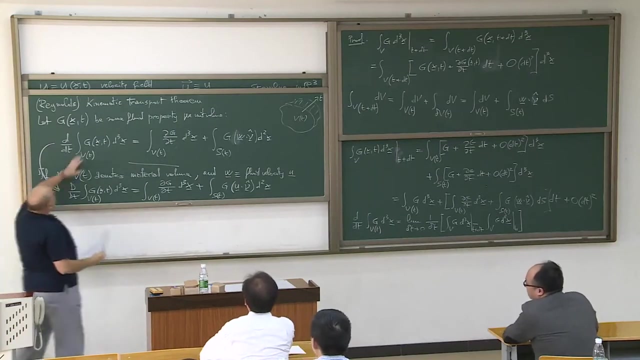 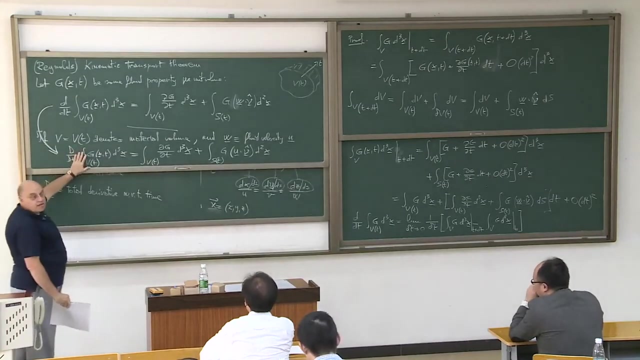 we are going fast now. g of u, dot, nu, d2x. d2x is ds over there, so from here we get to this. so the kinematic transport theorem for fluid mechanics becomes this one, and this one is a very fundamental tool, because you see how it works. 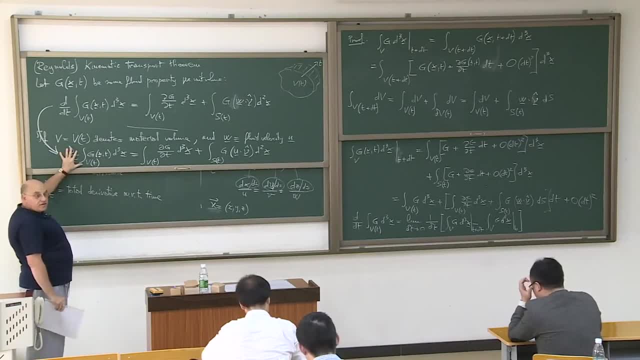 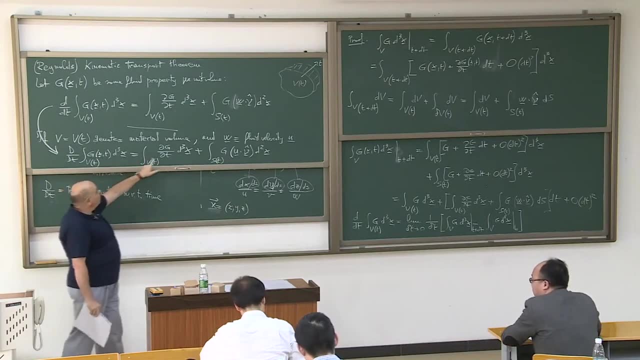 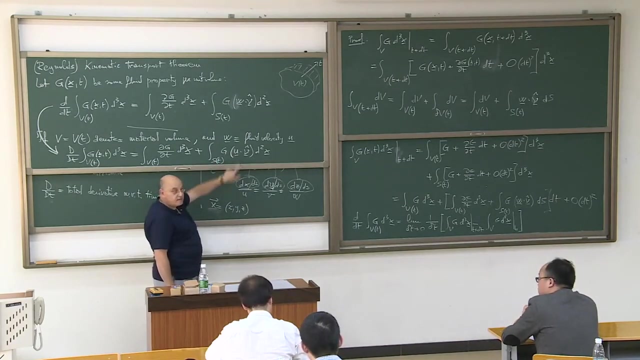 you take the Lagrangian derivative of a quantity under integration and you perform. you are allowed to perform partial derivatives inside. remember, vt is changing but is made by the same particles and these particles are moving according to the velocity u okay. so this tool is fundamental in 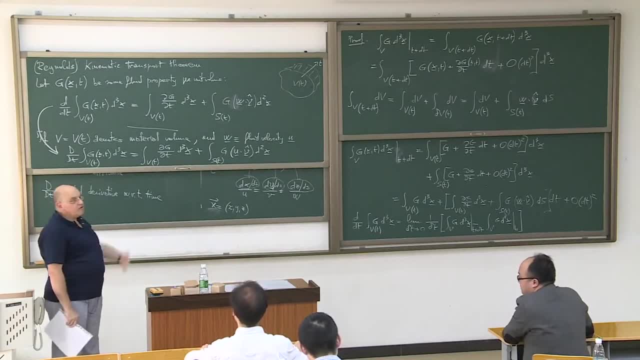 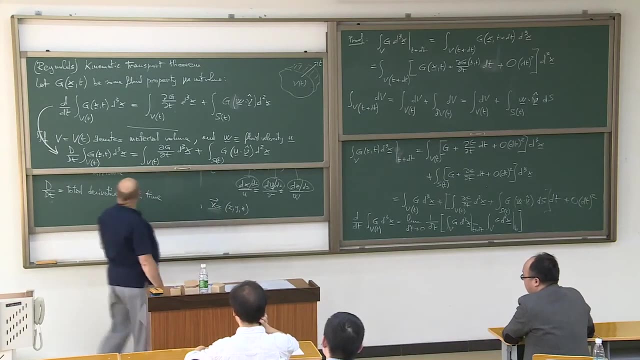 doing many derivations now. I will be quick because this is the hardest point when we are here. now we can use this tool and you will recognize immediately this tool in many derivations, in many derivations. I will use this tool if g is a scalar quantity, as it is now. 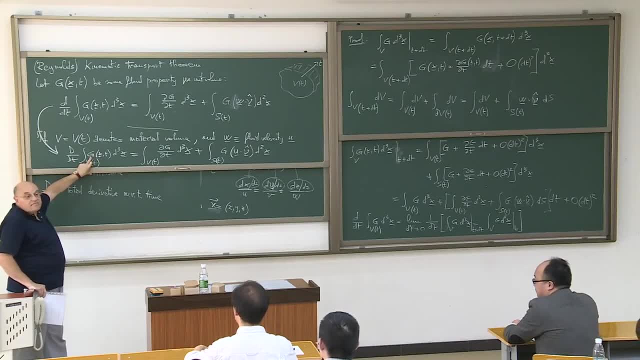 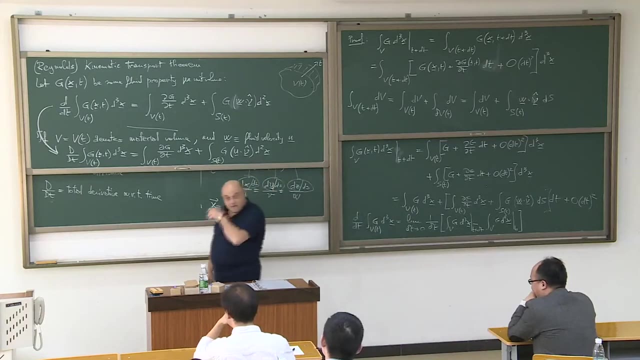 and represent density. we know that mass is conserved and I will apply d dt of this quantity of mass to show that there is no change of mass in fluid and we get the conservation of mass immediately. that is one fundamental equation. we will get to continuity equation. 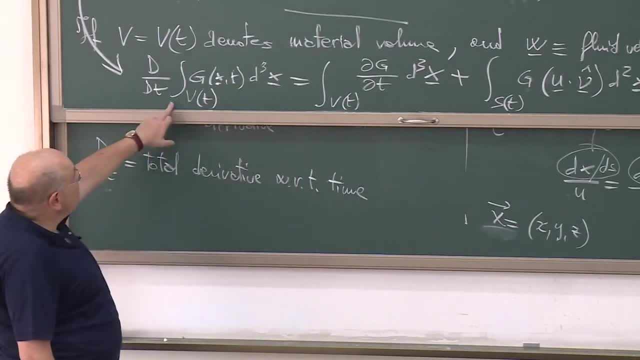 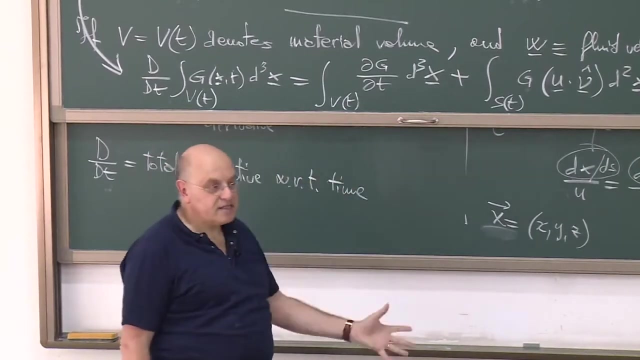 but before doing this, I want to show you. I want to mention, not to show you, but to mention that if I'm not going to do it is trivial, is very simple. imagine that you have a fixed unit vector in space, fixed. okay, you choose a vector in this. 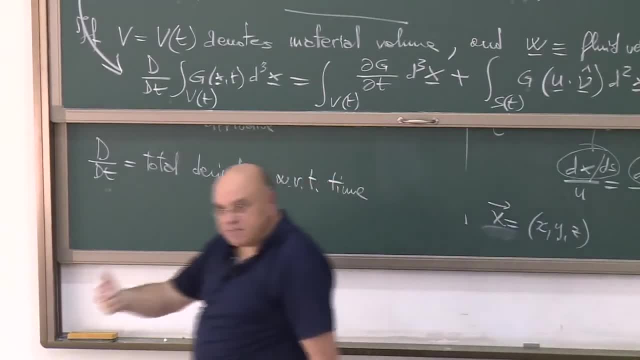 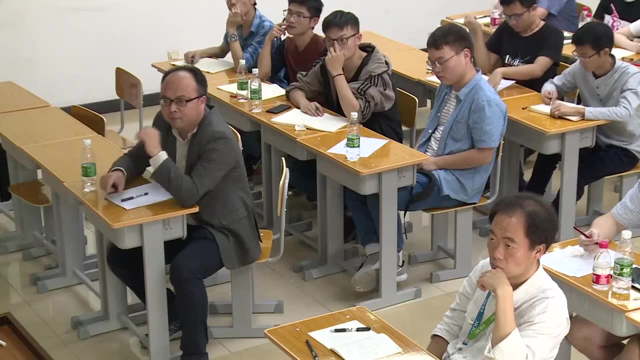 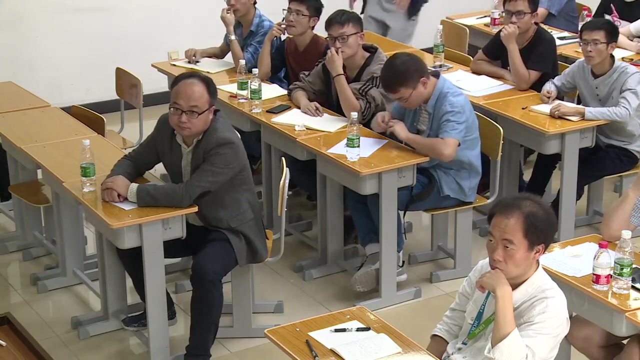 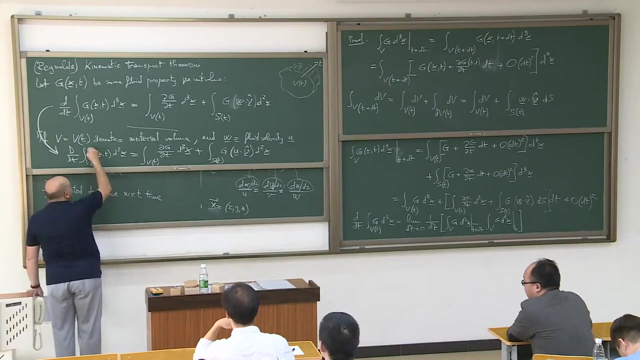 direction of unit length and you multiply this vector through this equation, all through. so you get inside, because it doesn't depend on time is fixed- and you get g times this unit vector. this g times the unit vector, becomes- I'm now moving- becomes this g is a g with the unit vector. 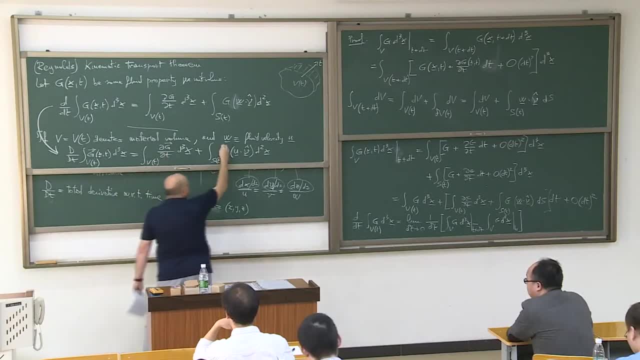 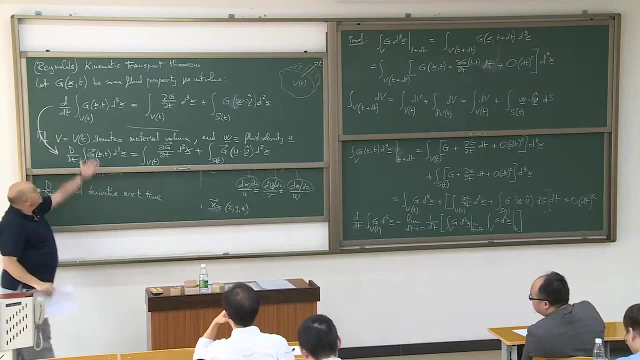 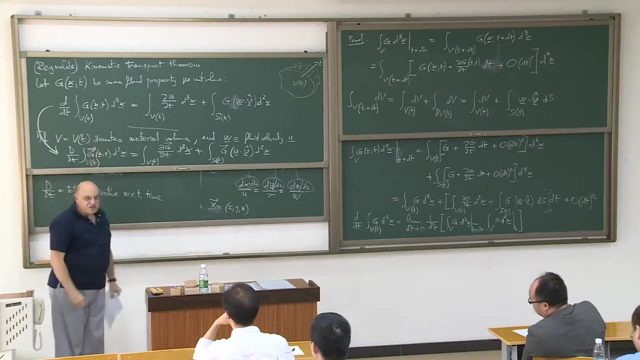 and the unit vector goes inside everything. so you immediately have a theorem after the theorem we had for a scalar quantity. we had also. we have a theorem for a vector quantity, actually even more, if this g we put for fun two hours, two hours is just not standard mathematics. but 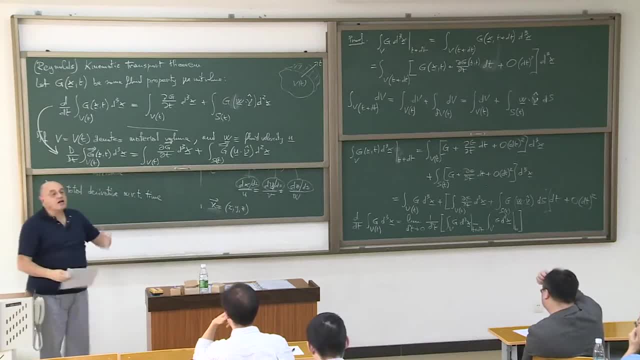 I'm just playing with symbols just to remind you that not only we have the theorem for a scalar, we have a theorem for vectors, we have a theorem for tensors, for tensor quantities is the same thing. why? because we just go through multiplication of something that is fixed. 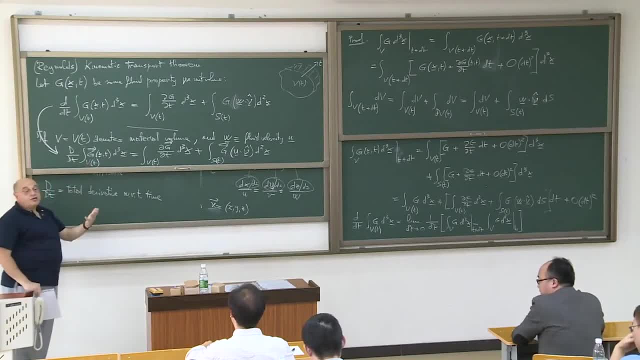 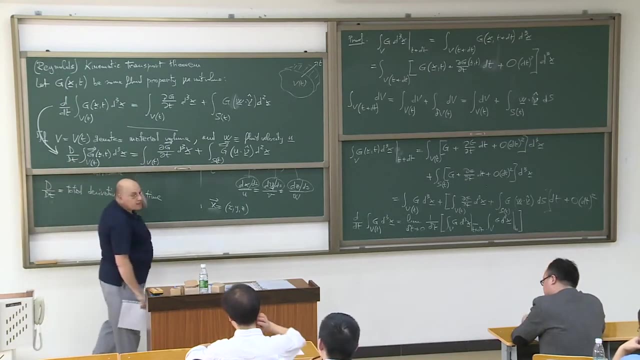 in space and time. so is a way to prove that this theorem holds for any quantity in any dimension. good, this is a starting point. we have a tool to use for a quantity that is either a scalar, a vector or a tensor. now, surely you noticed, here we have a surface integration. 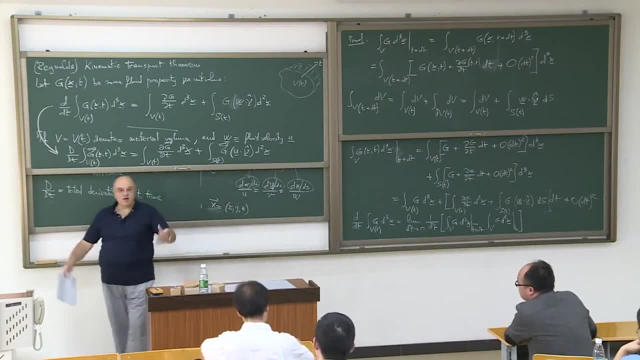 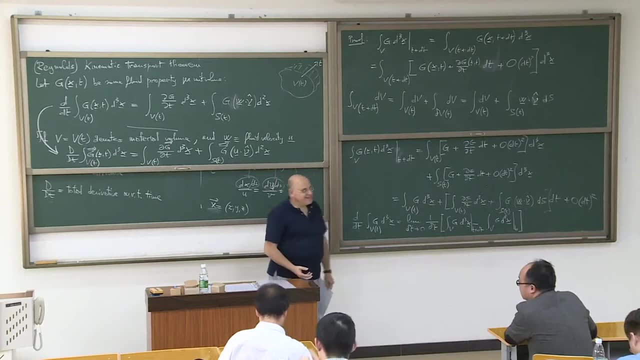 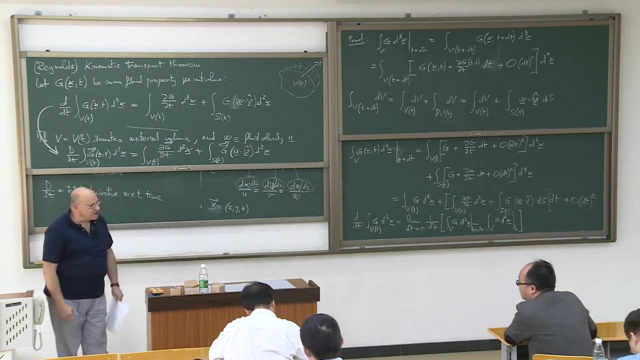 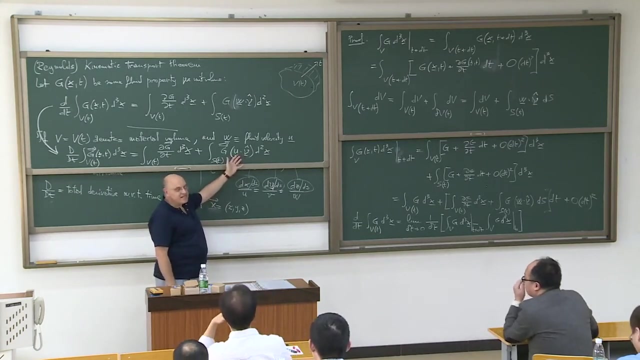 surface integration. come on. one of the first thing you have to remember in standard background education of math for physics is to use what Gauss discovered. we have an integration of a surface, so we have. we can convert this into the divergence right is called the divergence theorem because 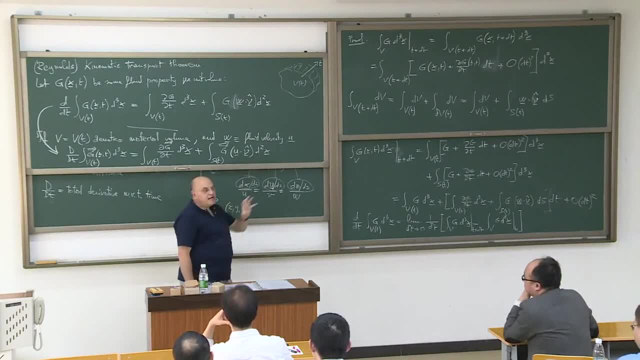 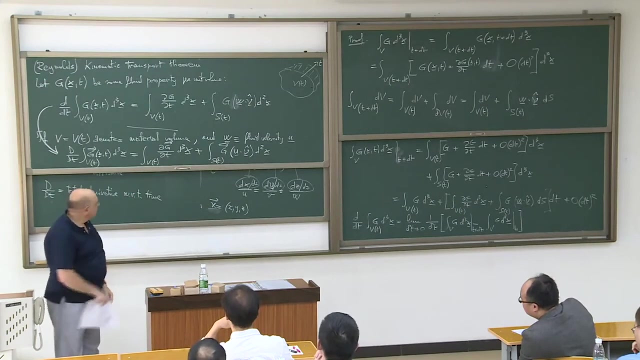 the nu on the surface gives you a direction along which you act. so you have a flux, a flux through the surface, a flux through the surface. and you use divergence theorem so you can convert this surface integral into the divergence equivalent of it. alright, so we do that. 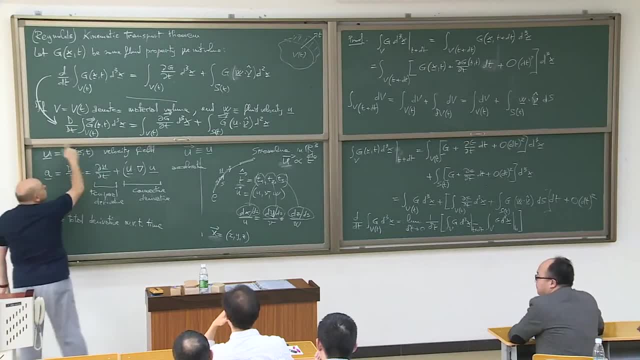 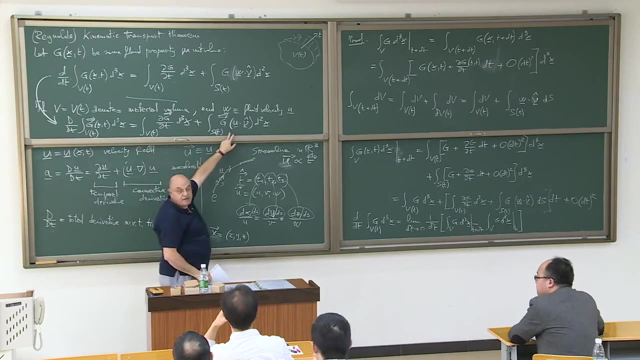 so already you saw quickly, once we got this result, how quickly we can now get this total derivative working on integral quantities, scalar vector tensors. and now we do one further step: we transform this by using divergence theorem and then we are almost done, because we have a tool that is working throughout. 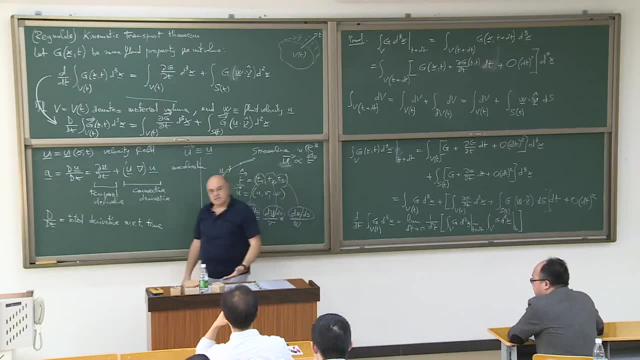 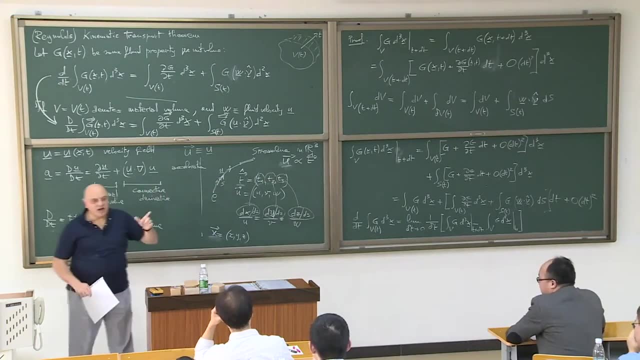 fluid mechanics repeatedly. remember that we had to go through this Taylor expansion at a point. ok, so these two features: one is that there is a little point that is, so to speak, not so worrying, but is worrying if you have a different frame of mind. and the other point is: 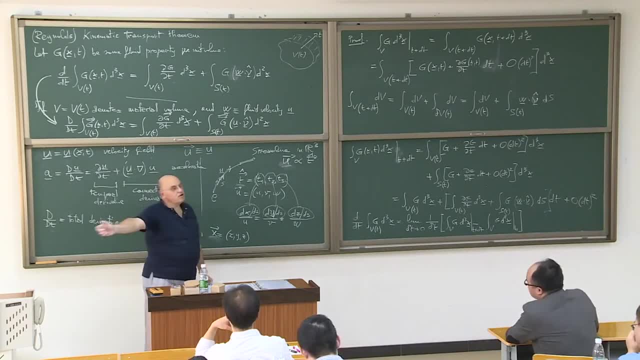 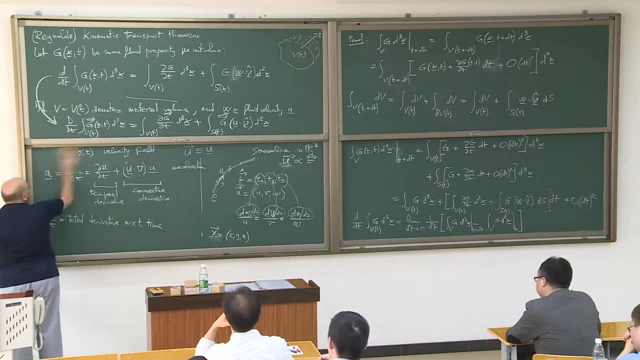 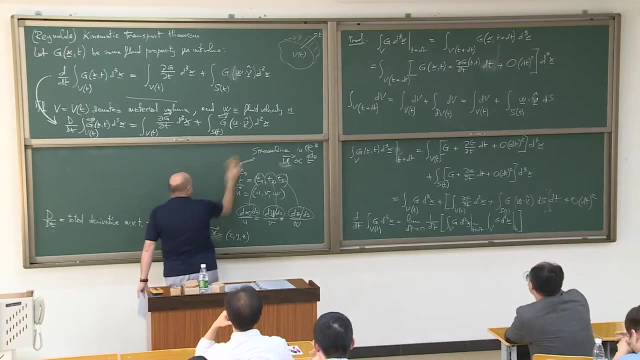 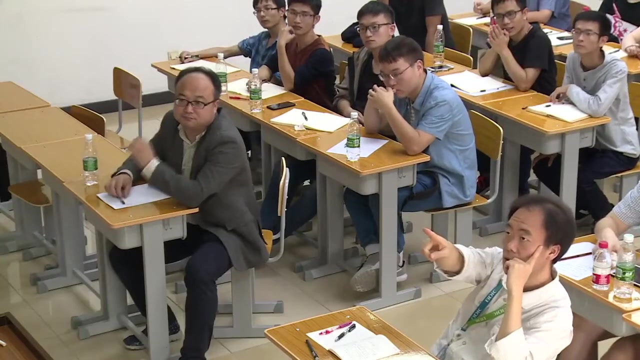 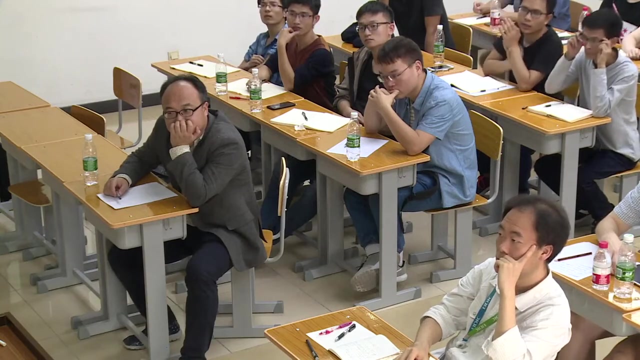 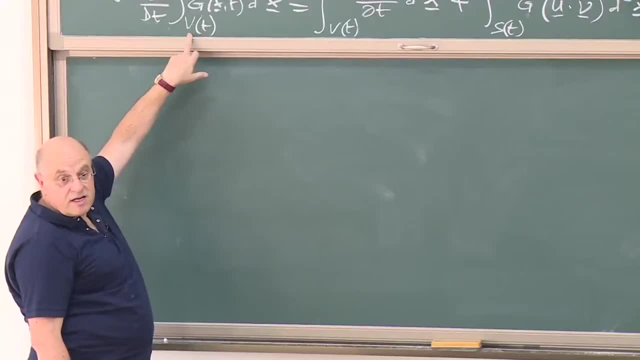 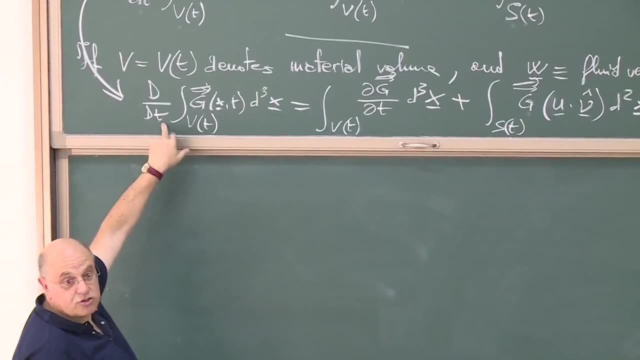 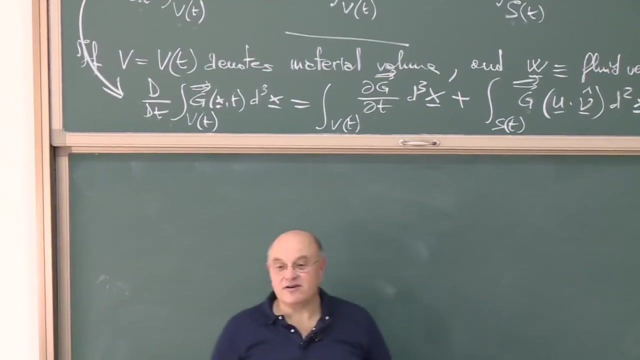 so this is a material volume and so you can convert the standard derivative, the ordinary derivative, with this one. because you consider the Lagrangian, you follow Lagrangianly. I did. I skipped, of course, difference between Eulerian and Lagrangian coordinates, pardon me. 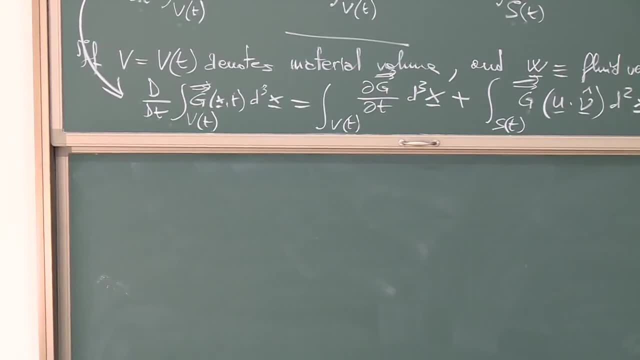 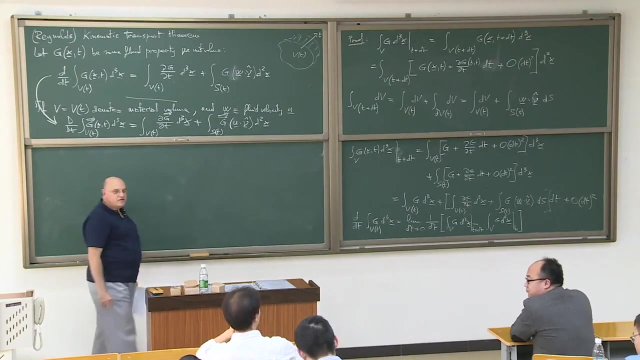 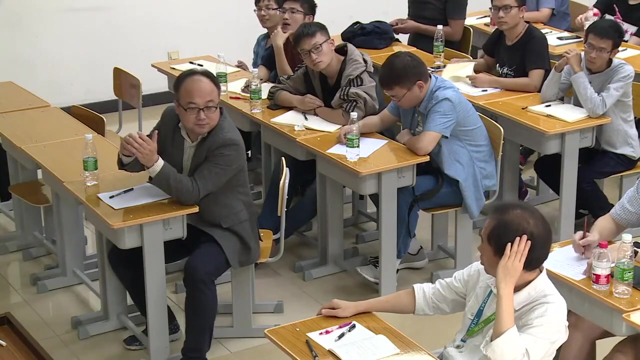 green function. green function, we get to the green function. yeah, because you see the G, no, no, it's not quite there. we get to the green function from the real space to the moment in space. but group of G is also singularity. sure, we will. I, I'm going in that direction. 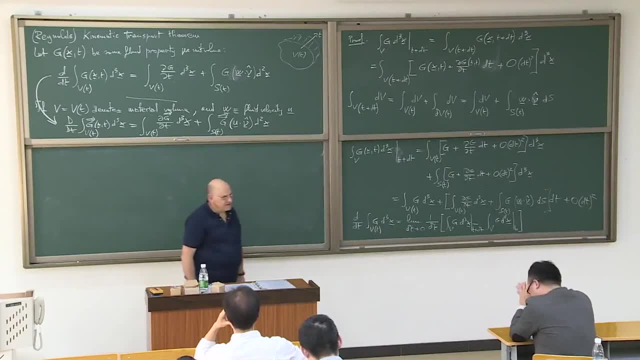 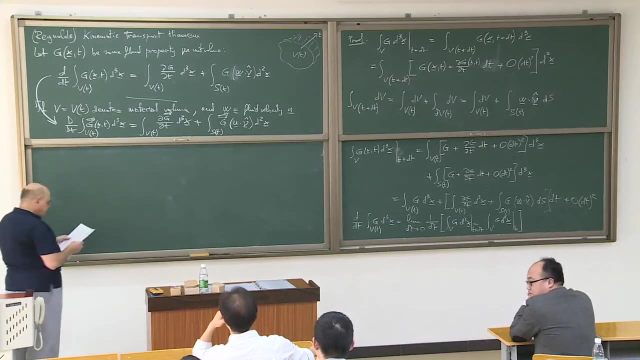 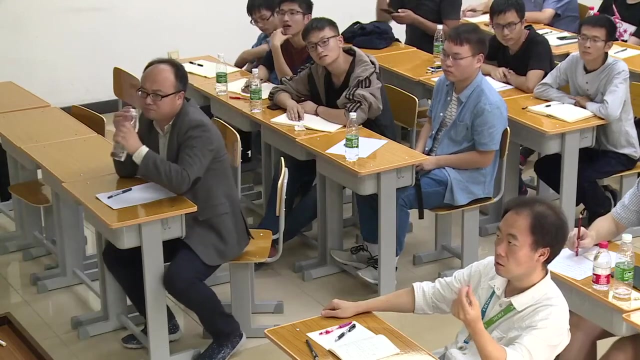 yes, tomorrow, not today. tomorrow will be green function time and singularity time. a little bit alright, so just skip the Lagrangian, the difference between the Lagrangian and Eulerian. ah ok, so this is important, it's a fundamental aspect. ah ok, I had to invent. 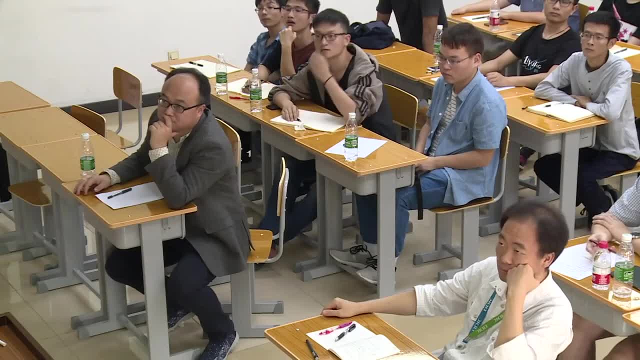 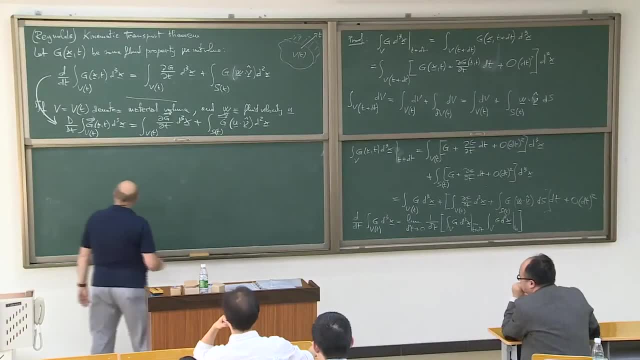 a way to explain this, one way to explain this or to remember this, is the following: suppose, I don't know, suppose you have a river and and you have a boat here and there is a, there is a bridge over this, ok, and there is a bridge and this bridge. 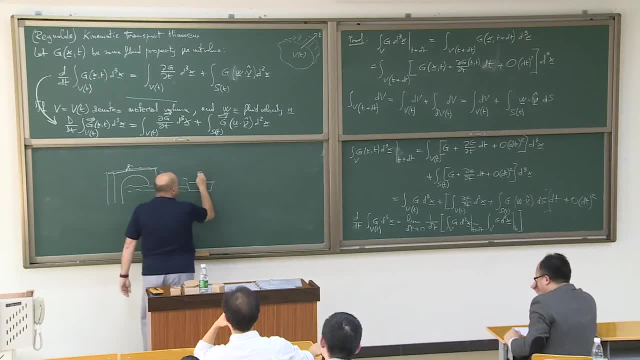 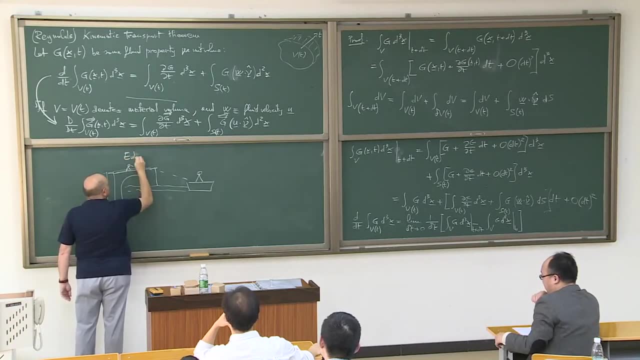 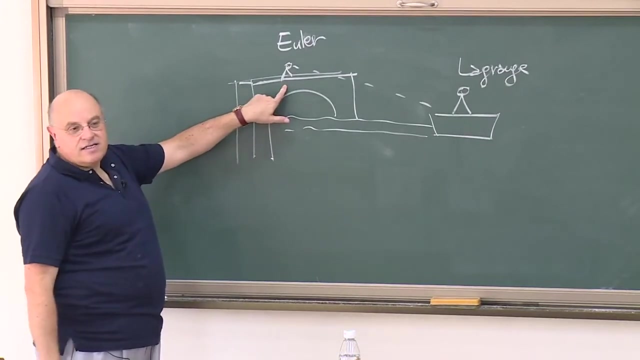 there is a person here looking at the boat and the boat. there is another person there and this person we call it Euler, Euler Lagrange. I hope it works. I don't know, I'm improvising. sometimes it doesn't work. Euler is a. you know, you have WeChat. 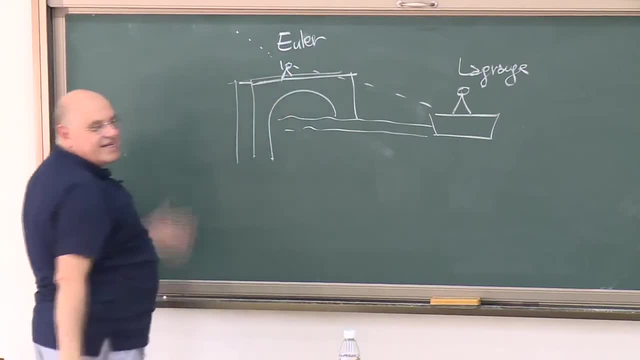 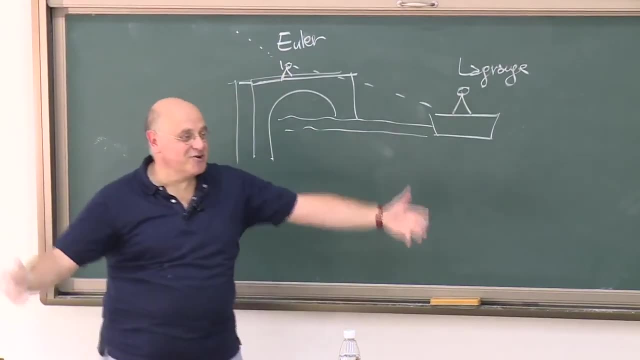 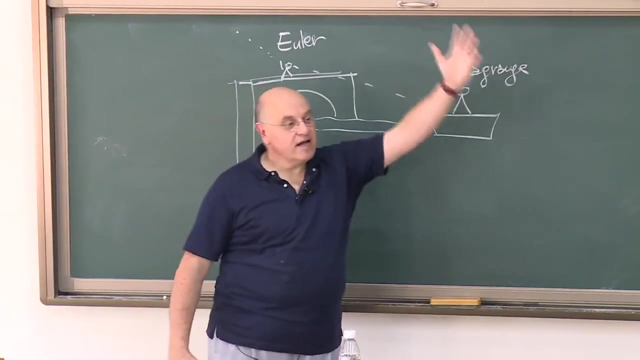 so he is WeChatting, he is sending information to a friend and maybe Lagrange is a beautiful lady. I don't know. he is a beautiful man, who knows what, and Euler wants to say. Lagrange is going away, so he is sending information about Lagrange. 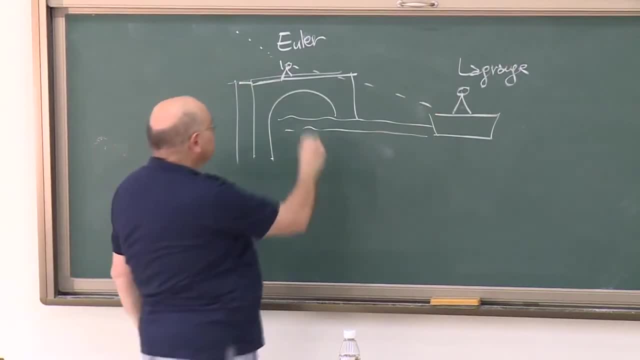 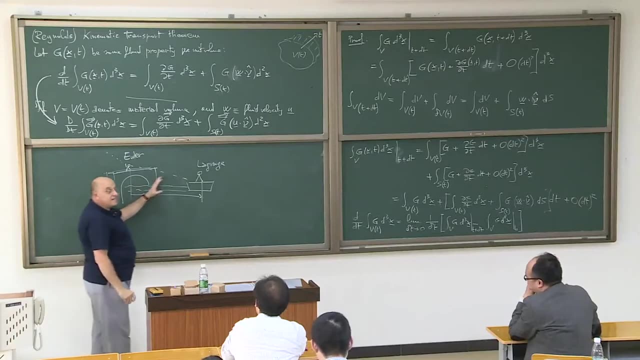 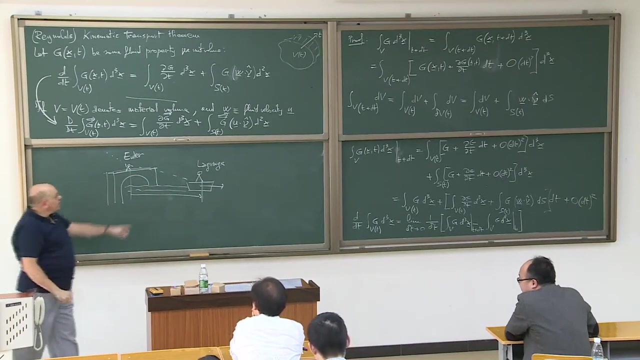 coordinates, coordinates. so the coordinates, this position is the Eulerian position. and as time, suppose the boat goes in this direction as time goes. this is signaling the position of Lagrange. ok, but Lagrange has a different view. Lagrange, you know, moves with the fluid. imagine that Lagrange is not really on a boat. 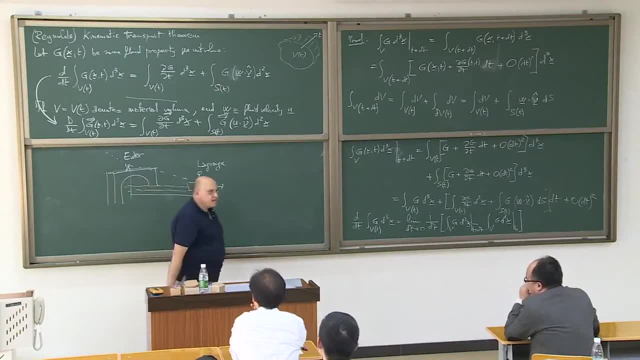 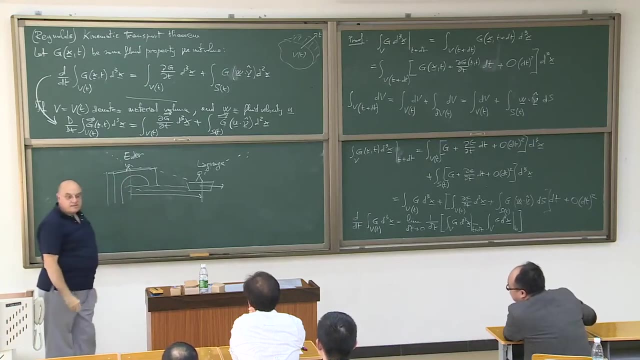 he is on a molecule of the fluid he is floating. so the information that Lagrange with WeChat to somebody else is sending is the reference, the distance from here. so Euler gives information in terms of as time changes and coordinate changes, but Lagrange gives information in terms 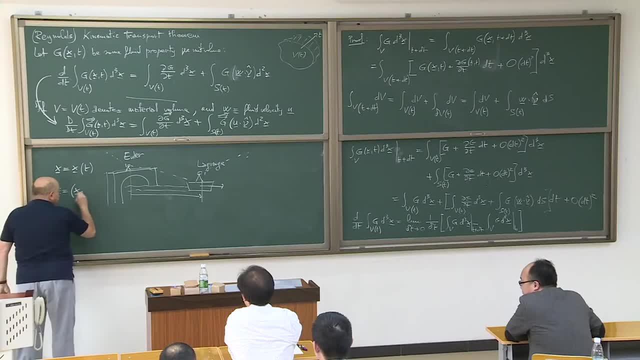 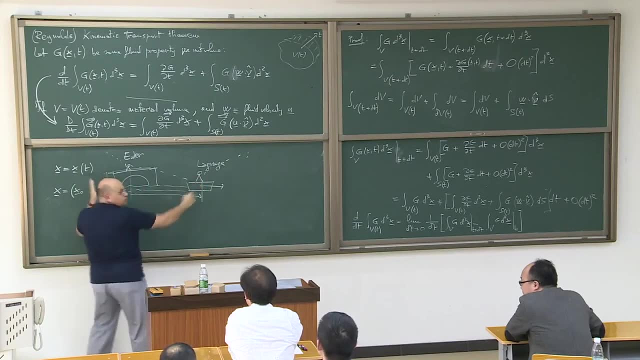 of the initial position. the initial position: it is zero. I was here and now I am moving away from here or from some reference point from where Euler is. so all the information is zero and t x. zero is the initial point and from that point, initial time: t: zero. 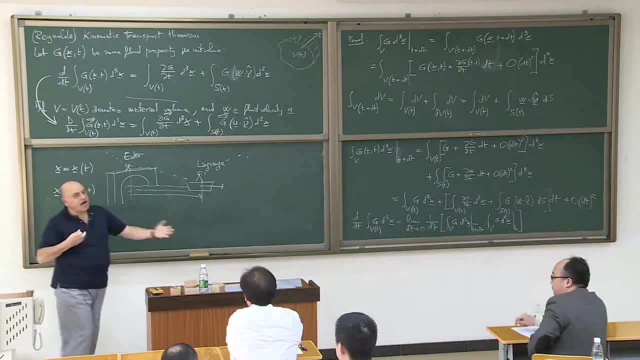 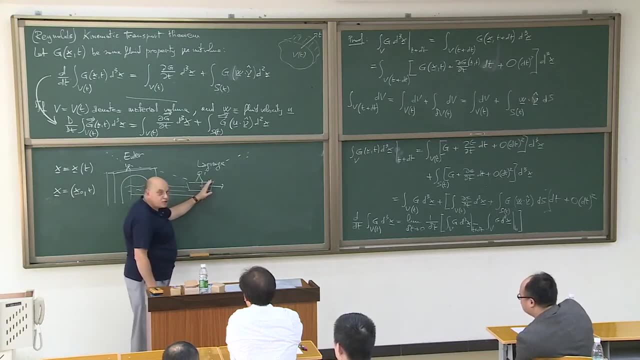 the initial position and from that initial position he sends the information as. so you have to know, you have to know how the motion is with respect to some initial position on a molecule. that is very bad for computational reasons, for computational reasons is very bad. that's why Lagrange. 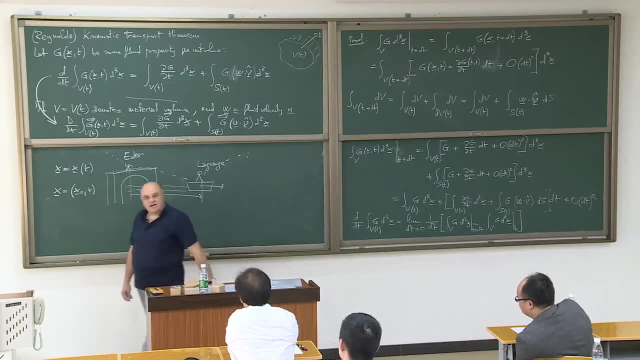 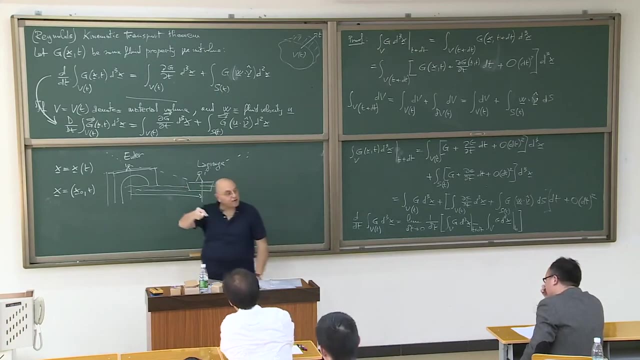 mechanics developed up to a point and then was dropped, especially in this last century, because you want some reference fixed and the motion taking place in your numerical box. but if you want to follow, if you want to follow the powder of coffee, you are on the coffee powder. 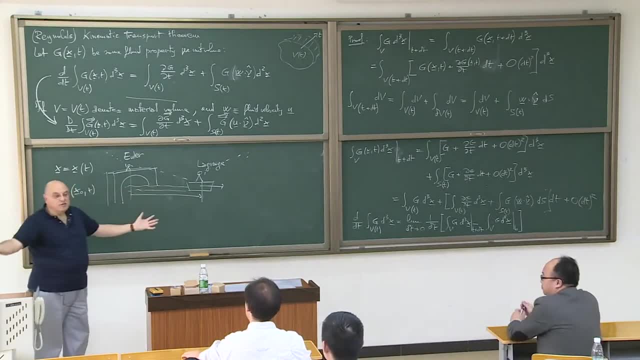 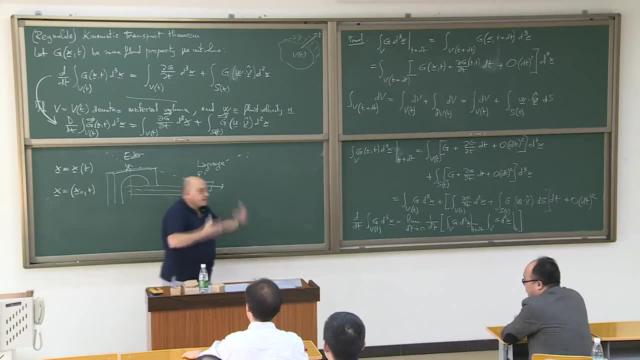 and you see all the world around you moving. that is very, very hard. that is very hard to report back the information. it's not very hard in principle. you are there, you are moving, we are on this planet and we see all the universe around us that somehow is moving. 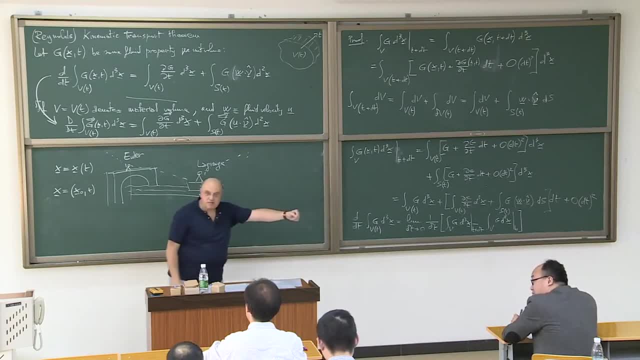 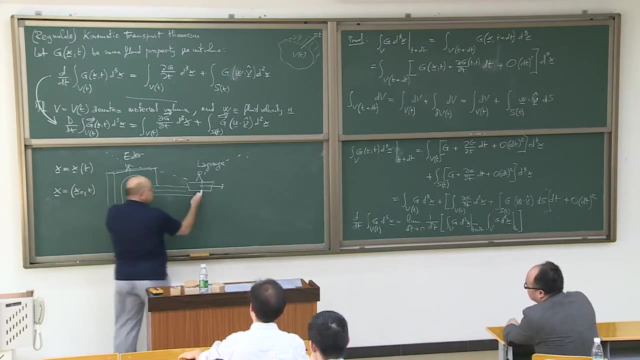 so to speak. but if you want to report back with respect to some reference frame- fixed reference frame is hard because you have to know this and you have to construct the map. you have to know the map at each time. you have to measure this one because you measure the position. 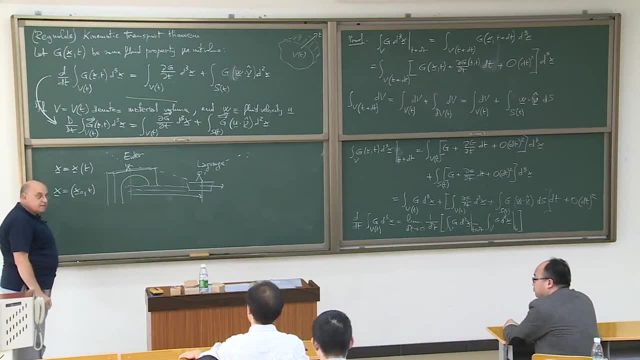 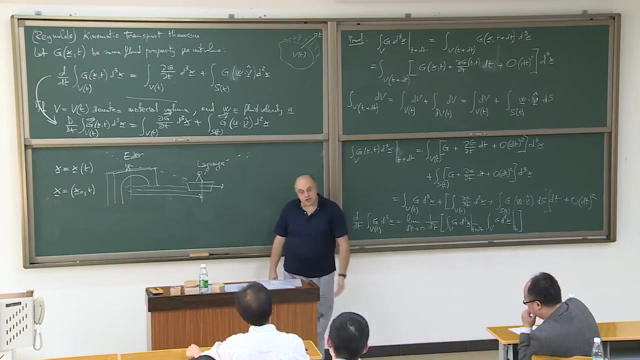 at each time, but here you have to have an inverse map all the time. so this is the Lagrangian viewpoint, this is the Eulerian viewpoint and then is reflected: when you integrate the equation, you may have velocity. you want to integrate velocity in order to have position. 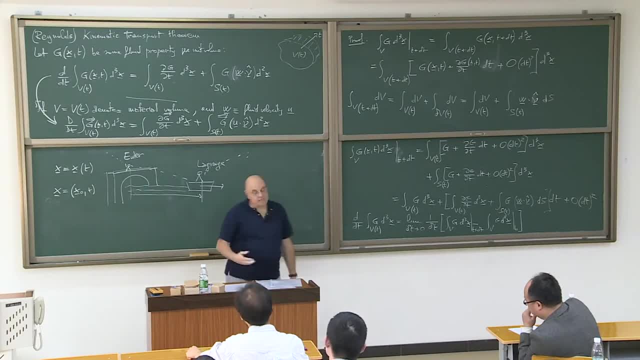 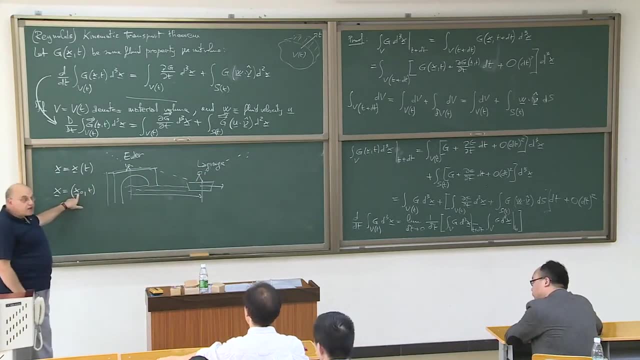 when you integrate velocity, then you have to take care of these two approaches. one is just integrating, you get immediately the position, and the other one is not enough because you have to know the function that depends on x0, x depends on x0, so this is more complicated. 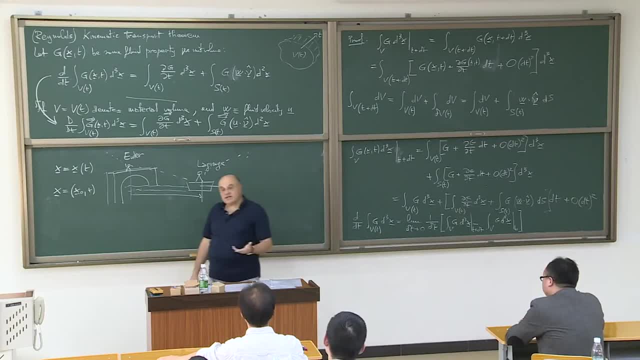 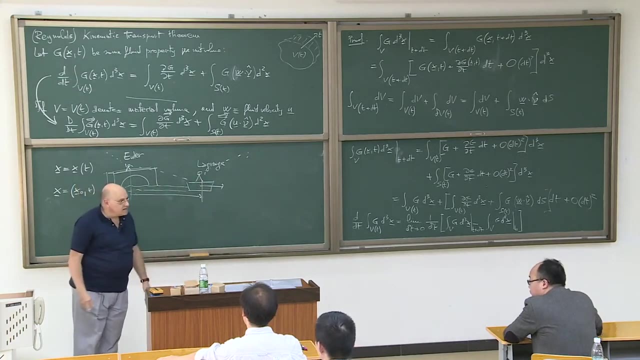 so this is the view we often, in many aspects I will present you: we use a Lagrangian viewpoint. we use a Lagrangian viewpoint. I told you it's not fashionable because computationally is very hard. why we use a Lagrangian viewpoint? ah, it's simple. 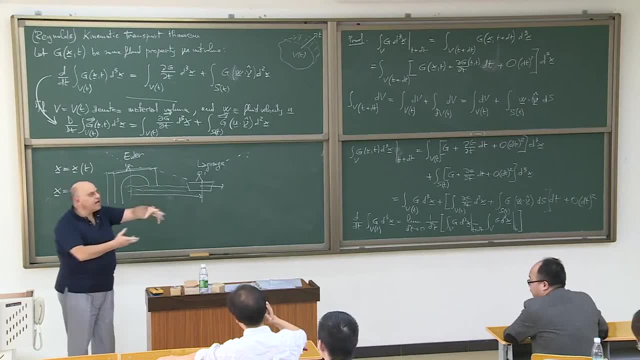 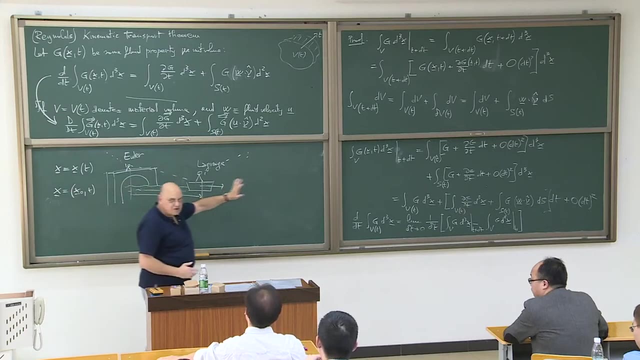 because I want to stay close to the structure. say, a vortex, I want to be on the vortex. I don't care if the vortex hits the river, hits a building. meteorologists care about that. meteorologists want to know if the vortex hits a building, so they have to have a reference frame fixed. 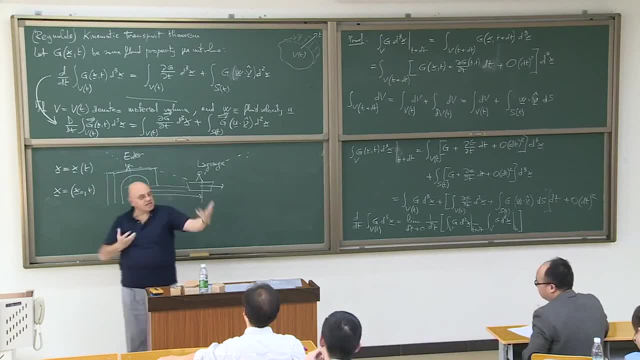 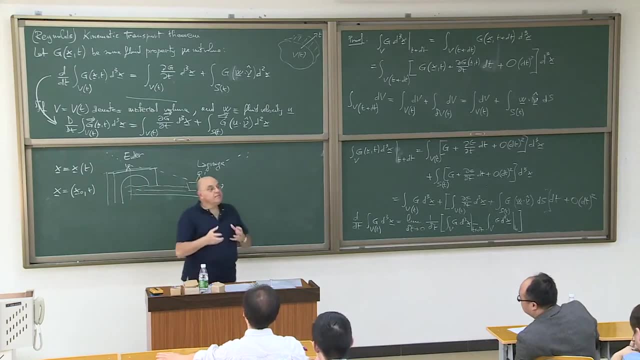 but I want to stay on the vortex. I want to see how the vortex evolves, changes its shape. ok, so I will be moving Lagrangianly and all I'm going to say will be: on these structures. suppose we take a magnetic knot. I want to see how the knot 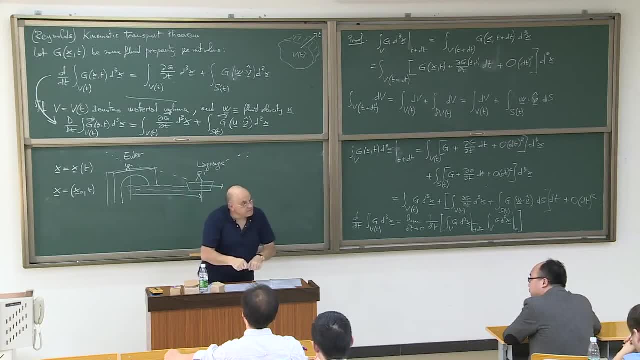 changes. shape is staying on the knot and not outside the knot, not with a fixed reference. so this was very popular at a certain point with a number of people. some, for example, Cauchy was keen on Lagrangian coordinates and Lagrange was not keen on Lagrangian coordinates. 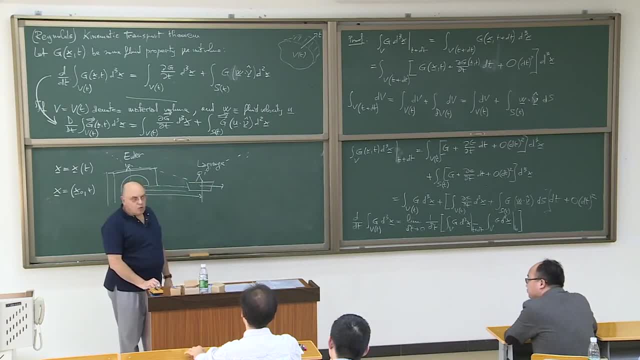 both are due to Euler. so it depends: when you use, say, the Cauchy approach, you find quantities that you may see invariantly, invariant properties, because you move. I move on this planet Earth and I recognize this planet Earth as my home. I know the structure of this planet Earth. 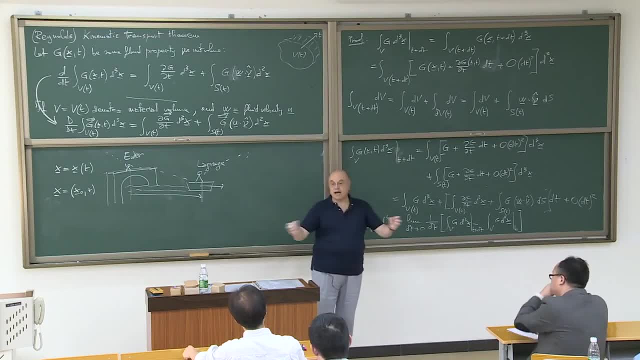 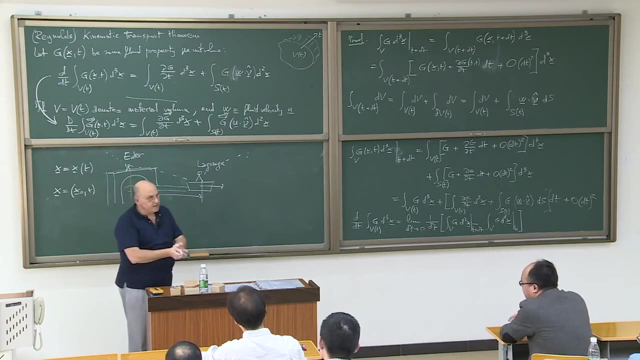 I know everything of this planet Earth. I can see if it is changing or not, if it is breaking up or not. but if I'm away and I'm studying a planet, I have to report back this information all the time. so invariant properties I have to study Lagrangianly. 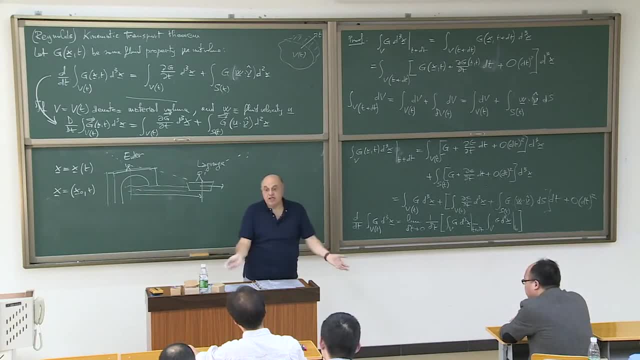 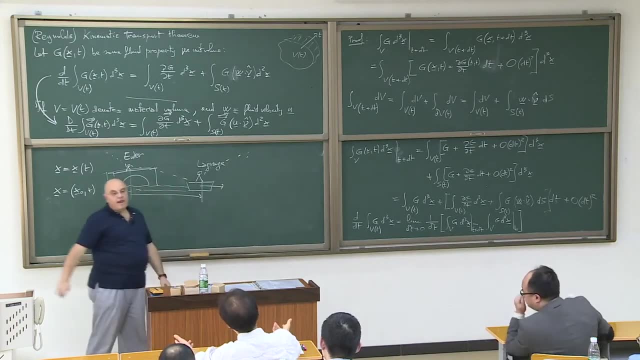 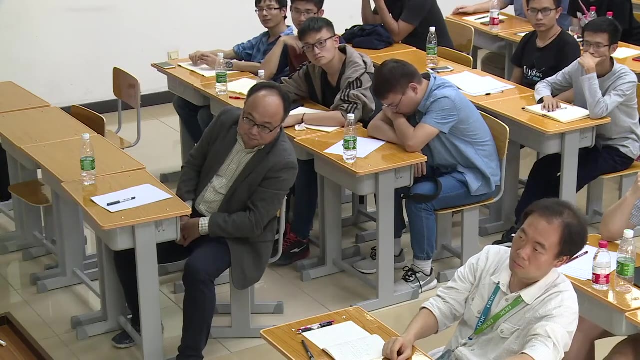 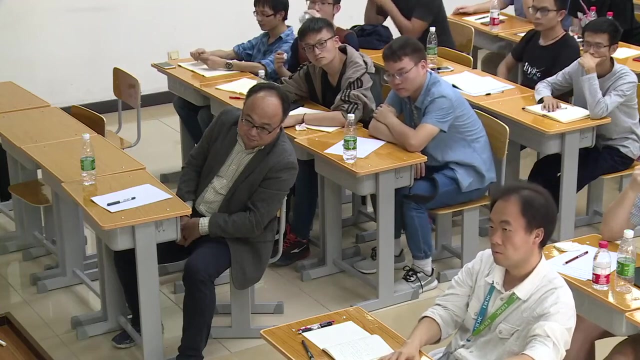 because I can see staying on the structure if it changes some topology, for instance. so is the Lagrangian frame an inertial frame or not? um is not. yes, Euler's, Euler is definitely. you have to have this flow map, the inverse of this flow map, all the time. 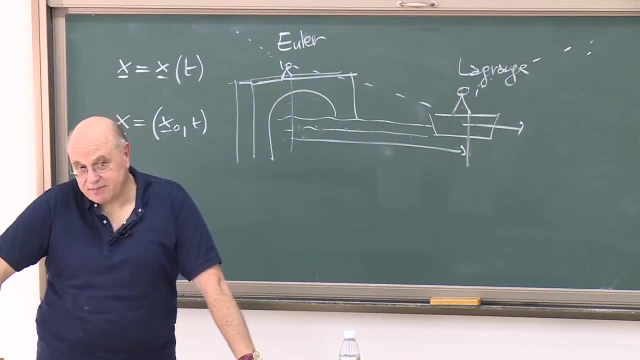 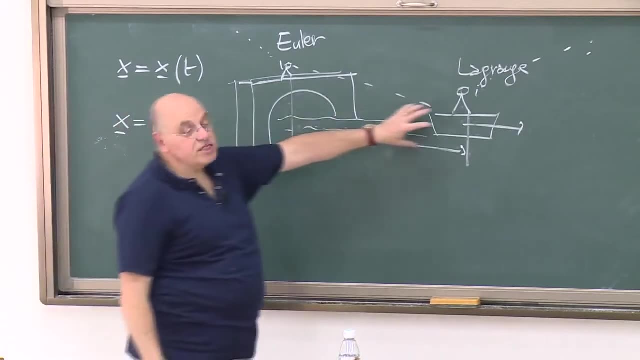 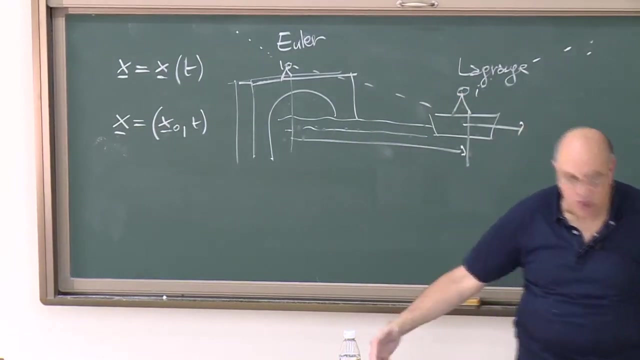 that makes problems in reconstructing the position, because what you're thinking now is Eulerianly. you think as an Euler. you want to know this boat where is going. but I don't care where I'm going, I'm caring if the boat breaks up or not. 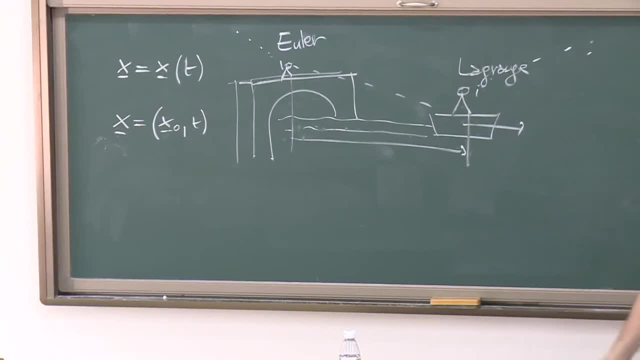 I want to stay on the boat and I can reconstruct the motion close to the boat, with respect to the river. I was, with respect to the shore, to the bridge, to some reference, but sometimes I don't care. you see, I don't, I may not care, I may not care. 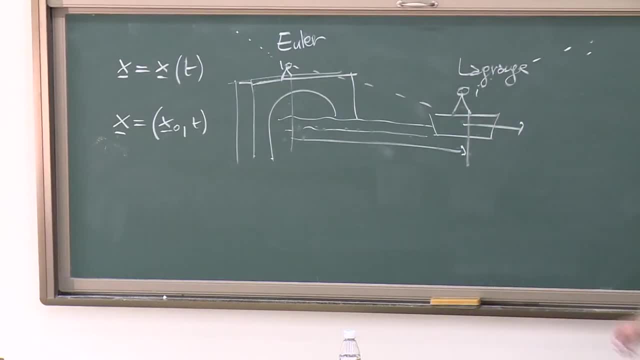 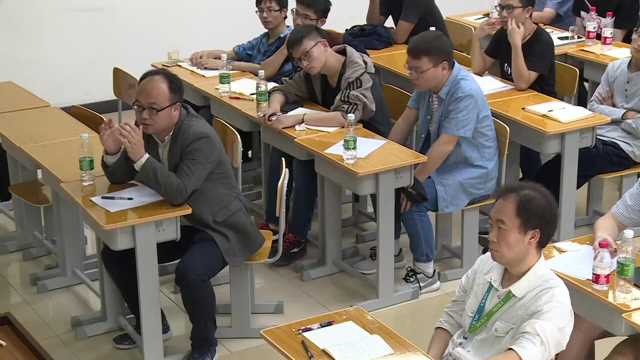 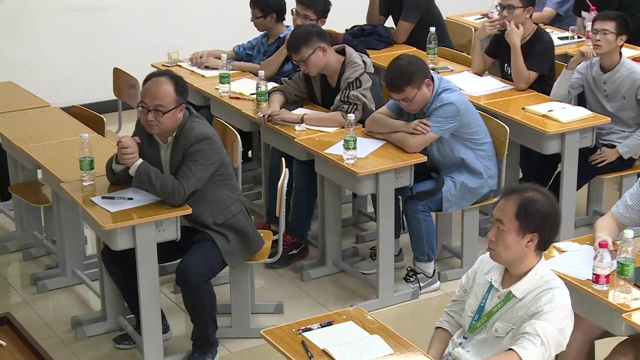 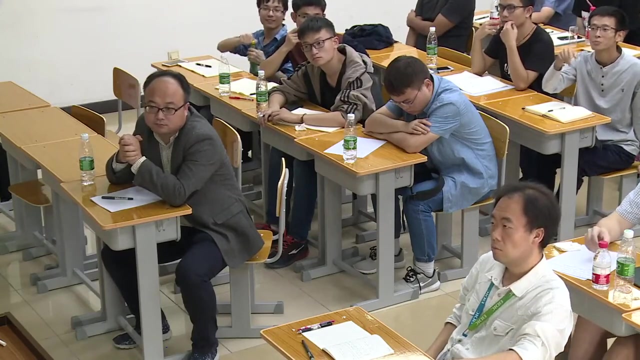 if you are away in the sea, you may want to take care of your boat. if the boat is working, fine. no, at the moment it's still kinematics. you're right, we get to dynamics in a moment. can you say the viewpoint of Black Round is more natural? 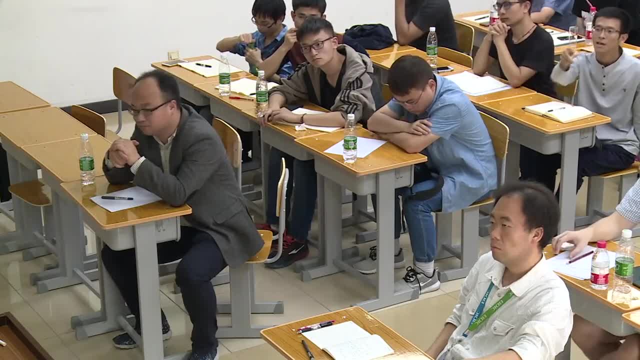 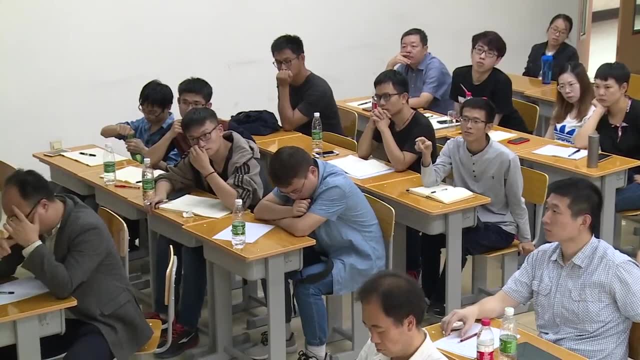 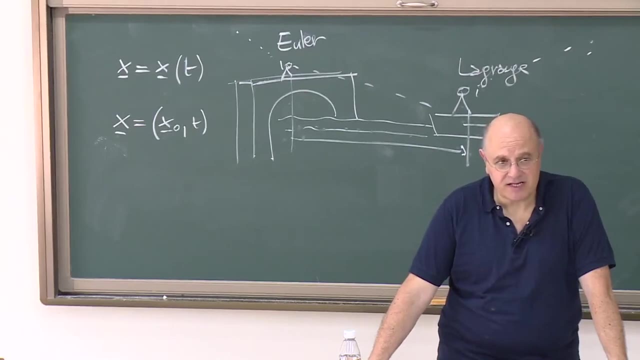 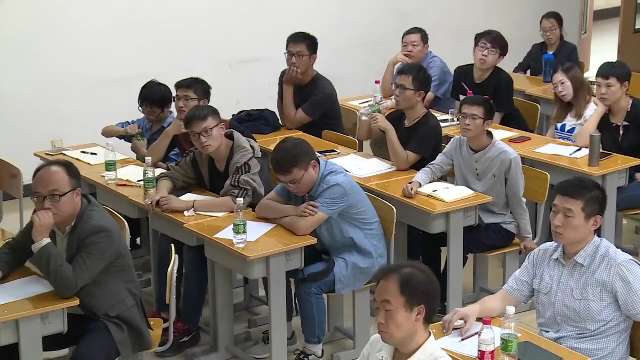 it is consistent with the theory of roundness and Euler's point is consistent with cat, cat, cat. ah, I don't. I'm not so sure about that because it depends on the problems. certainly, if you- I rephrase it my way- if I'm considering invariant properties. 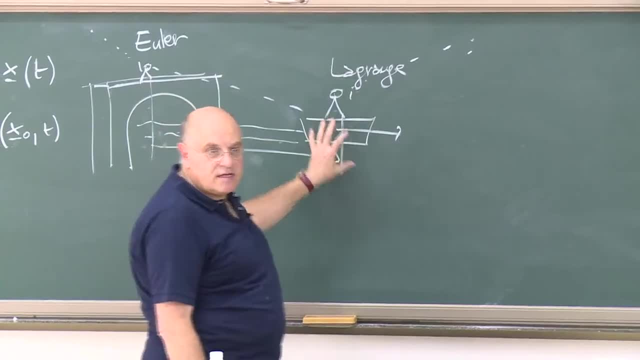 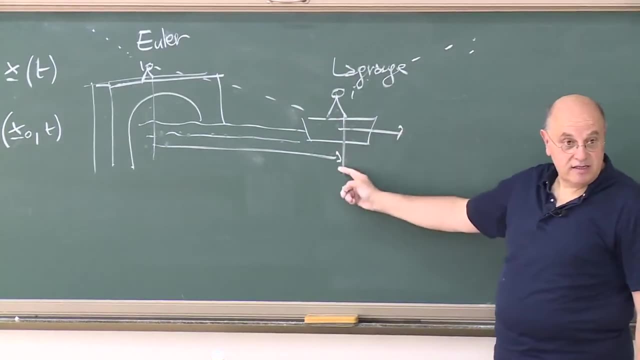 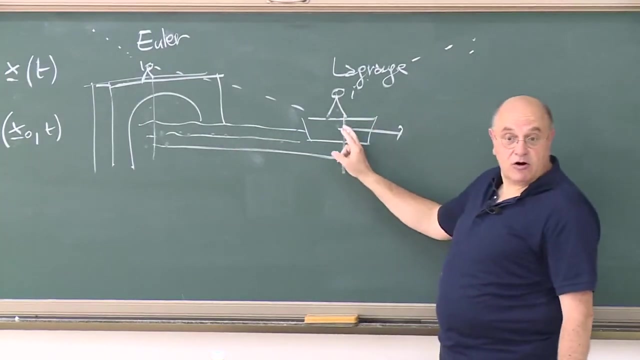 of an object, say the boat, then I am Lagrange, because measuring changes here, measuring changes here can tell me if these changes are occurring or not. but if somebody wants to know here what the changes are occurring here, you see what I have to do: I'm moving. 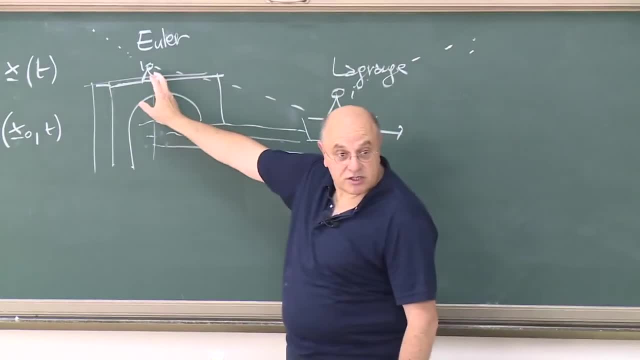 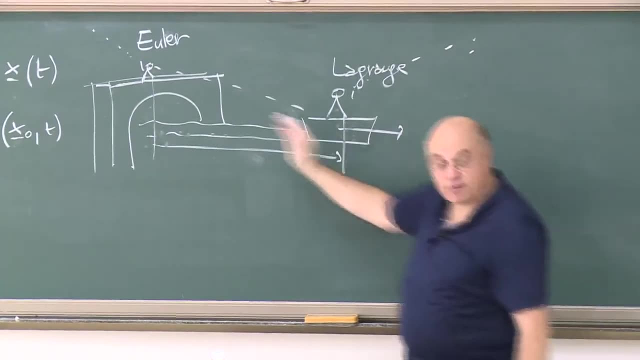 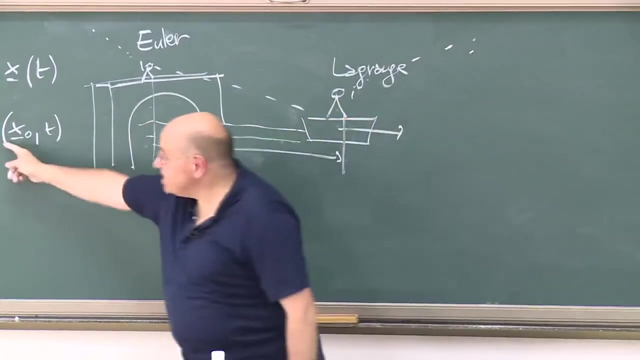 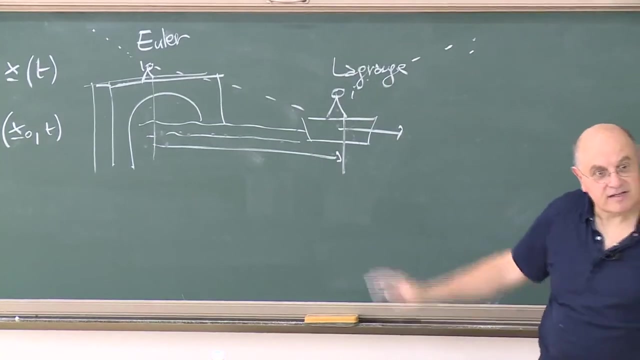 all the changes I have. I have to tell this changing to this person. in terms of the distance from the bridge, I have to add some more information because I'm caring about the bridge now, so I need this flow map. inverse, you know, is taking water. this is a change. 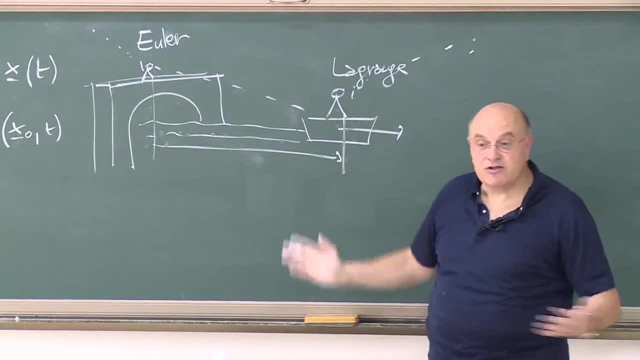 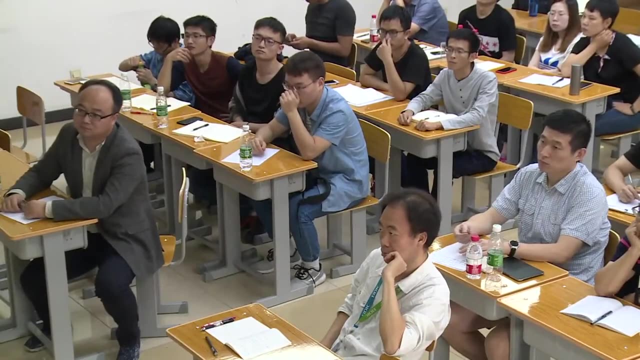 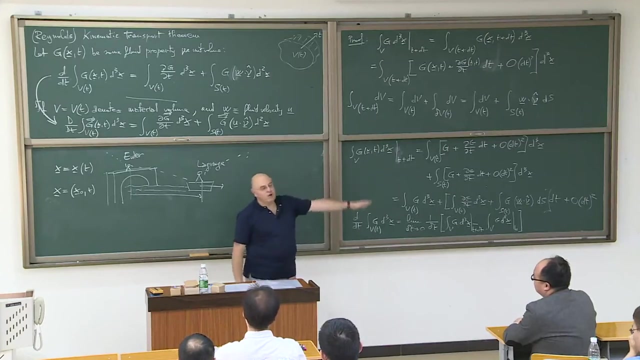 and with respect to the distance. but if I care about the water, if the boat is taking water or not, I don't care about the distance at all. I just care about if it takes water or not. if it doesn't take water, I'm happy and suppose I don't want to go anywhere. 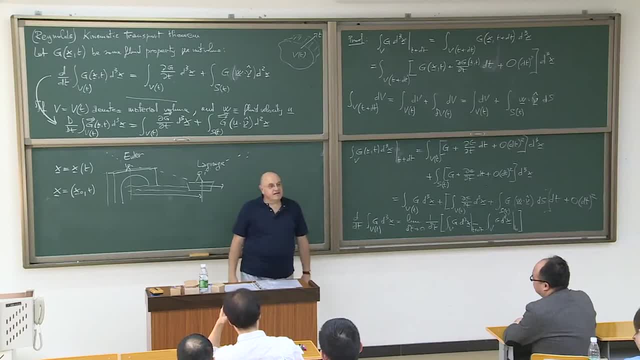 I just want to float, suppose. then it's ok, the boat is fine, I'm not taking water. I'm not quite sure where I'm going, but it's fine. but if it's taking water, I need help, I need to communicate my position and I need to communicate. 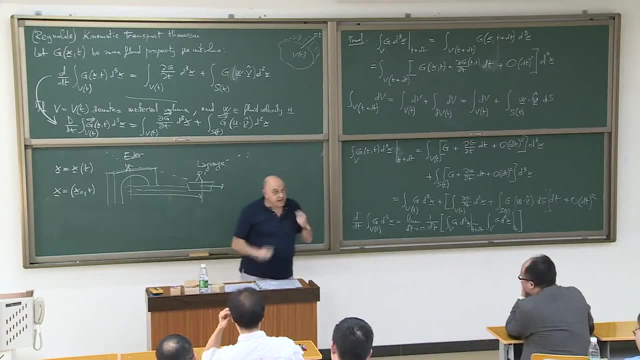 how much water I'm taking in and the people that listen, they have to compute two things: the water I'm taking and if I'm going away, where I'm going to be, where I'm going to take, because I need two information. so, of course, if you are helping somebody, 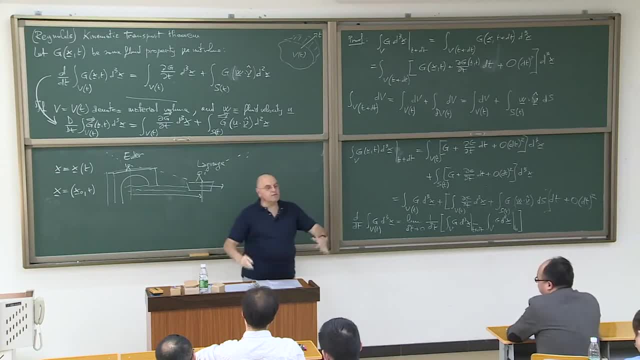 it's easier to have Eulerian viewpoint. the Eulerian viewpoint means you are mapping from a fixed reference frame. whatever happens from here, I just need to know if there is water or not. so suppose this is the example. suppose the water is empty and it's floating well. 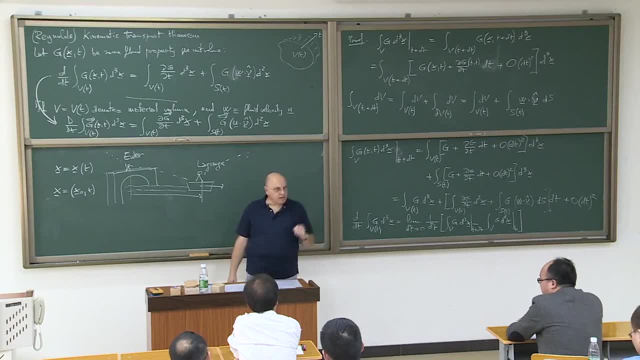 this is the invariant property I want if I'm taking water. this is no longer conserved quantity, and so this is not invariant with respect to motion. of course it's not invariant also in Euler terms, but in Euler terms, to have the same amount of information, I need just more information. 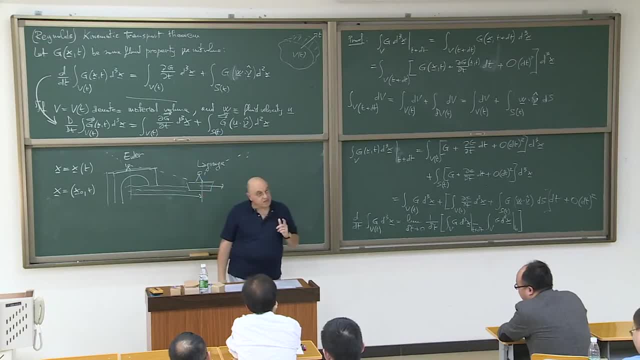 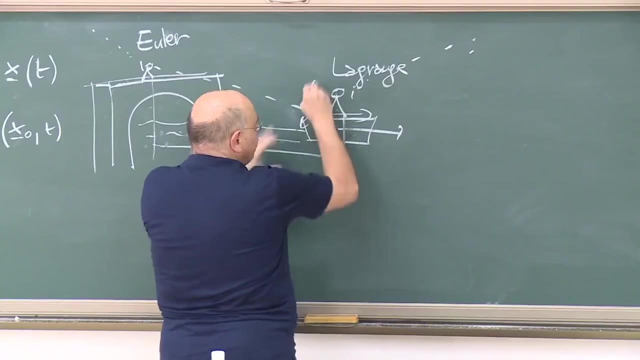 because I have to report back all the time. you see the difference. it's advantageous to stay here and to see what happens, because computationally, if you are Lagrange, you have to calculate. you have to have a reference system here that calculates your invariant properties and then you have to report back. 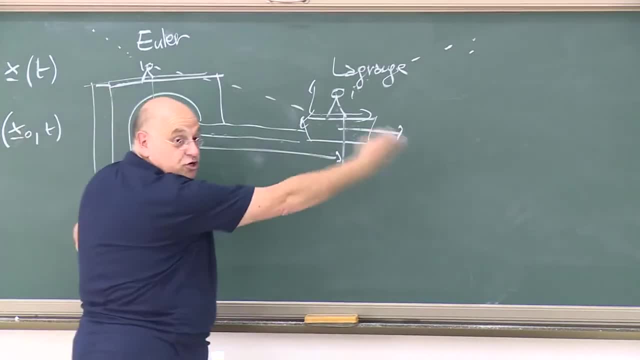 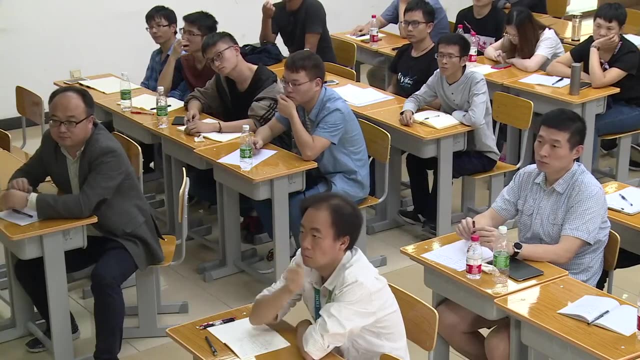 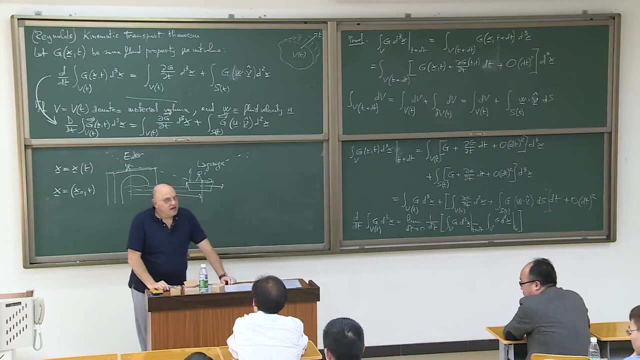 but to report back you have to know the evolution of the fluid. there is a similar problem I my first. one of the first problems I considered when I was your age is exactly of this type of problem. at the time there was a beginning of string theory and my first paper was actually. 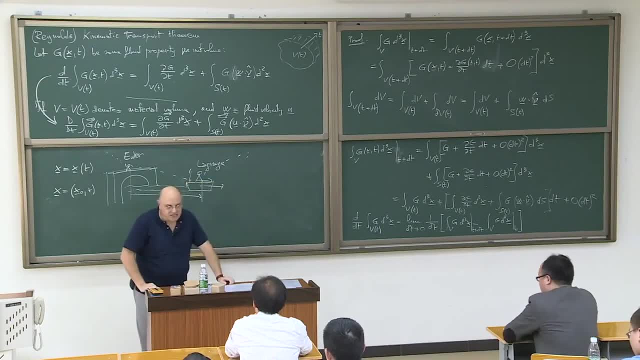 in this context. it was the emerging string theory of the time, in the 80s, late 80s, and the string was a vortex, a la Taubes, and these vortices could be studied either with a reference frame on the vortex or from outside, and so 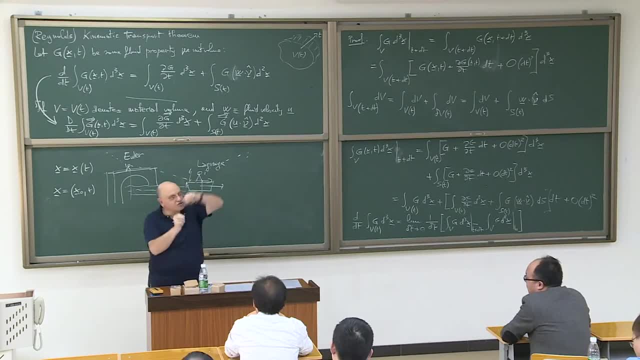 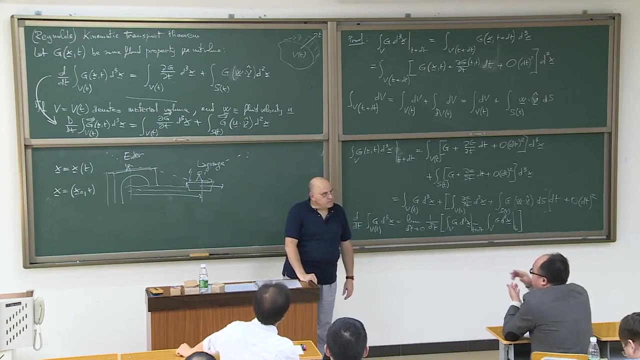 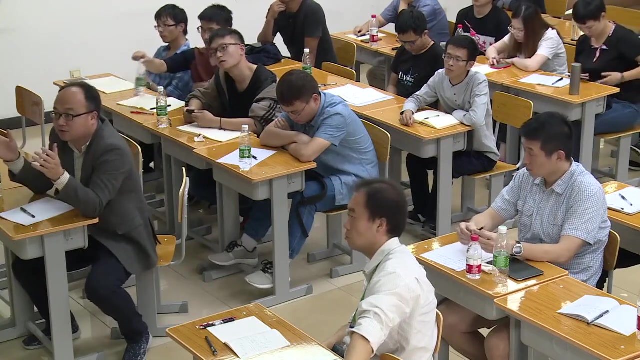 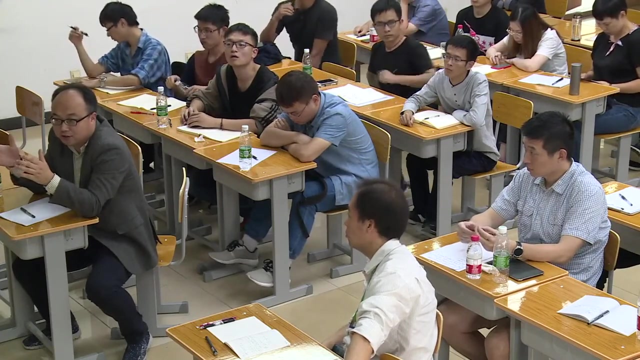 I started to consider the Lagrangian viewpoint. to stay on this string. on this string you see the motion and perturbation of the string, but then you have to report back sometimes, or both, yeah, you can choose both dynamically. it's not the same, it's a. 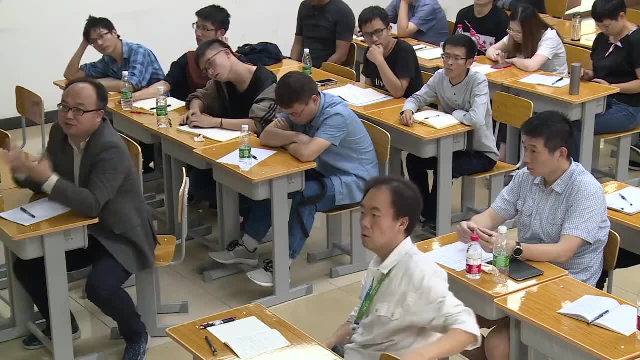 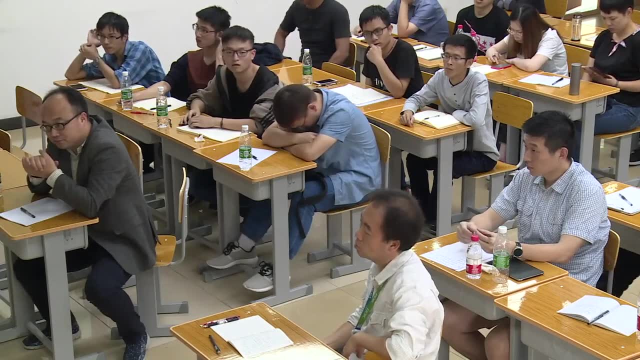 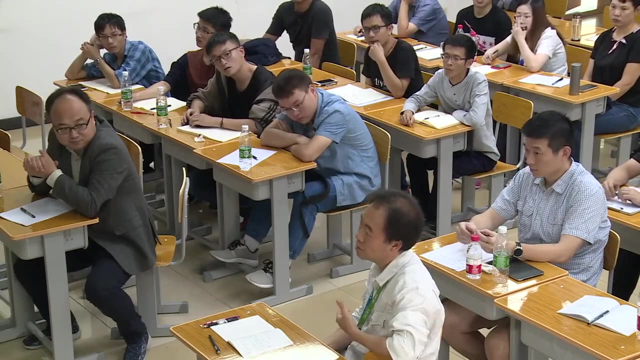 composition of functions. oh, of course. oh, sure, sure, sure, sure, it's the same. you can transform one system into the other, so in principle it's not a problem. so the Lagrangian one should have an extra term. the Lagrangian should have information about the initial position. 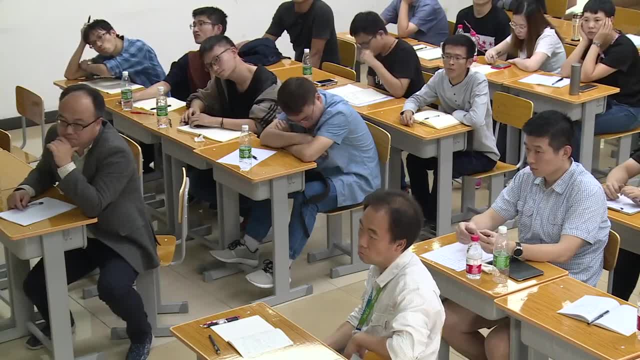 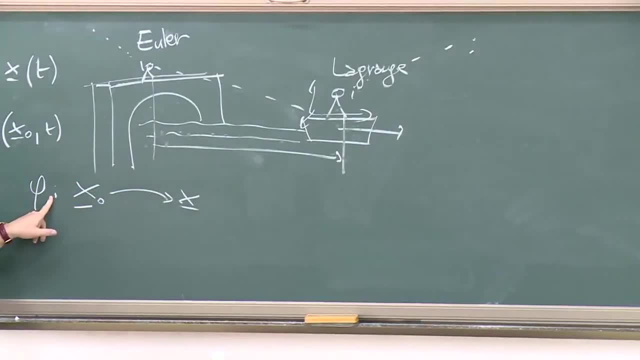 all the time. it's the very first mapping. I gave you this one x0 to x, and I have to know this map and I asked for the existence of the inverse at all times, that assumption that one is not an inertial system. so you should have an extra term. 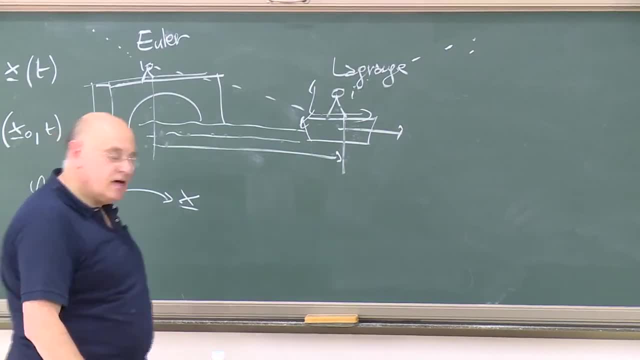 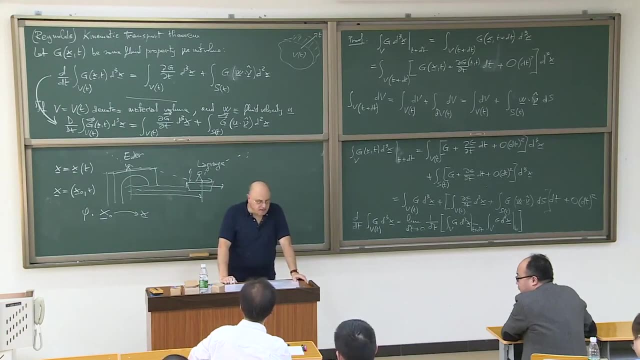 oh, you have acceleration, you have extra terms. it reminds me you know better than me, because it's not my field, what is called Thomas precession. Thomas precession is when, instead of the electron, you are. the system of reference is yeah, yes, is Matteo, now is. 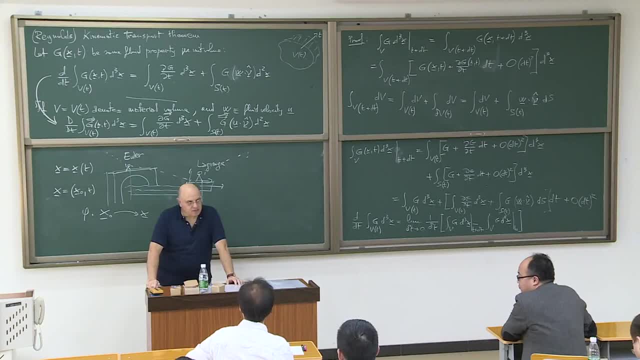 taking care of that problem. yeah, so this, this problem, will accompany us, and I will have time to make more comments, because, of course, a vortex will induce a motion, a fluid motion, and it depends where you are, if you are on the vortex or if you are on the fluid. 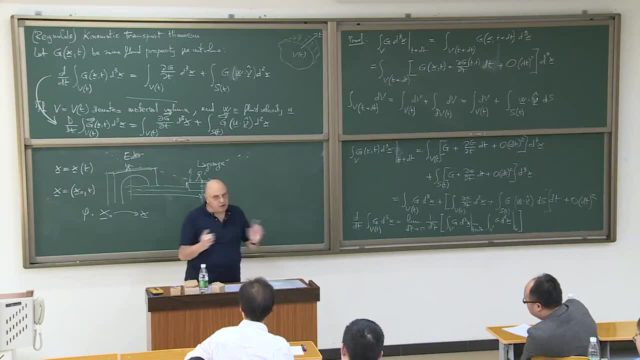 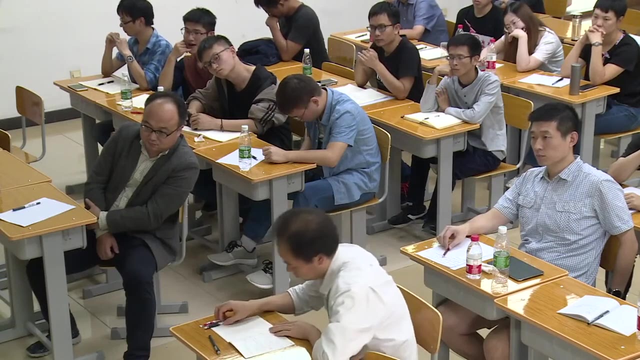 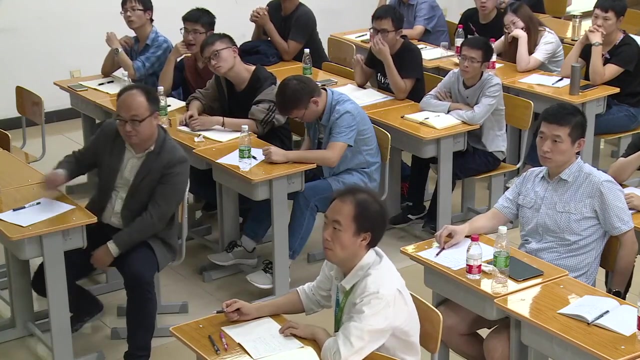 the physical phenomenon is the same, but the way you perceive dynamics is different. the way you perceive it, yeah, yeah, ok, so I want just to. so this is a little story about Euler. so, remember, Lagrange is on a molecule and is moving, and Euler is fixed and we are looking at the world. 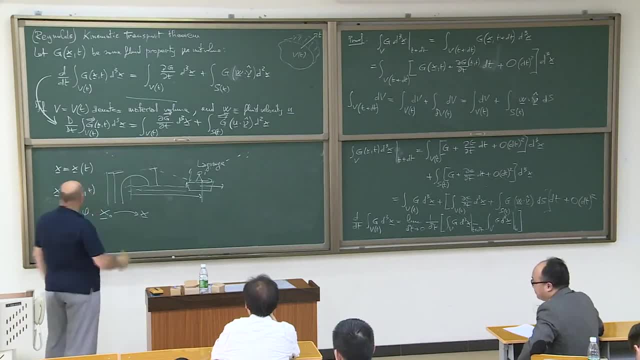 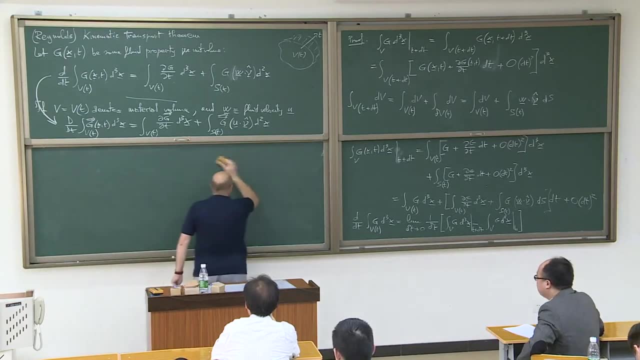 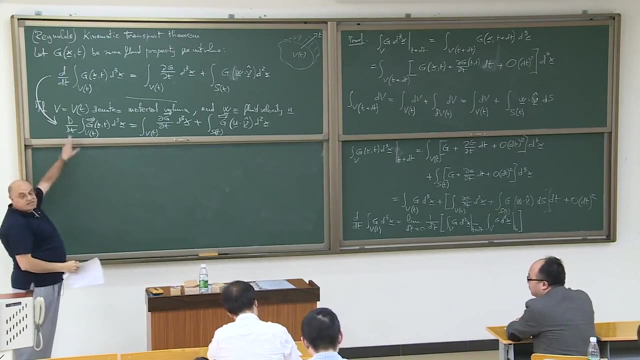 that is changing. ok, this is just helps you maybe to remember these two. and this is the so called Lagrange derivative, because it combines together the time variation and the space variation. we will come back to this because it's important when you say that something is constant. 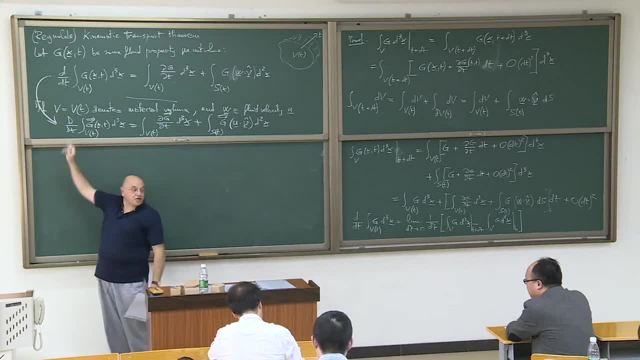 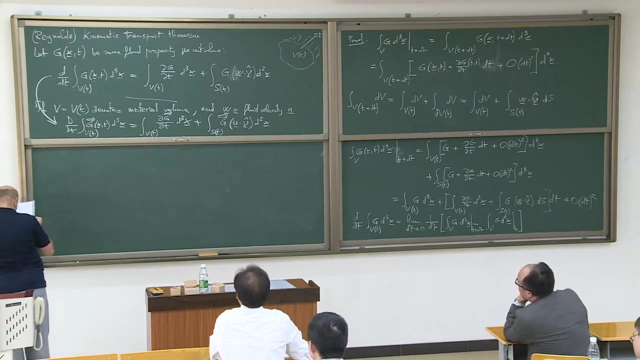 is constant with respect to this variation, it doesn't mean that has constant value. it means that the sum of the variation in time and space balance out. ok, alright. so of course we have the quantity. from this, we can say a corollary. the corollary is: 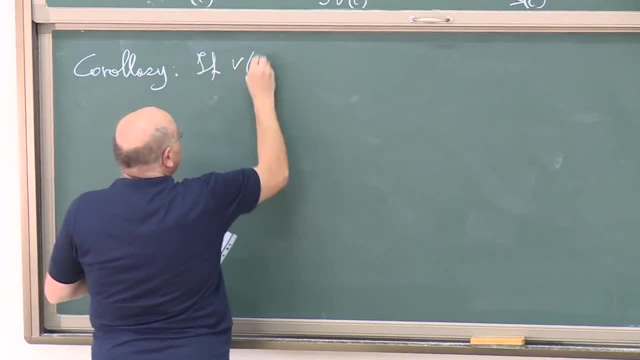 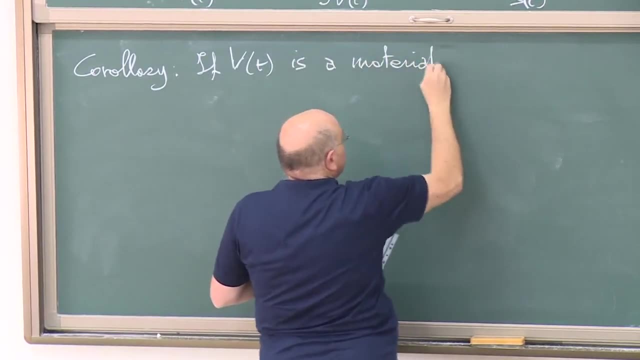 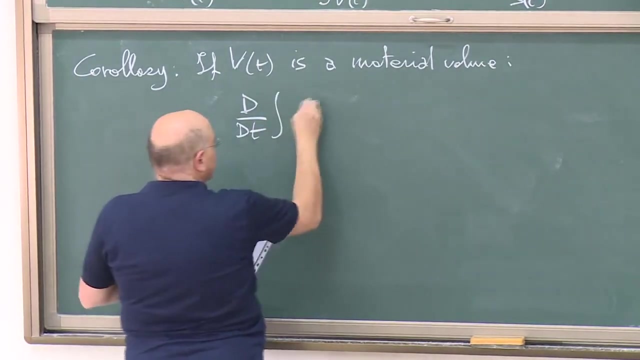 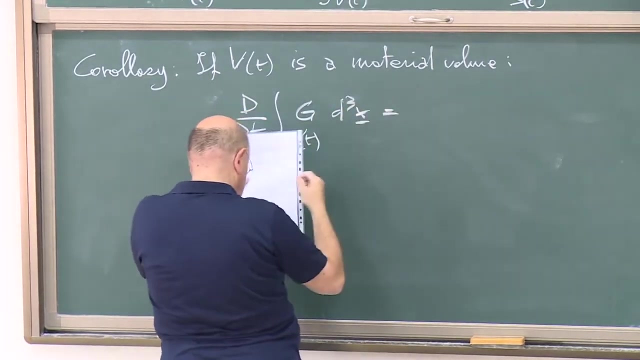 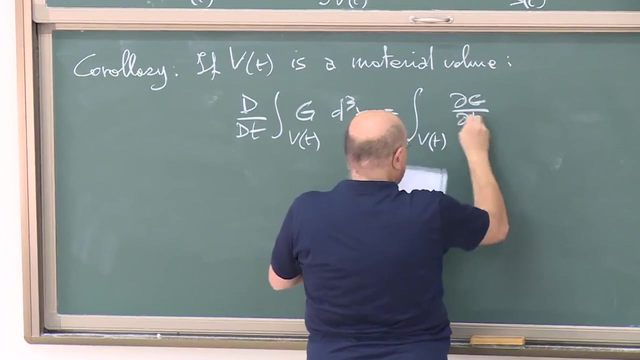 that if v of t is a material volume, then derivative with respect to time, of this quantity g. as I said, it can be a scalar or a vector. at the moment it's still a scalar, if you like, is just the integral vt of dg dt plus I applied divergence theorem. 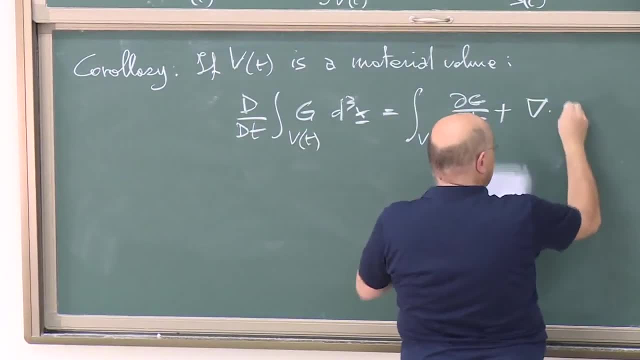 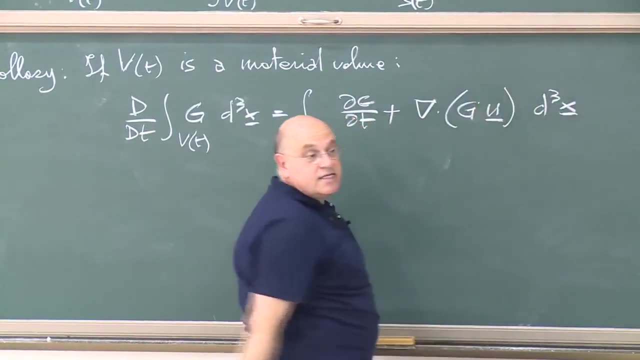 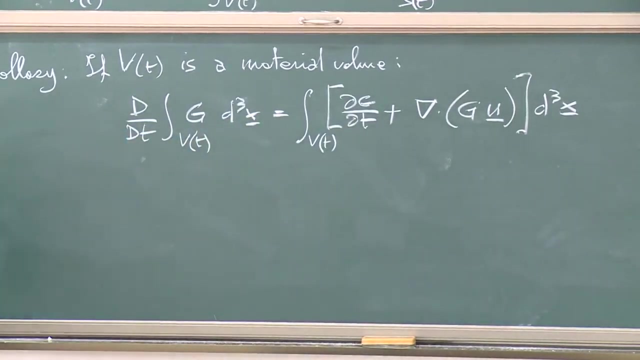 to that one and I have the divergence of gu. in d3x I transform the surface integral into a volume integral, and this is just the basic relation. yeah, one last step. this is just easy on the blackboard to do it. please repeat the exercise of multiplying everything. 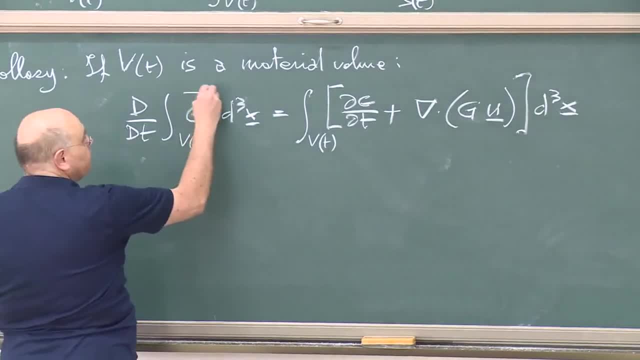 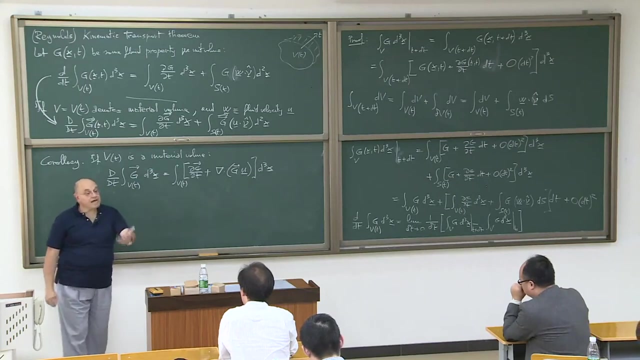 by a fixed vector and then you immediately transform the same equation into an equation that works for a vector. what we'll do? we use this dual aspect. when g is a scalar, we use mass and we apply this, and when g is a velocity itself, we get the conservation of. 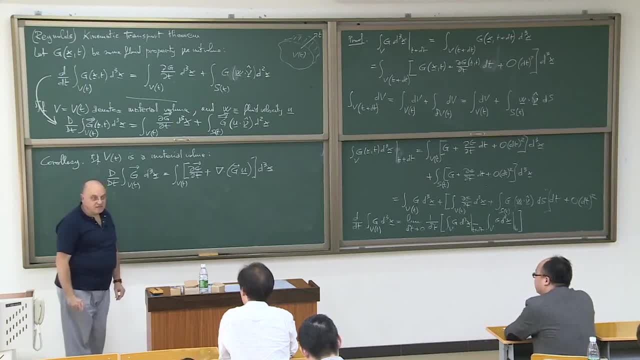 linear momentum. I stop here for the moment. we take a break and then we resume. ok. 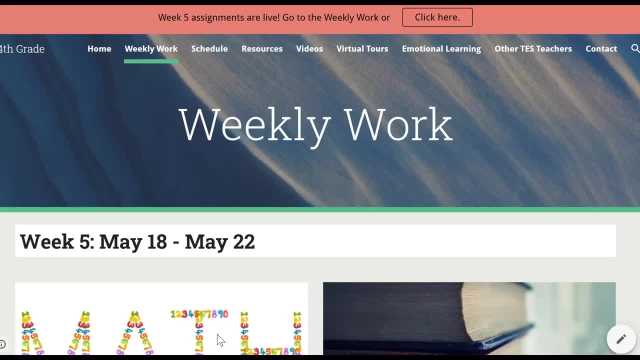 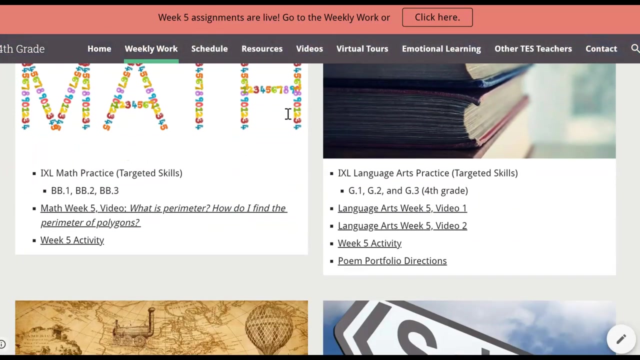 Hey fourth graders, This is our poem portfolio question and answer and tutorial video. So first I'm going to start off by showing you where you can find the directions for the poem portfolio. So I'm here on our fourth grade website, I'm going to click weekly work and then I'll scroll down By the 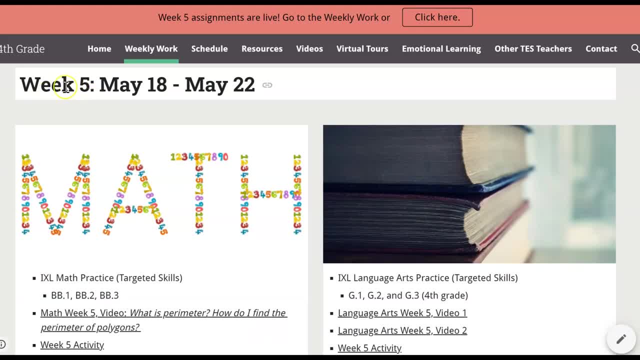 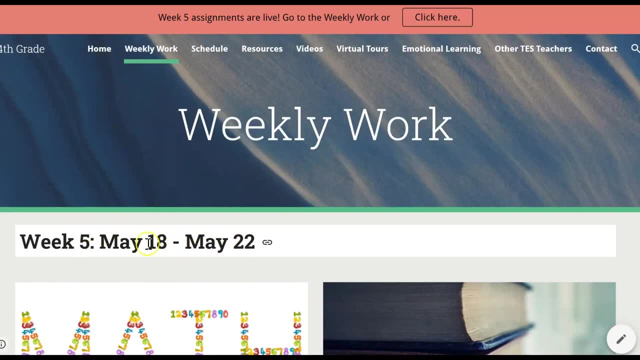 time this is posted it will be week six. It says week five right here, but I will also have the poem portfolio directions under week six. So when you go in on Tuesday or Wednesday and want to work on your poem portfolio but you want to see, 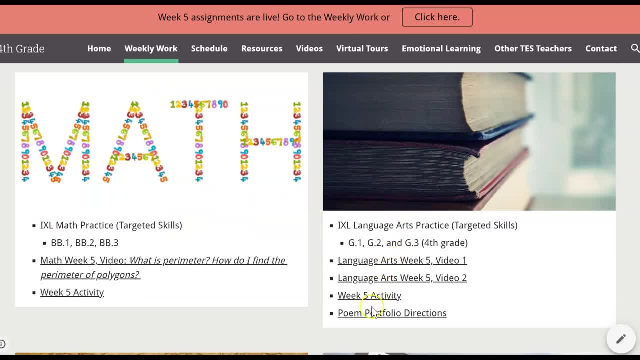 the directions week six will be up and there will be a link that says poem portfolio directions right there in the language arts. During this week six we will have two other videos to cover the last two types of poetry and then plus this video. So 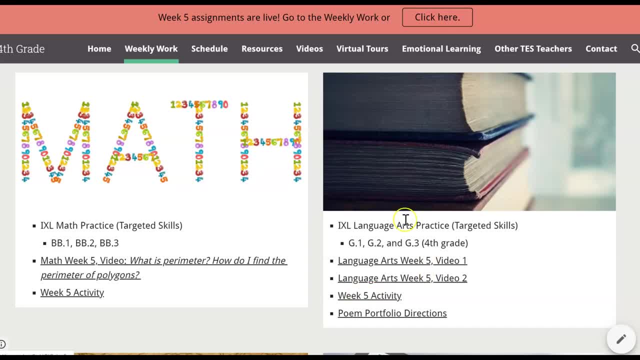 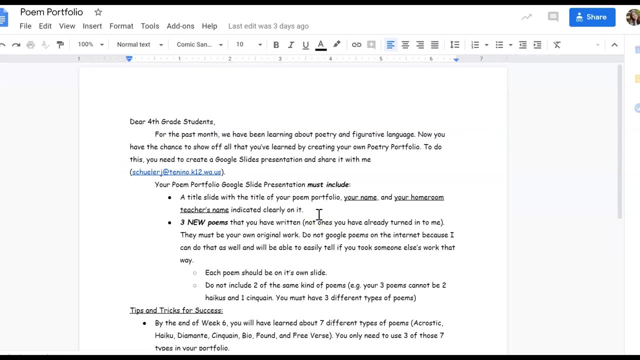 three videos, but there will not be another activity and there will not be IXL practice skills, because I want you to focus your energy on our poem portfolio. So let's take a look at the directions. I clicked on it and it took me to this document. It is shared with you, so a view only version.